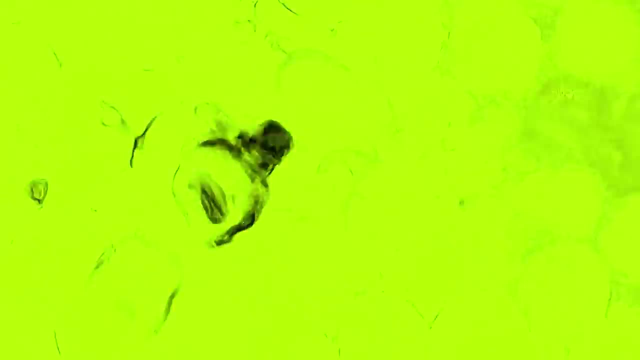 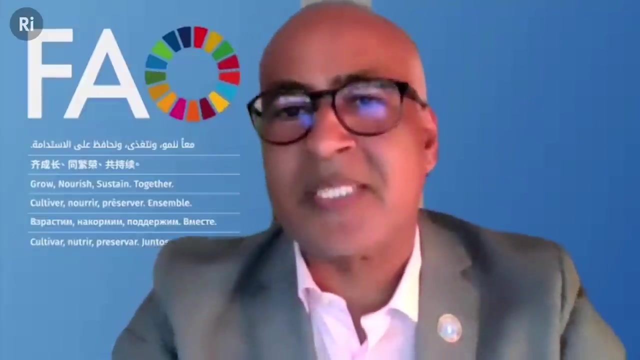 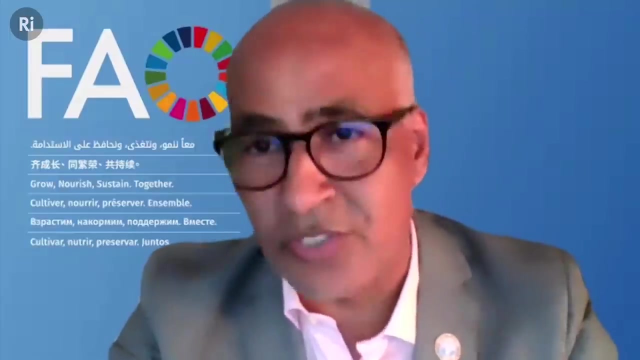 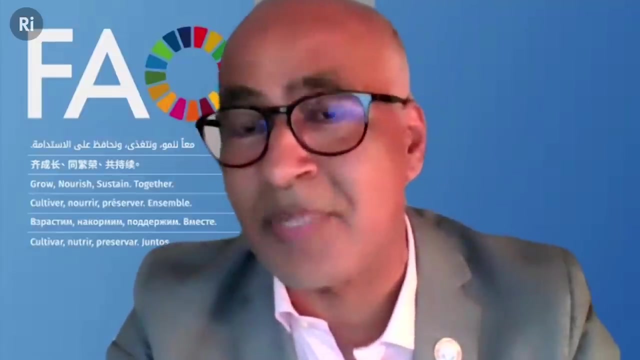 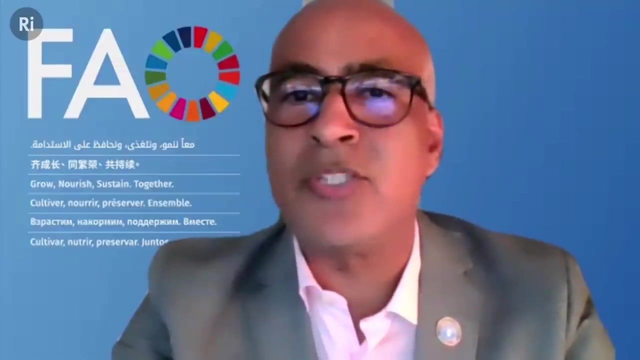 So today we're going to talk about these two main topics: climate change and biodiversity. If we look at what's happening globally, unfortunately we're not on track in tackling climate change or tackling biodiversity loss or achieving the sustainable development goals, So we are still not acting enough in terms of magnitude and in terms of speed as well, really. 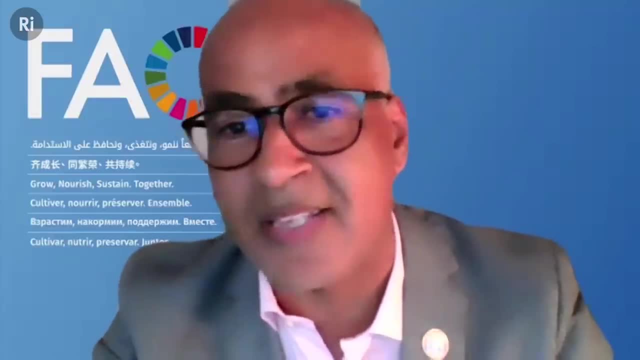 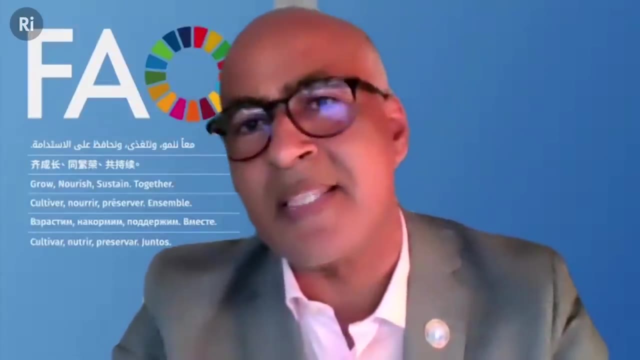 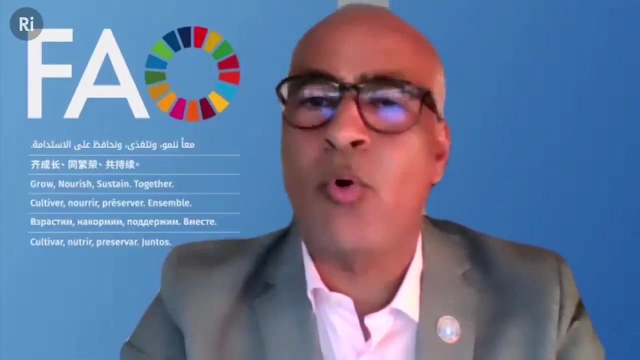 to tackle these challenges, These challenges, they are much faster than us. And if you look at the climate change, the Intergovernmental Panel on Climate Change, the IPCC, in their special report on 1.5 degrees C, they clearly stated that the world has already warmed by 1 degree C due to. 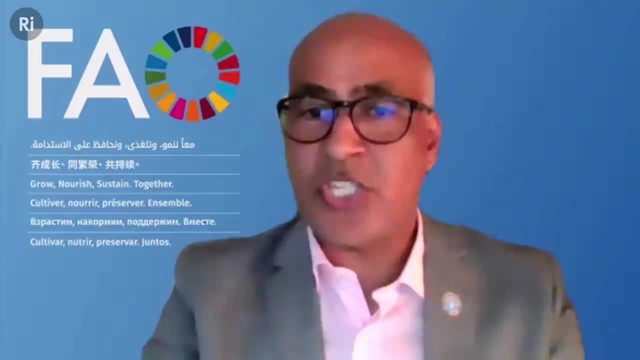 our human health. So we're not on track in tackling climate change. So we're not on track in tackling climate change. So we're not on track in tackling climate change. So we're not on track in tackling human activity And, as a result, climate change is already affecting people, ecosystems and 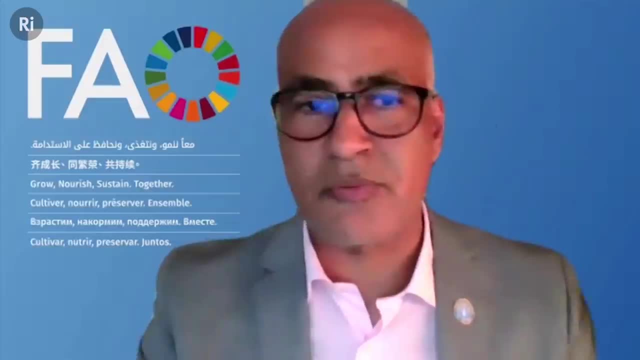 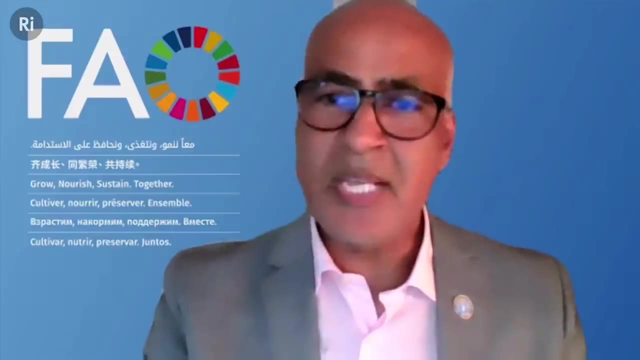 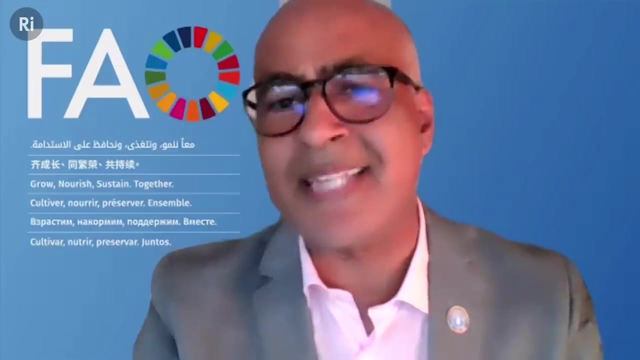 livelihoods across the globe, And the main conclusion from the report was that we have basically now around nine years to fix this climate crisis, And I'm sure you all heard lately about these floods in Germany and how this showed the devastating impact of climate change. 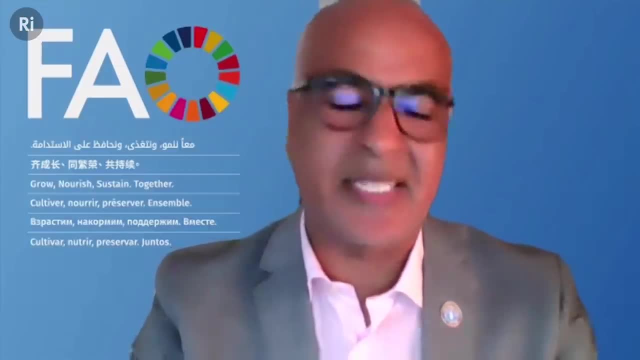 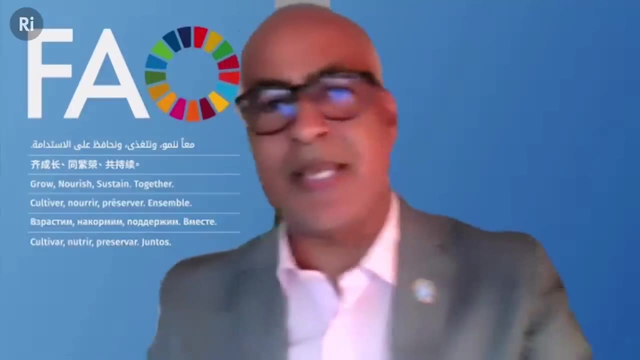 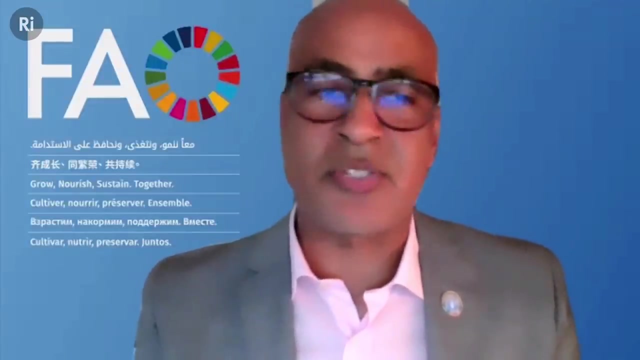 and where this impact can hit anywhere at any time, And if you look at the difference between the one point degrees C, two degree and three, and this highlights the importance of why we need to stay below 1.5 degrees C to avoid the dangers of climate change. If we look at the difference, so at 1.5 degrees C, 4% of the mammals will lose half of their habitat And at 2 degrees C that will double. That means 8% of the mammals will lose half of their habitat. 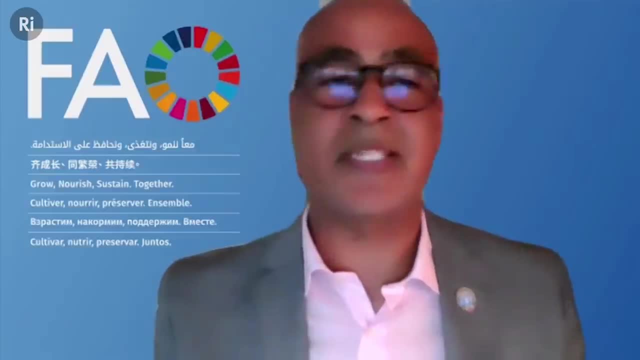 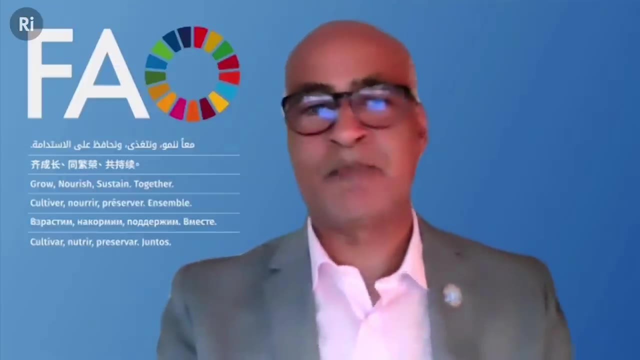 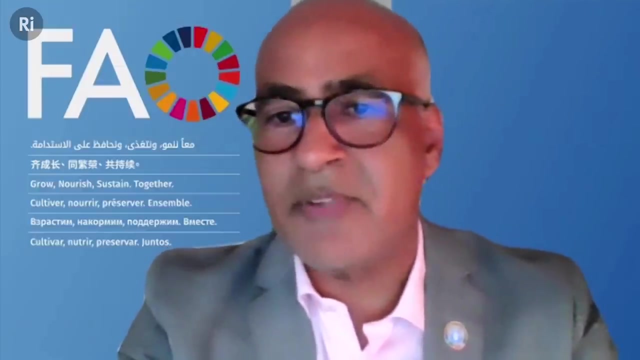 And at 3%, at 3 degrees C, rather, we're talking about 41% of the mammals losing half of their habitat. And if we look at the IPBES report, the Intergovernmental Science Policy Platform on Biodiversity and Ecosystem Services, 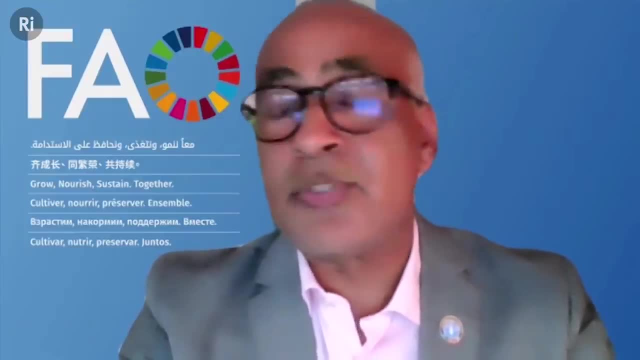 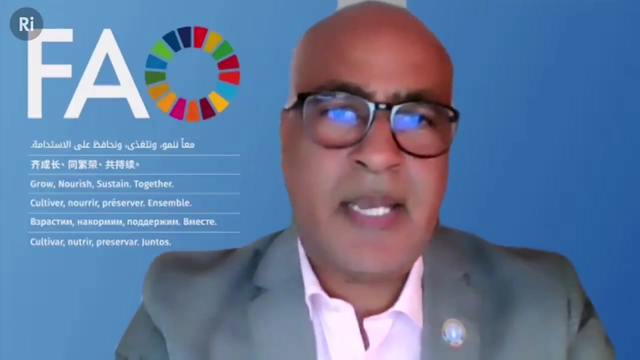 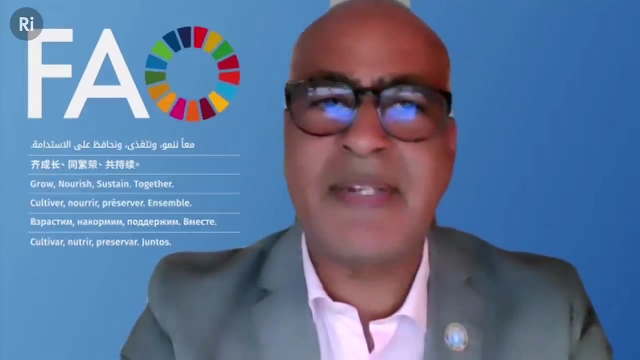 in their global assessment report, they also show that, unfortunately now we have around one million species of plants and animals that face extinction within a few decades. In terms of deforestation, unfortunately now we're witnessing around 4.7 million hectare of forest. 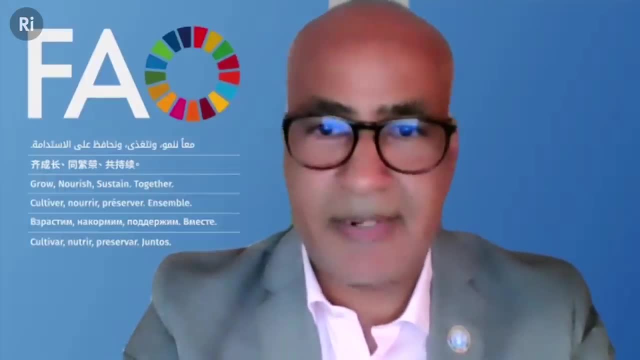 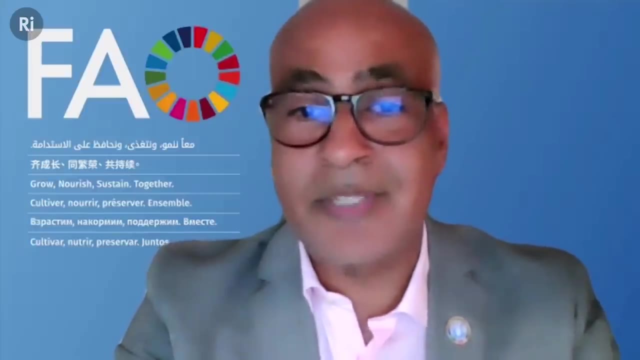 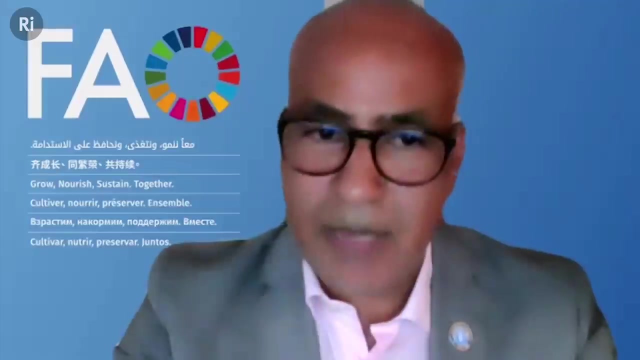 an area larger than Denmark, that are lost every year. So at FAO, we're trying to well. our goal really is to defeat hunger, basically, and to achieve the sustainable development goal: to achieve zero hunger and also to tackle climate change and biodiversity loss. 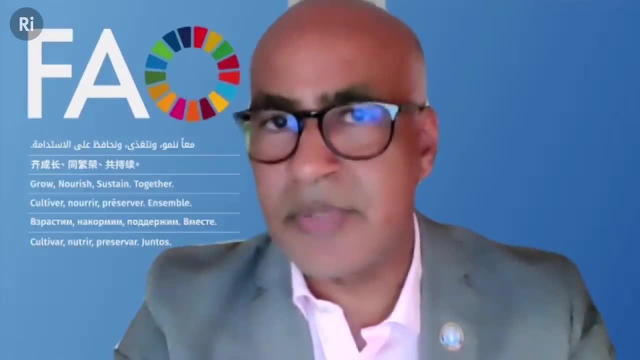 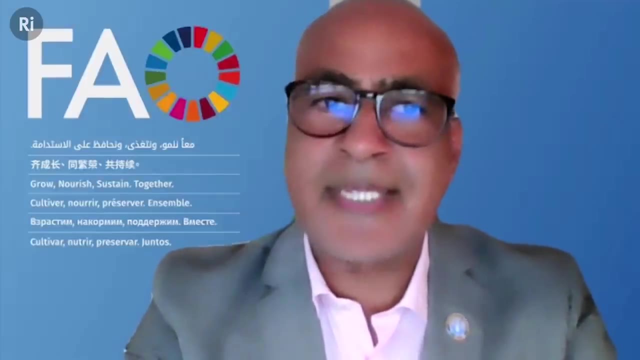 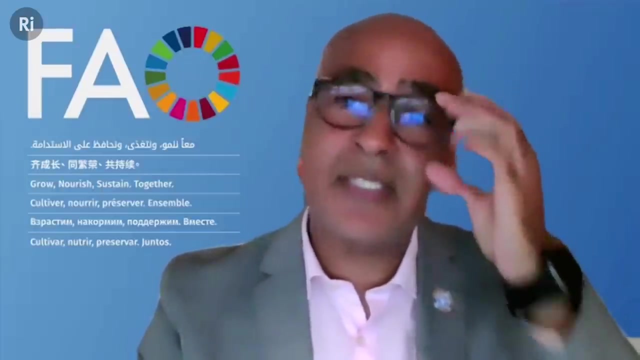 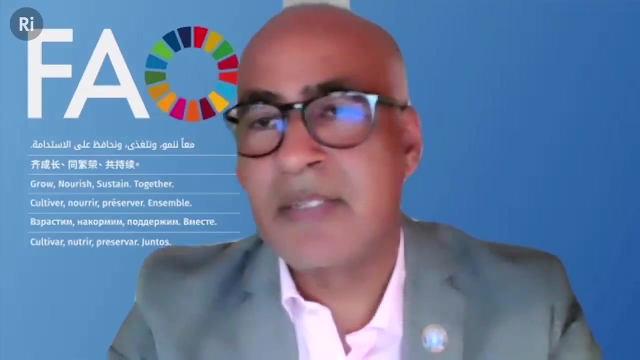 to ensure resilient, inclusive and sustainable agri-food systems, And every year we publish a report that is the state of food security and nutrition in the world, called SOFI, And this year we found that between 720 and 811 million people are going hungry following a year of lockdowns. 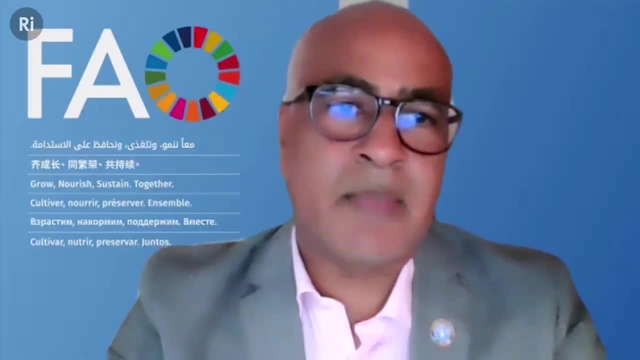 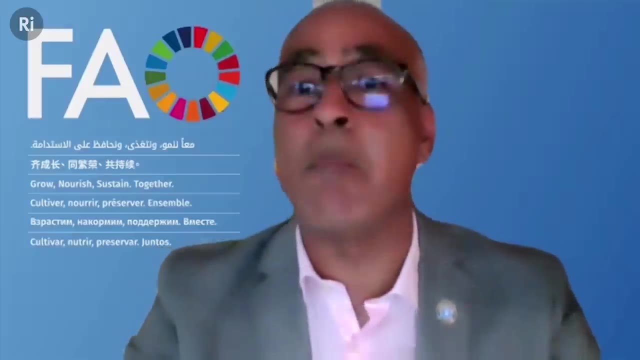 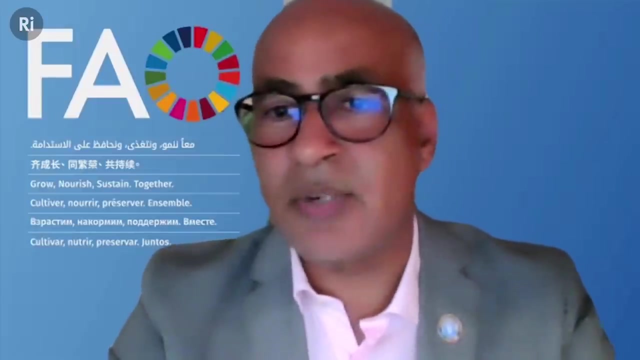 and stalling global economy. So what this means is that, again, we have the urgency really to transform our agri-food systems to make them more efficient, resilient, inclusive and sustainable, so that everyone can have access to affordable, healthy diet. 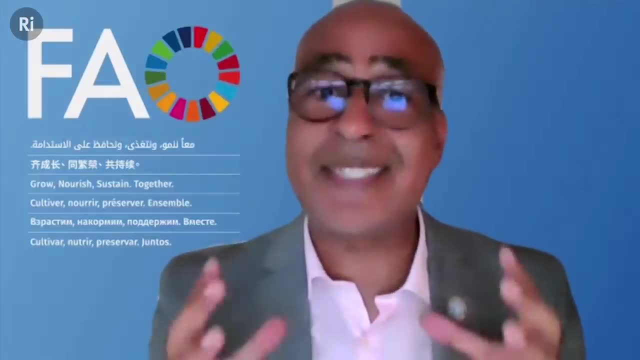 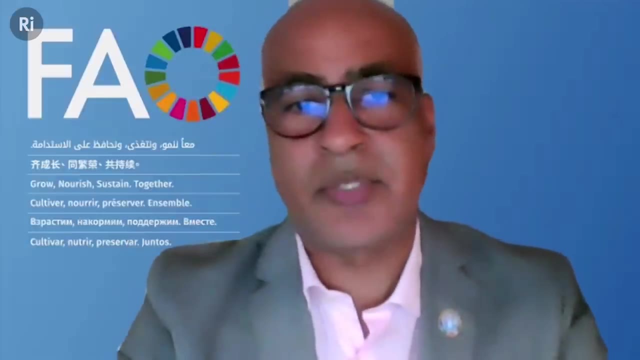 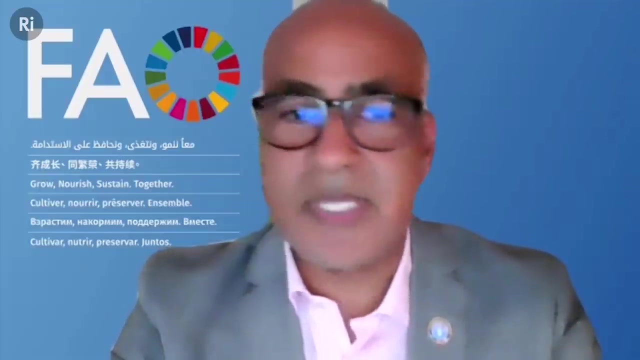 So unless we acknowledge really all these challenges and the scale and seriousness of the problem and act big and fast, then we're not going to be able to solve climate emergency and the biodiversity crisis and we're not going to be able to achieve the sustainable development. 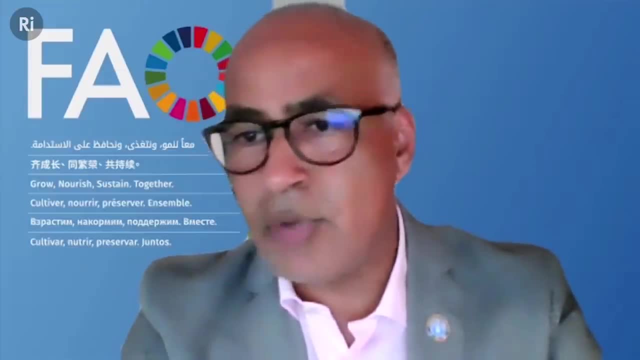 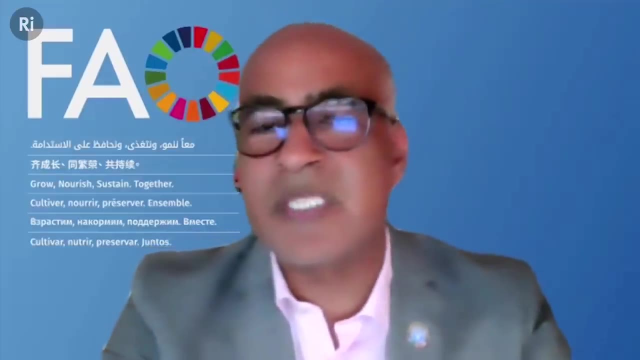 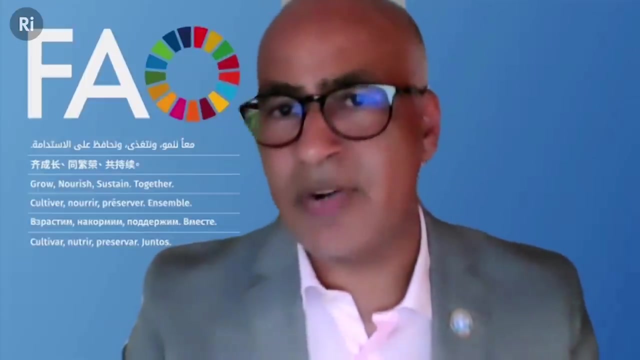 goals. So there are major events happening this year, as you know: the Food Systems Summit, the Conference of the Parties on Biodiversity, the Conference of Parties on Climate Change, COP26.. This will be in Glasgow in the UK, And these are all opportunities really to rethink our connection. 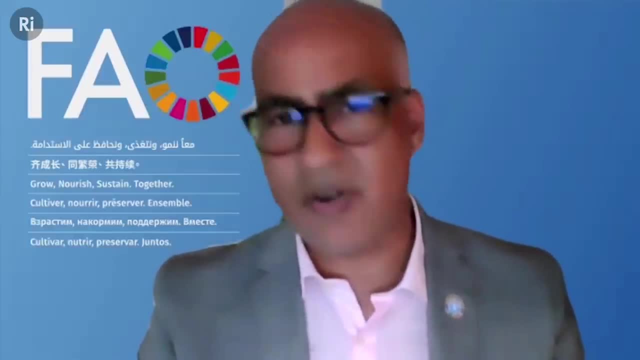 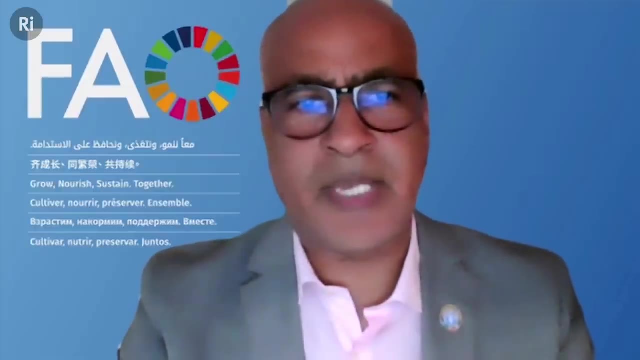 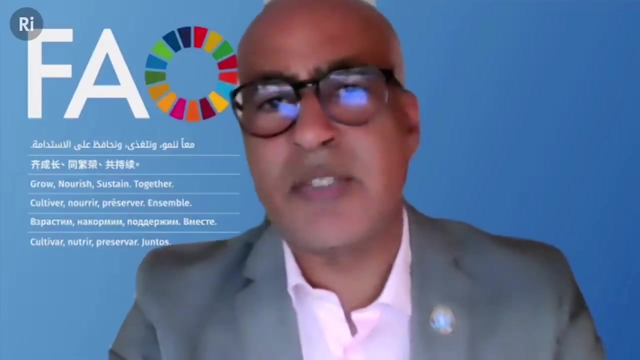 with the environment, with nature, with the climate, to rethink our behavior, how we use food, how we grow it, how we distribute it, and to think about sustainability in the long term. And, as you probably know, the Food Systems Summit which is going to be convened by the UN Secretary. 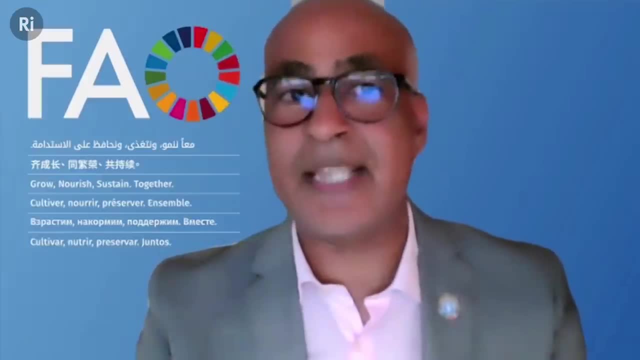 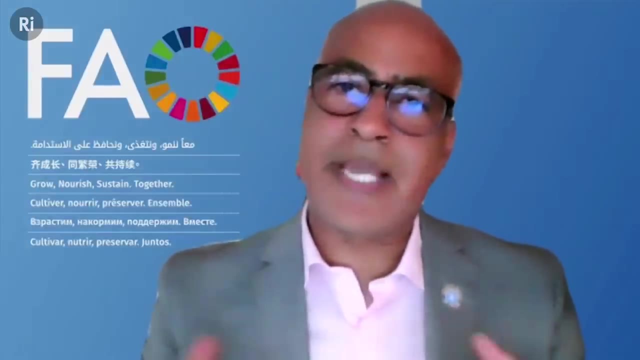 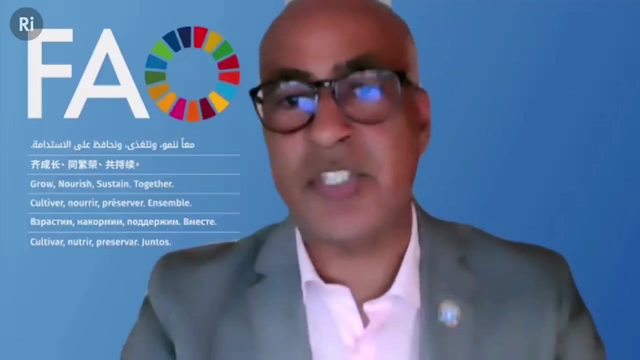 General as part of this decade. we're living in the decade of of action to achieve the sustainable development goals by 2030,. the summit is going to look at what we call game changing solutions towards achieving food security and tackling the impact of climate change and biodiversity loss. So these are opportunities that we really need. 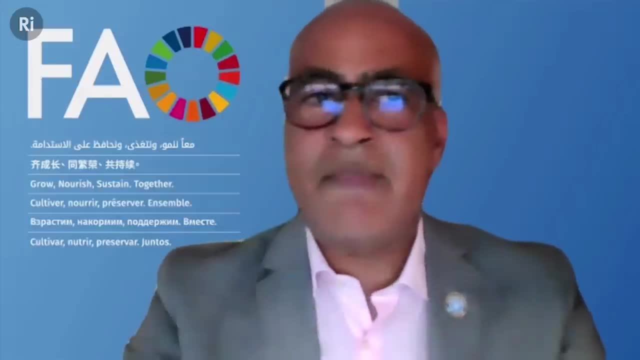 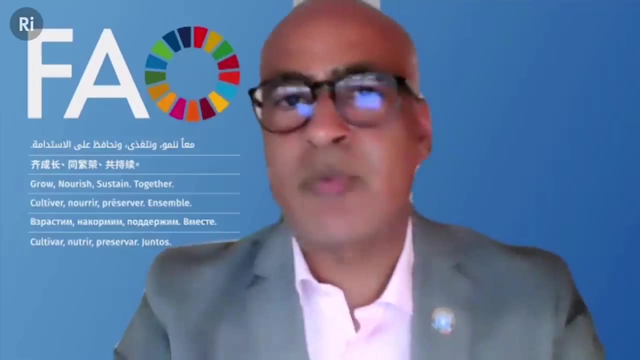 to capitalize on. So really, everyone has a role to play. And back to our event today, Age of Extinction, I would say what should we do about it? and so this is our topic today, and our panelists will discuss the psychology behind climate change and biodiversity, and what information and stories 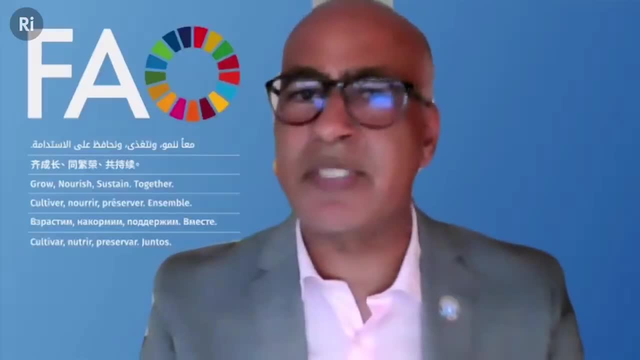 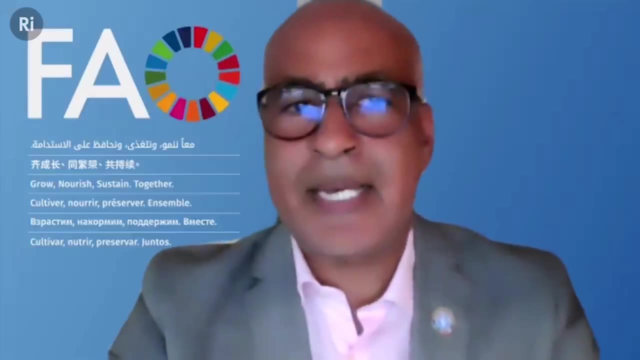 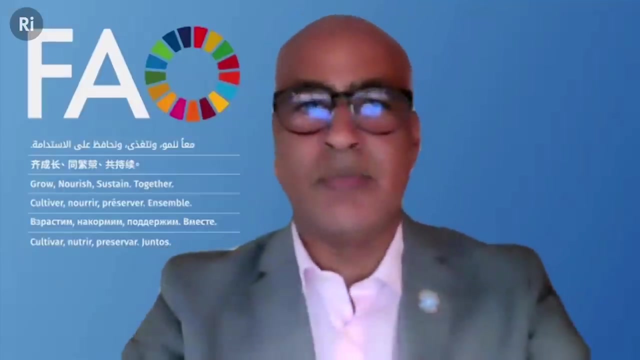 that work really to keep people involved, keep people engaged and positive about the future and to act. as i said, everyone needs to do their bit, and how can climate professionals really discuss their work in public without you know the doom and gloom as we say? so i'm really very 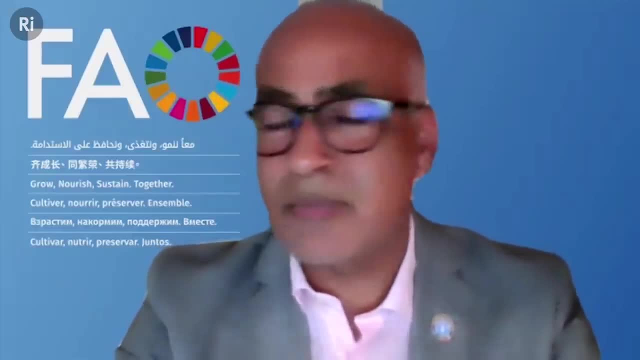 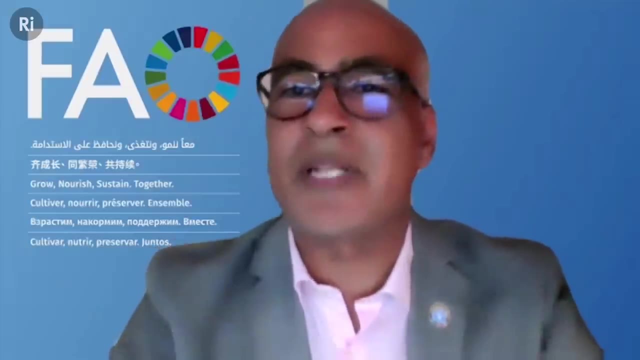 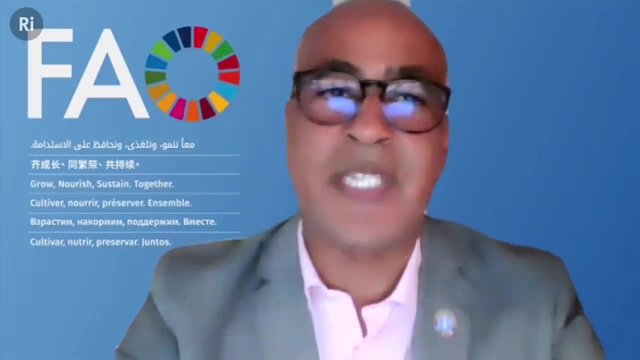 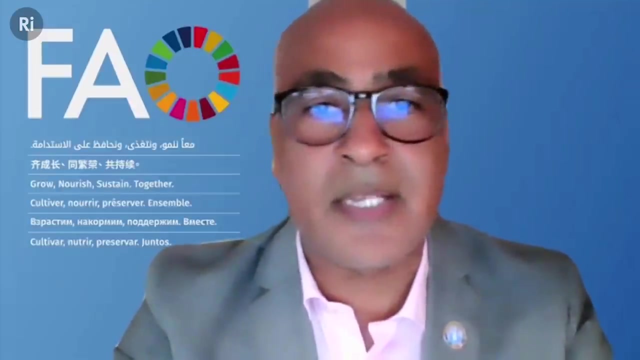 pleased that today we're joined by four experts from a diverse background: uh tilly collins, who's a senior fellow in the center for environmental policy at imperial college, london. she publishes regularly on aspects related to urban ecology, ontology and sustainability. our second speaker is um sahana gosh, who's a science uh journalist focusing on biodiversity at the mongabi, india. 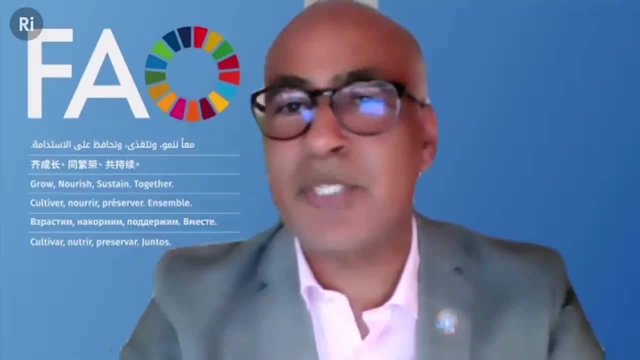 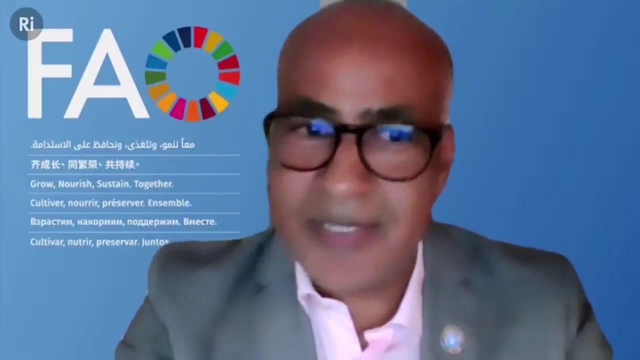 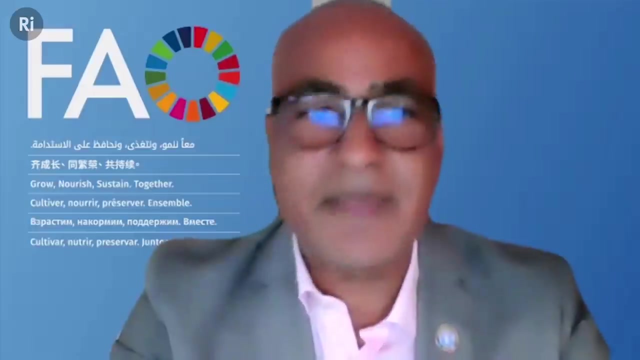 she reports particularly on biodiversity, climate change, environmental health and gender, and she's also the coordinating editor for beyond protected areas and natural climate solutions special reporting project at mongabi. and our third speaker is, uh, nicola davis english, who is the an english zoologist and children's book writer. um so, she was one of the original presenters of the bbc children's. 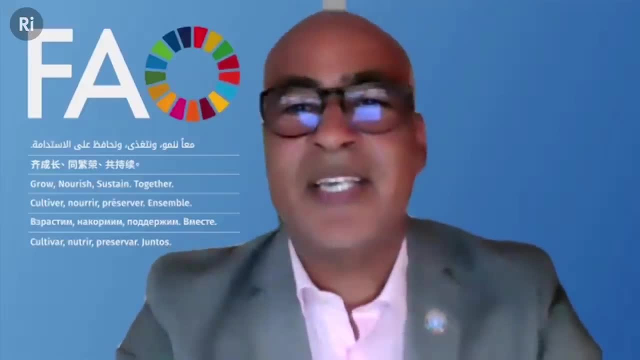 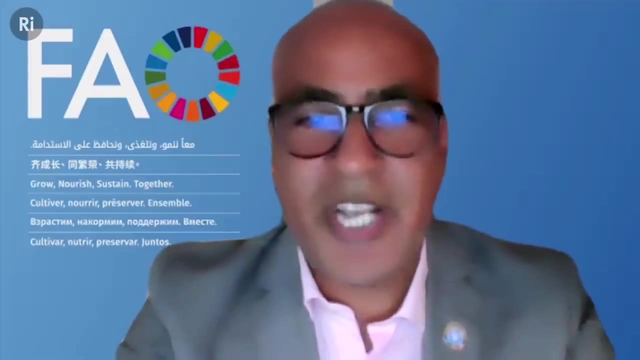 wildlife program, the really wild show, and more recently, she has made her name as a children's author. our fourth speaker is miss angeline chen, who is the co-founder director of development and partnerships of the global coalitions, and she holds a master's degree in international relations and affairs from university. hillary kirkton are from india andjar goes to bbc. the womanagua for dates and future studies should speak for her teaching international relations and affairs from university. um, so i'm here to tell you that. first let me introduce myself. Ein�cushman, how are you and me for these? 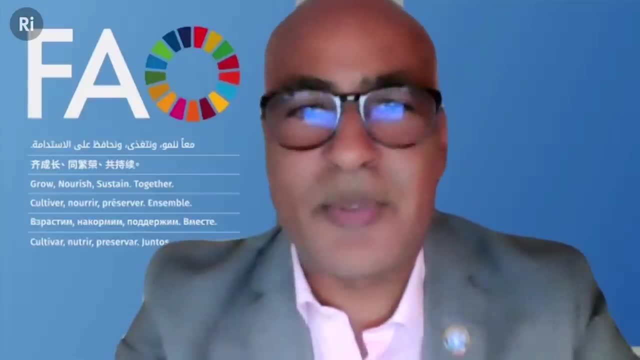 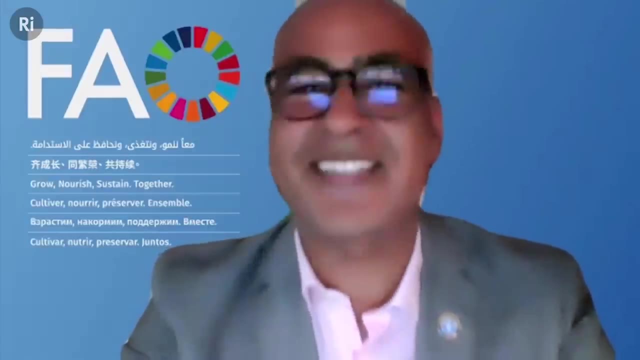 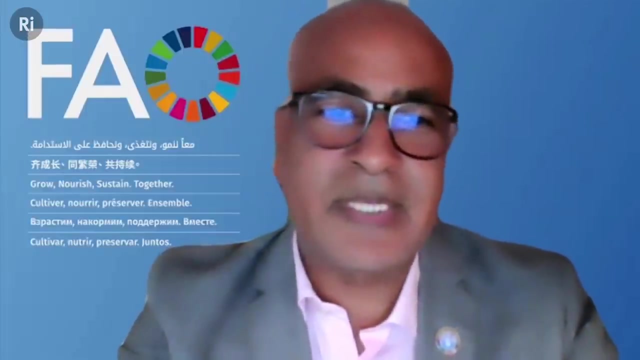 the University of California, Santiago. So thank you for all our speakers for joining us. Just to remind each speaker that you have 10 minutes. then we can move to the questions and answers where I would like to involve the audience. So for those of you joining us, 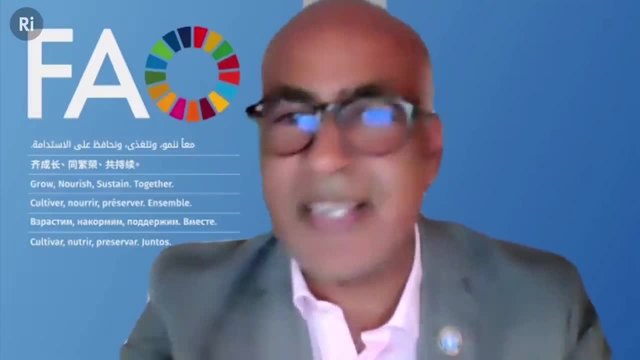 please post your questions, your thoughts, anything you want to share with us in the chat box. And for questions in particular, please post your question. I will put them to our expert later on. So with this introduction, I would like now to invite Tilly Collins. 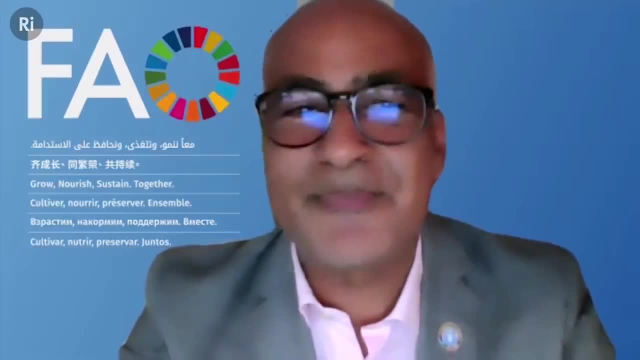 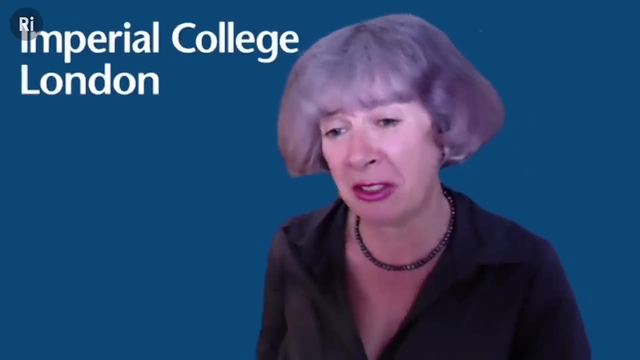 who will give her first presentation. Tilly over to you Good evening and thank you so much for inviting me to join you, And I cannot help but echo your words. I think we need to act big and we need to act fast. 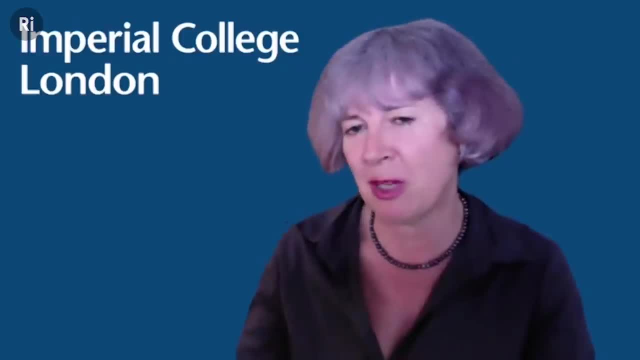 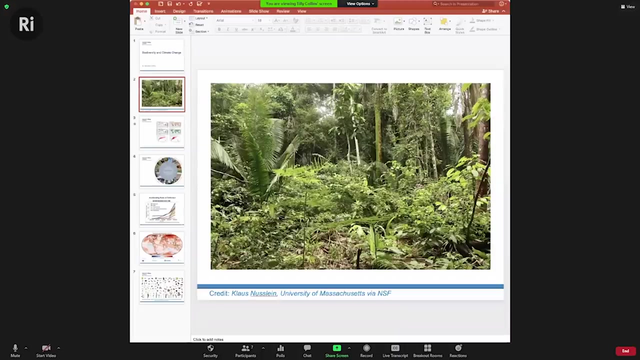 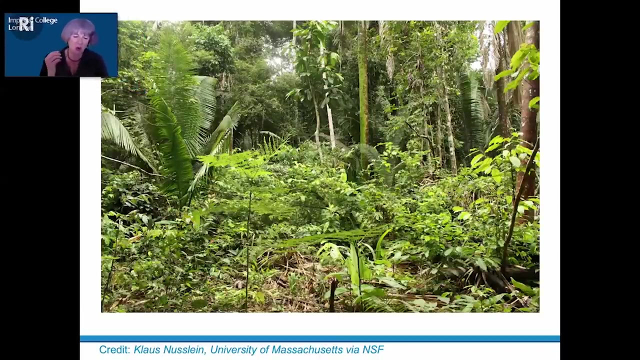 And we're extremely fortunate that we're beginning to be in a position where this is starting to be possible. But really my role this evening is to start to think about what biodiversity is and how we describe it and how we use it. really, I think that most people have a really clear notion. 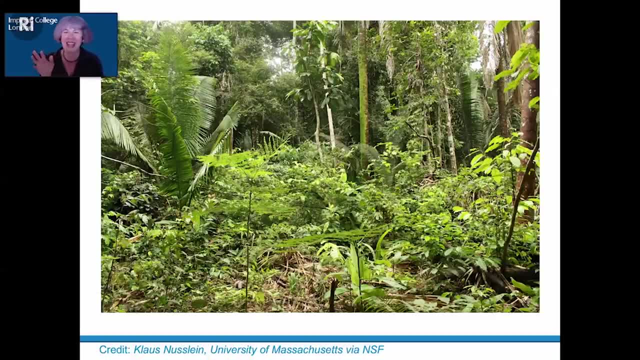 that biodiversity is the sum and the detail of all the living things that surround us. Much of that is visible, like here in this picture, But the vast majority is invisible because it sits below the ground. It sits in the soil or deep in forests or in the oceans. 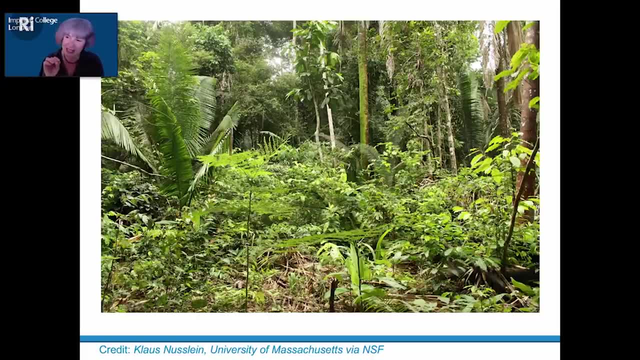 or at microscopic scales, where we don't really see it and our understanding is still quite limited. Ecology, which is essentially the science of biodiversity, seeks to understand why we see the species that we do where we are and where they are. To demonstrate this, I will introduce Tilly. 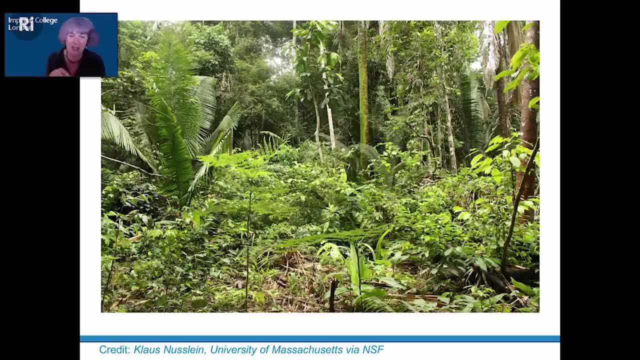 So what we do is we go to our regions, do where we do and in the numbers that we find them, And it's through a long practice of ecology that we have a clear idea of where we find the most biodiversity and that we can understand the multiple values and benefits of what we see. 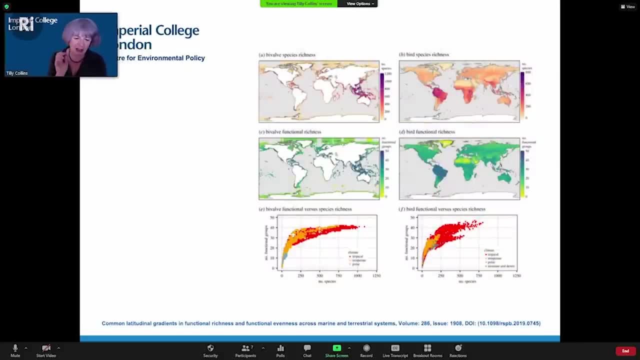 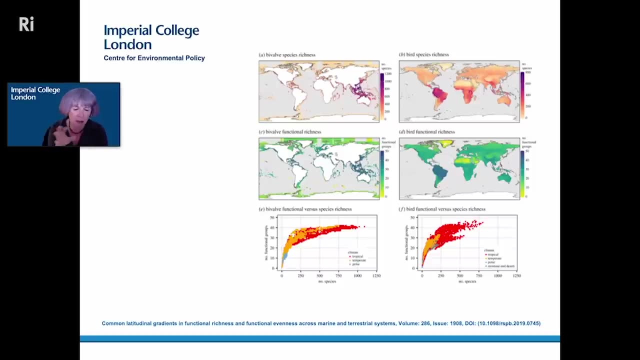 We observe that there are clear latitudinal gradients, simply really, that the tropics host many more species than the temperate zones and that the number of species present in environments tends to decline as we move northwards or southwards towards the poles. 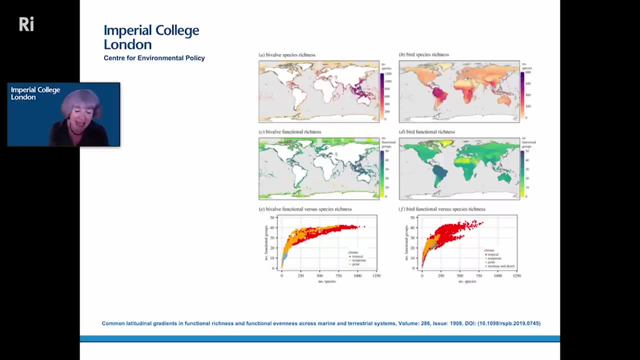 This pattern is thought to be driven by reasonably stable, year-round tropical weather ranges that allow very many niches in the tropical areas, and also, in part, due to the solar energy that hits those tropical areas, which is less seasonal than at the northern and southern latitudes. Water matters too. Arid areas such as the Sahara desert have much lower biodiversity than moist areas in the same band. For high levels of biodiversity, water must not only be present but also available. There's plenty of water in the global north, across Russia. 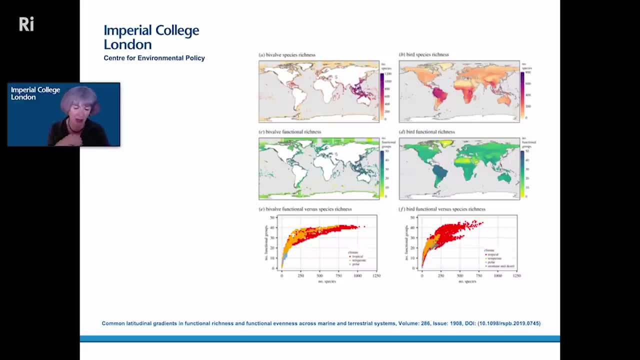 but it's locked up in ice a lot of the time and many organisms just can't use it. This consistent availability of water affects biodiversity and affects the amount of biodiversity that any region can host. In many mountainous areas, there's seasonal water availability. 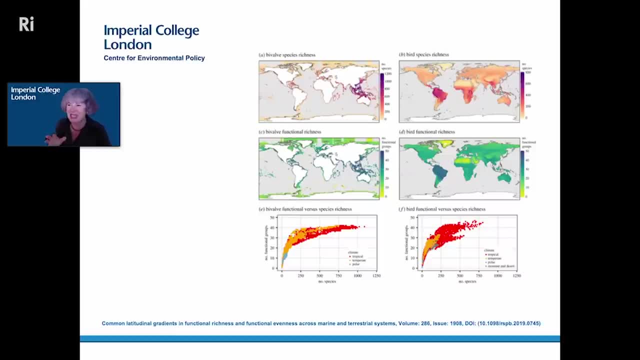 but the rain that falls isn't retained in thin soils. it flows down the mountains, leaving seasonal droughts which that limit the plant growth and consequently reducing its microplased. Japanese umbrellas biodiversity of those areas. Flatterlands, with their deeper soils, host much more biodiversity. 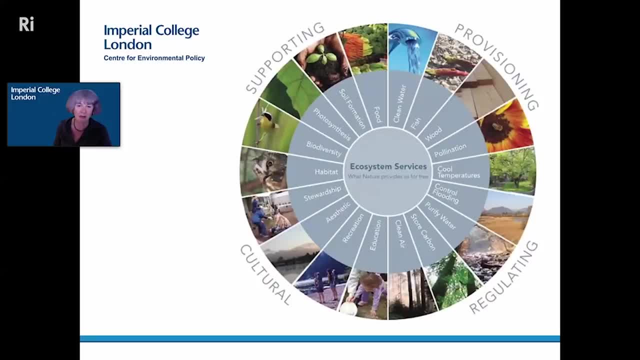 because they hold water for longer. The natural systems and ecosystems in the world. they serve and support us. they provision us with food, they provision us with fresh water, they regulate our atmosphere, they regulate our climate and nutrient cycles. they make soil, they sequester carbon and 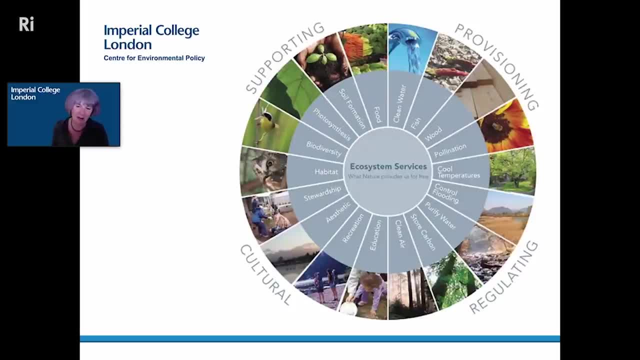 they provide cultural and aesthetic experiences. These are the ecosystem services that biodiversity provides and on which we depend. They are our natural capital, and their intrinsic biodiversity, at whichever latitude, is what gives them their resilience. But by resilience I mean their ability to resist disasters and to recover rapidly and to continue to provide the services on which we depend. 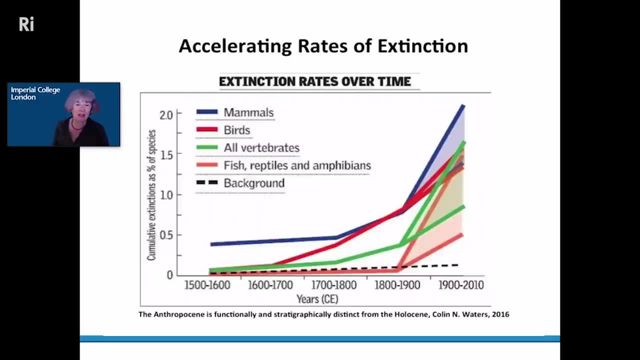 Ecology has also given us tools to count and thus the data to analyze these patterns, and, with paleoecology, giving us a clear sight of patterns through time. So biodiversity is not a constant, it's a pulsing thing. We've built us the tools we need to reach ourense. Pixie members, who are the reasons why we live where? 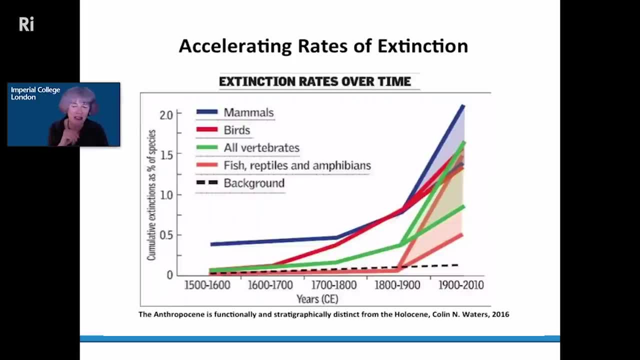 We've built us the tools we need to reach ourense. Pixie members, who are the reasons why we live where. We've built us the tools we need to reach ourense. Pixie members, who are the reasons why we live where- been through five major mass extinctions in the history of biology that we can identify. 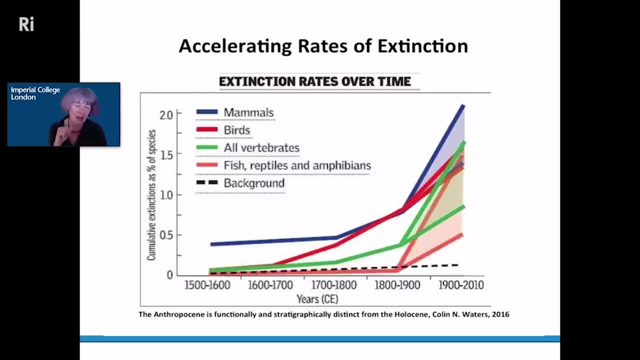 but we're now in a sixth, and we're in the first of its kind. this is an extinction driven by a single species present on the planet: we, the humans. we've directly transformed natural areas. we've taken the flatter wetter lands to produce food and fiber and other goods for our consumption. 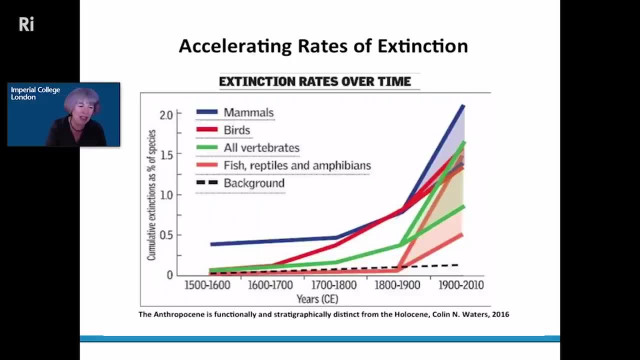 as we exist in greater numbers before and our individual footprints grow with our development status, so our influence can spread. farming is moving into drier areas and more distant lands. in order for us to produce the food we need, nature is pushed back into those areas where we are fewer. 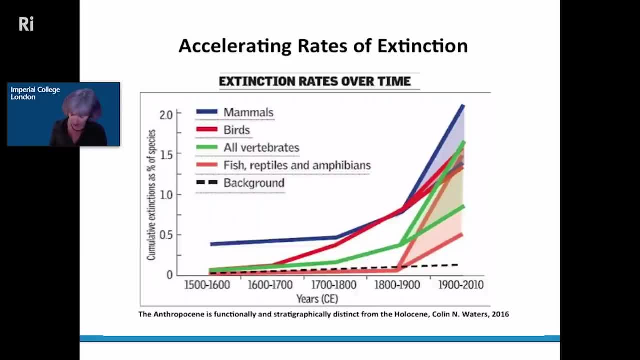 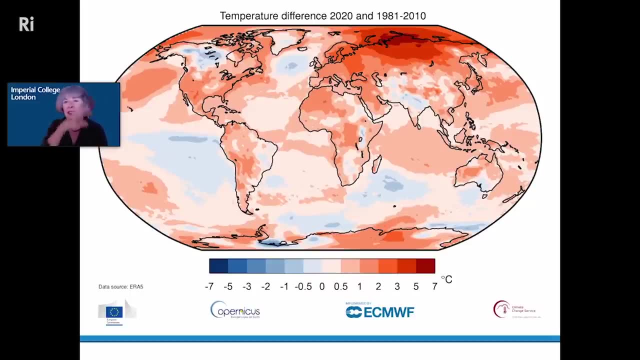 and farming is more challenging. so, along with the this habitat change, we have now changed the climate by influencing the atmospheric gases that insulate us. this change is is evolutionarily extremely rapid and has profound consequences for the ecosystems of all regions, including those of the global south, where much of the biodiversity 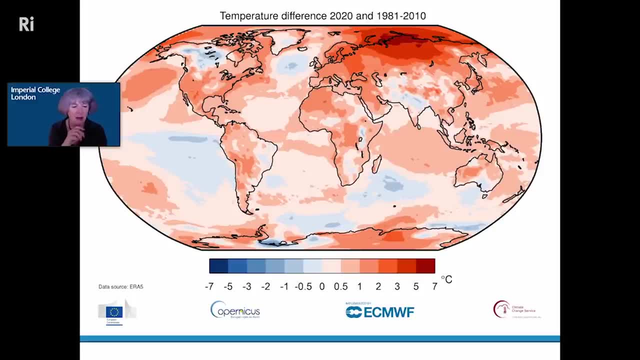 is concentrated. climate change acts much faster than evolution, can deliver adaptation and drive species to move their ranges. so organisms are pushed from areas where their adapted biological requirements are met and, when acting in concert with the habitat change, this tends to push species into less hospitable areas, such as further up the mountains or to where human influence is already great. 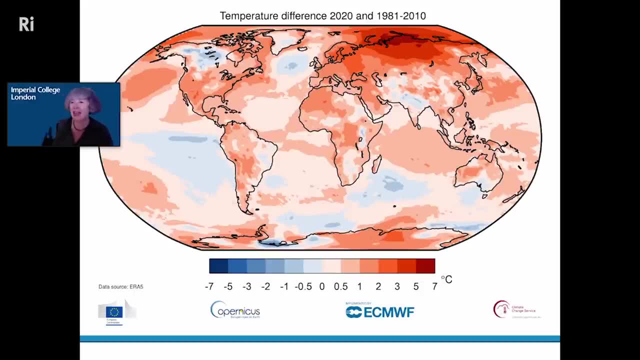 we may marvel when a new butterfly lands on the british shores, but that usually means that part of its former range has become uninhabitable. in this image you can see the warming scene up there in the north of russia that will allow conifers to grow. 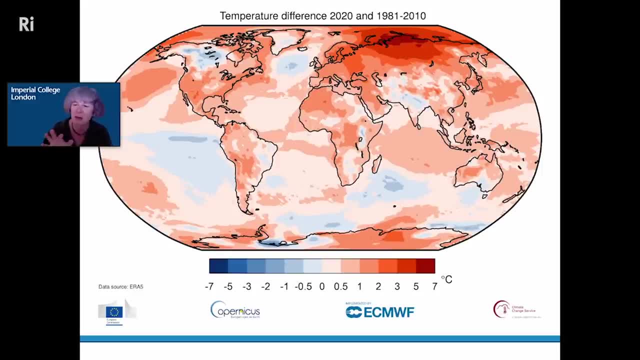 but those conifers will be darker than the surrounding landscape and that may exacerbate and drive further heating in those regions. climate change thus affects the weather and the temperature patterns of any natural area. zittouni mentioned the floods recently in germany, the canadian heat wave. 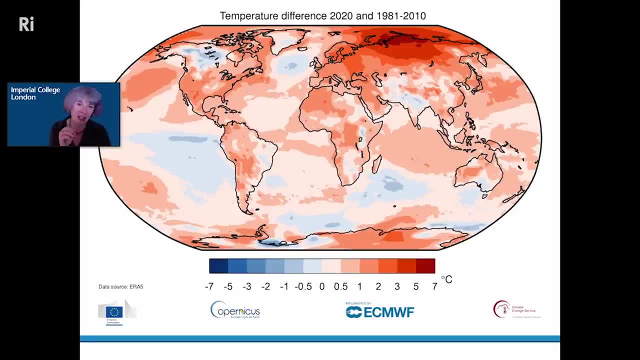 is a chemical plane. it may be a cause of climate change, but it causes city influences in the climate. thisếme is the law we wrote. we need climate change. as we go through the camera, we're seeing these changes and these changes affect the species composition of natural areas. 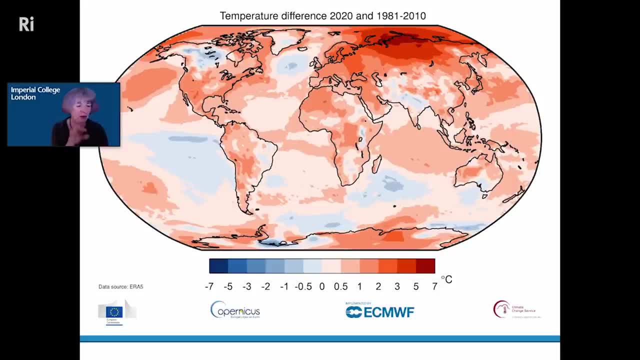 and then their resilience to cope with the catastrophes that come their way. so the climate driven change, climate change driven floods and frosts and heat waves that we see in these greater frequencies and at greater extremes will be vastly more devastating when there's no more ec jalum, when there's no more xiting to this kind of the situation. now to toxic air. if you have advanced genetic health research as a thermal and bio-fuel generation, so this is the case, apparently, in the context of where we certains, when you have been taking the climate change at most different plants scratching territory here, raise the blinker area you are happened to see on the ground. 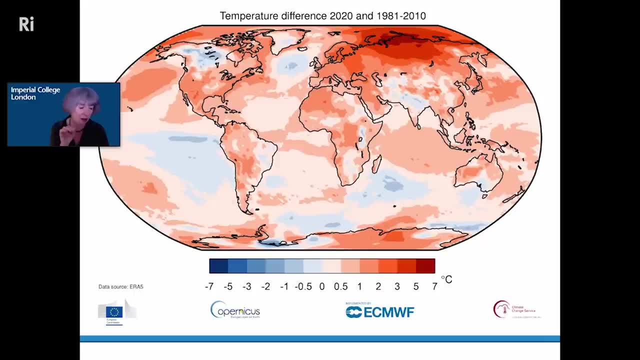 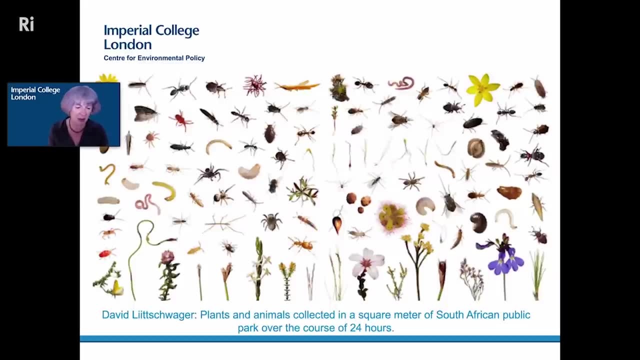 overstating to impoverished ecosystems and the services that they provide will be lost to us. There are very many things that we can do to help, and these all start with acceptance of facts and the understanding of the effects of our consumption patterns. There is no place now for 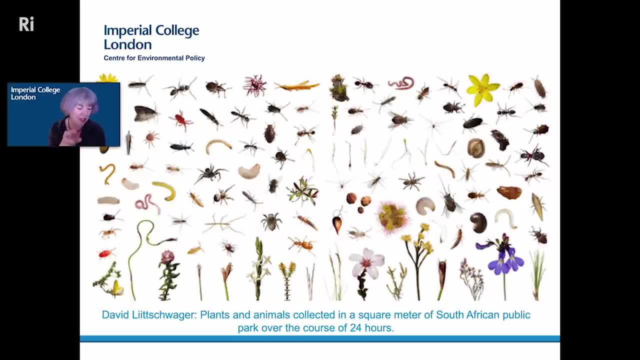 denial, and all the space in discussion must be for restoration and adaptation and technological improvement and growing efficiency, so that we can produce the goods that we need and want in a way that impinges much less on the natural world and brings greater equality of access for all. We must share the efficient technologies we develop and form resilient, long-term institutions. 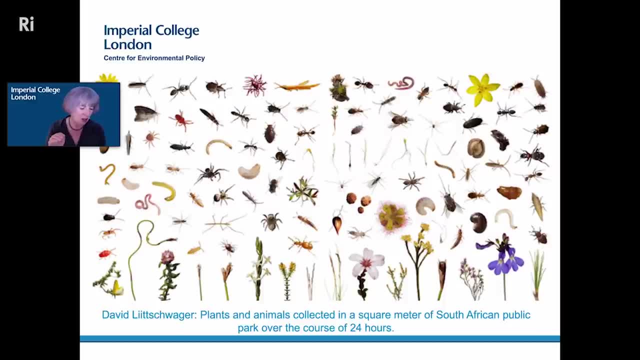 that we support. We need to work together to create business models that will reduce our effects On the natural world, both through direct action and through climatic alteration. the increasingly urban nature of people presents opportunities. It's efficient to keep people in cities. With improved urban designs, we can give space to integrating semi-natural ecosystems. 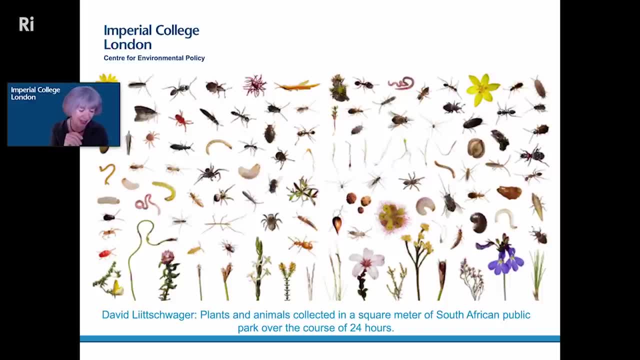 and the services these provide to our cities, while creating the space to restore natural environments outside of our cities. We can create a world where we can create a world where we can create a world where we can. We can create a world where we can create a world where we can create a world where we can. 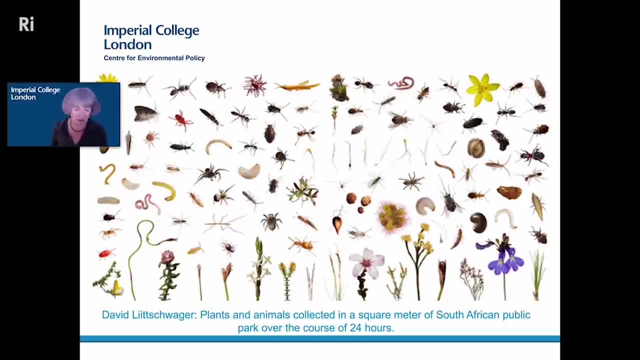 work at smaller scales as well, so any restoration or diversity enhancement matters. Even small steps that we make give us power. I urge you to plant. Plant so that insects can feed and that soil organisms can prosper. Plant so that your hearts are uplifted when you see green space. 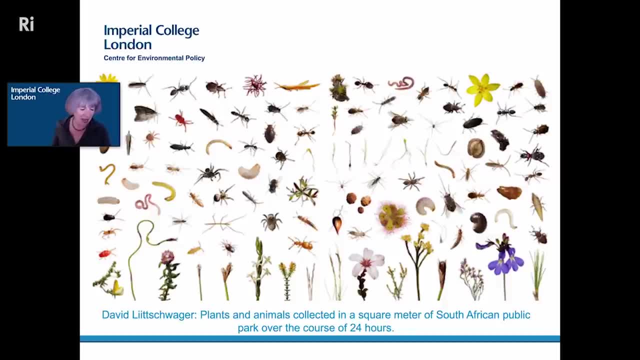 Plant so that carbon can be taken up and held at every single scale. The climate change that is happening can be acted on at many different scales, and we must protect and enhance biodiversity, both for its own sake and for ours. We need to act big. we need to. 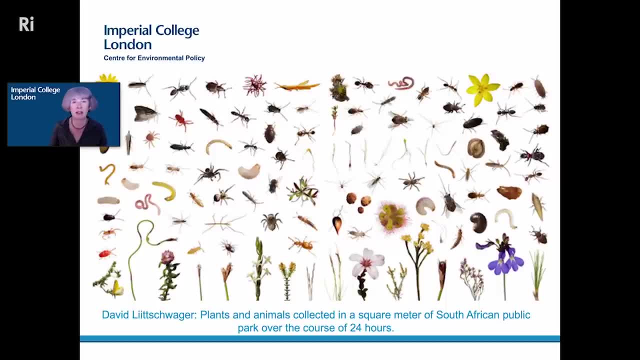 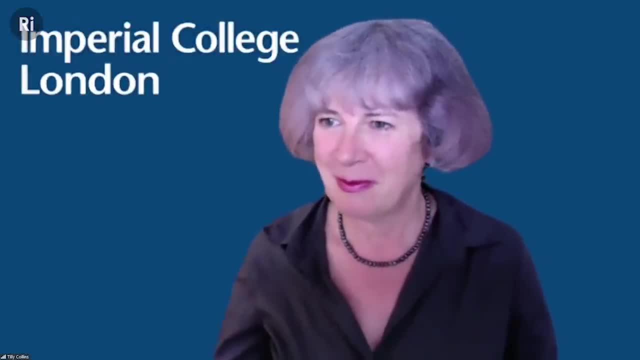 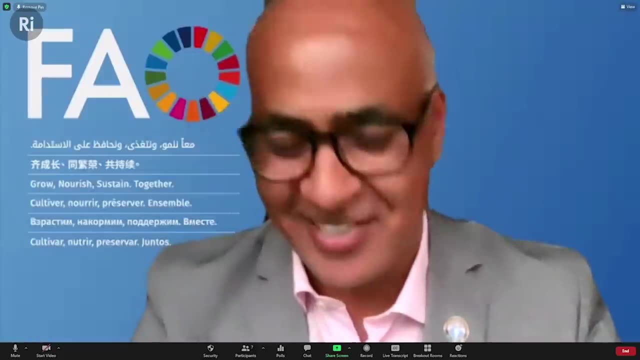 act fast and we need to come together to put pressure on this happening. Thank you, Brilliant Julie. Thank you very much. Thank you very much. Thank you very much, Tilly, And that's hot on 10 minutes, Thank you, And thank you for a great introduction. 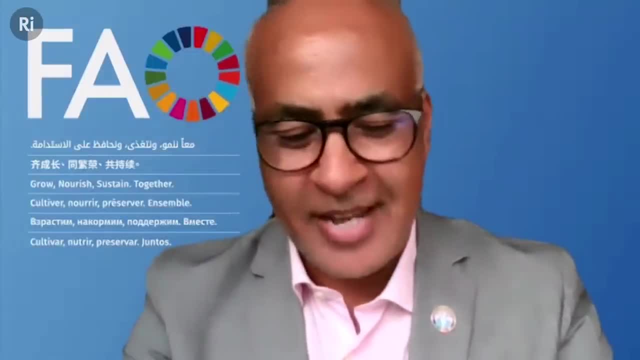 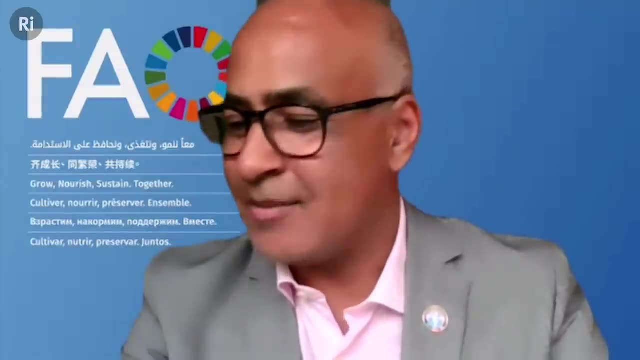 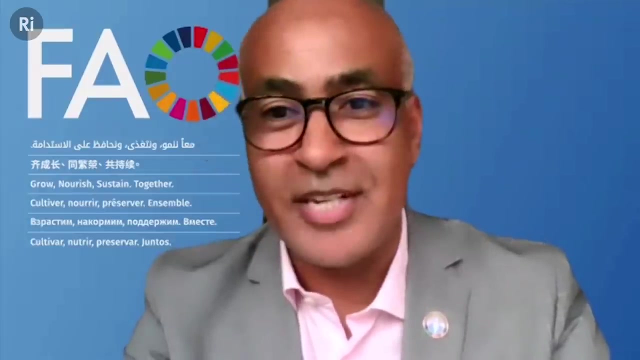 I just pick up one, one thing. I mean, you said so many facts are really very helpful- and just pick up one thing which you said: to accept the facts and make sure that we move into restoration, adaptation and take advantage of technological innovation, I think that's the way forward, Absolutely, Because the impact is already there. 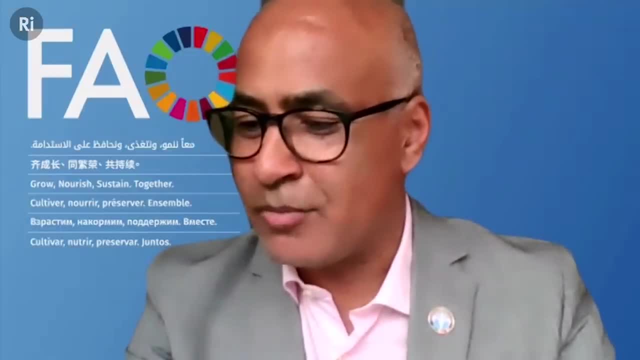 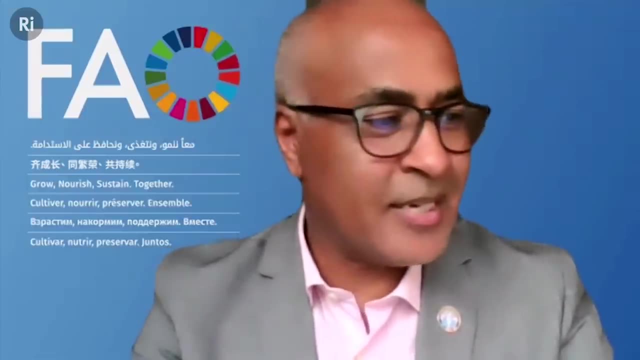 That's amazing. And on restoration, I just want to mention that from this year, we've entered, actually, the decade of ecosystem restoration. Basically, we have 10 years to restore the planet really, So the same as climate change, more or less. 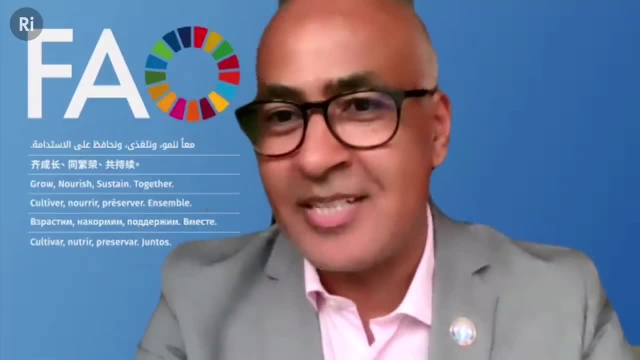 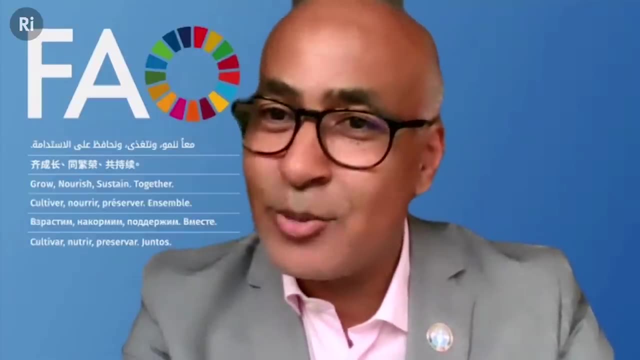 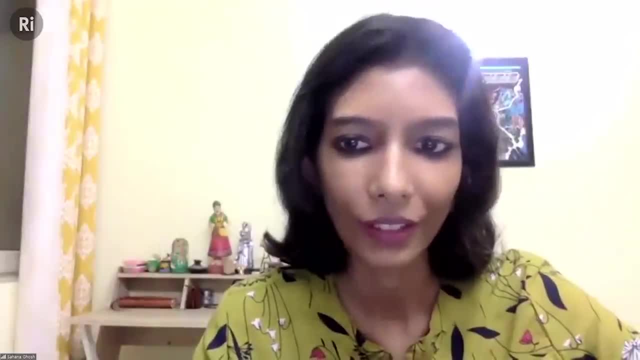 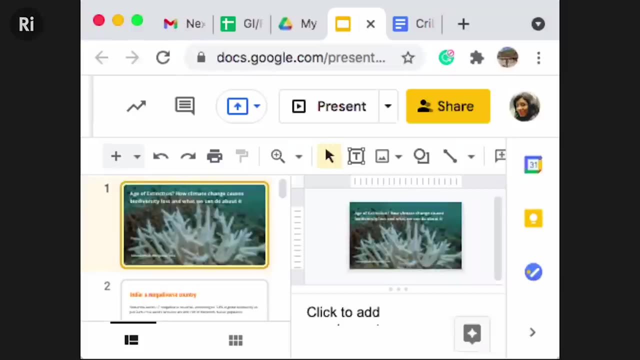 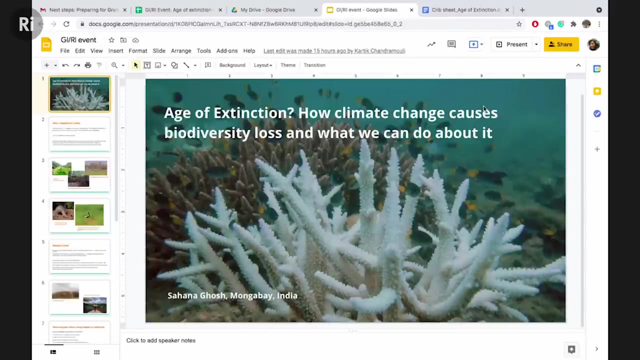 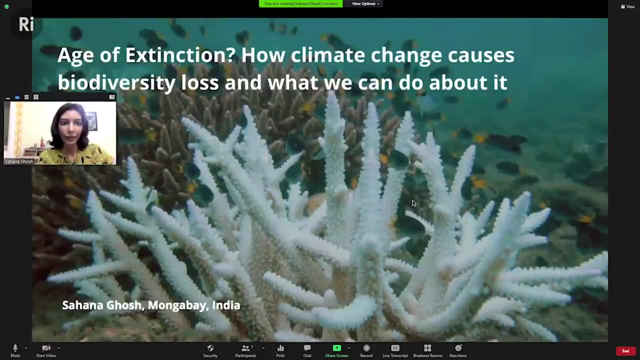 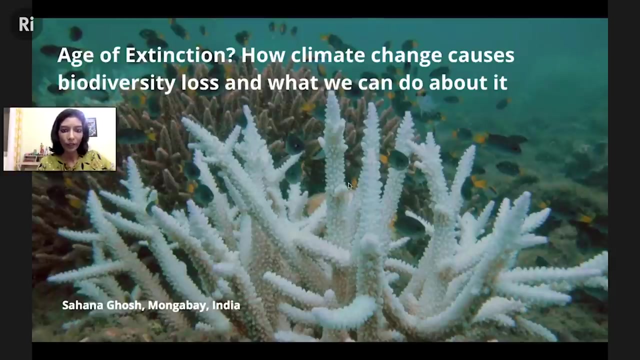 Thank you. Thank you, Sathuni. I'll try to sort of take you all through a trip to India, And so I'm Sahana and I'm a science journalist And I'll be talking to you. what exactly are we doing in India, And 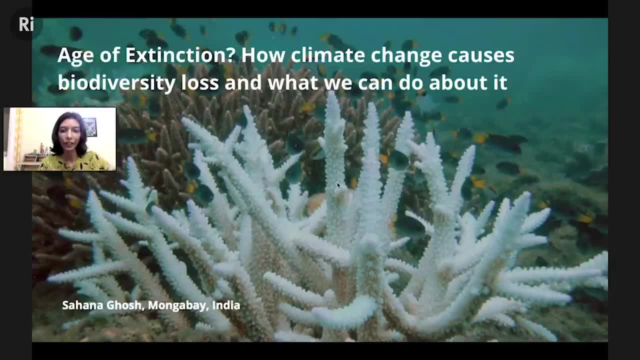 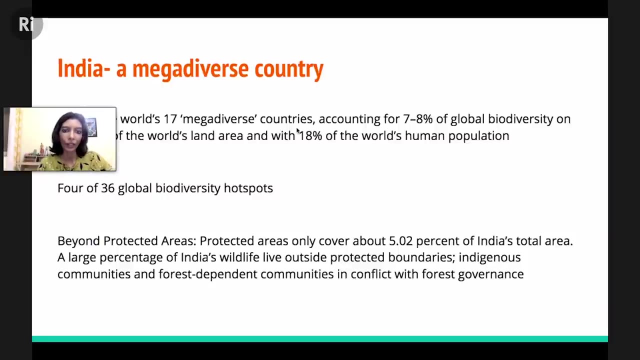 as journalists, what are our responsibilities? As Tilly said, accept the facts and, carrying on from what Satuni said about the UN Decade of Ecological Restoration. So, as you know, India is a mega diverse country And in this landmass in India, you know we've got about. 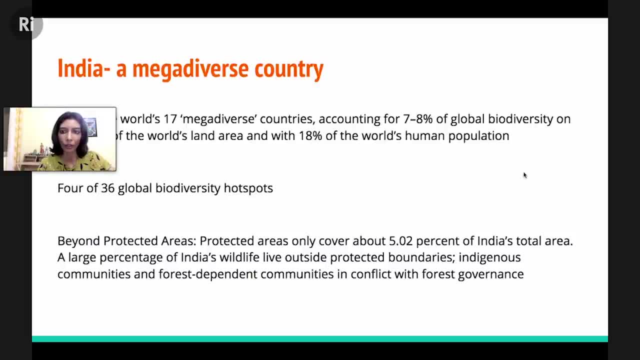 seven to 8% of global biodiversity. that's sort of squeezed in 2.4% of the world's land area And we are sharing this biodiversity with 18% of the world's human population. Now we've got in India. 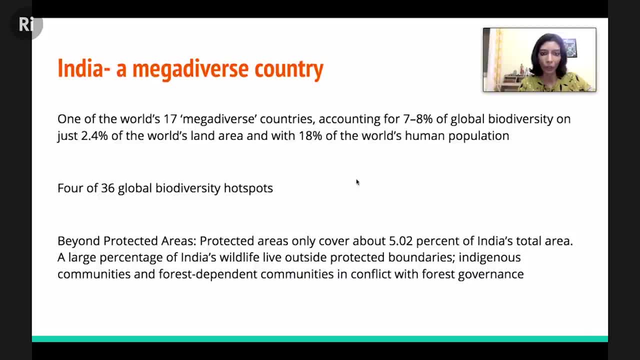 we've got about four of 36 global biodiversity hotspots And what's important is that we have protected areas, you know, but these only cover about 5% of India's landmass And a large percentage of India's wildlife live outside these protected areas, which means that there are 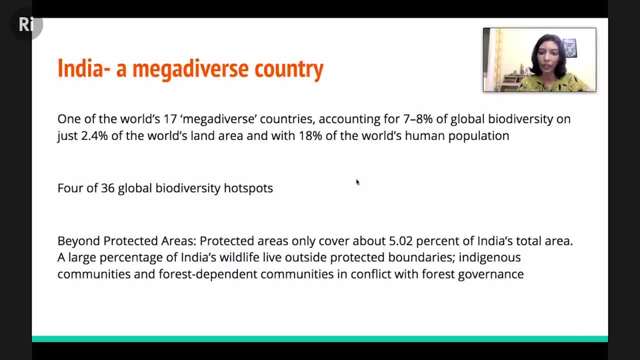 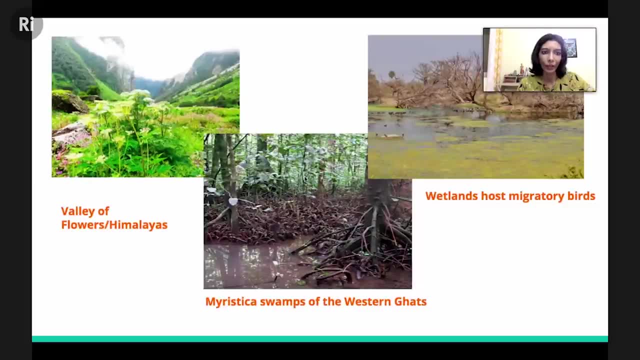 frequent conflicts with communities that are living around the edges of these forest areas, of these protected forests. Now, as you can see from this slide, there are these lovely landscapes in India. you know, these variety of habitats in India we have. we've got the Himalayas, we've got. 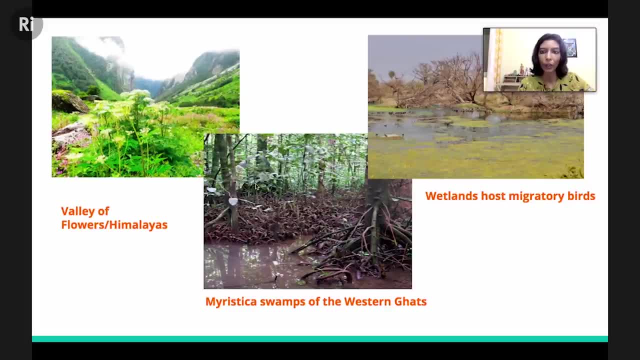 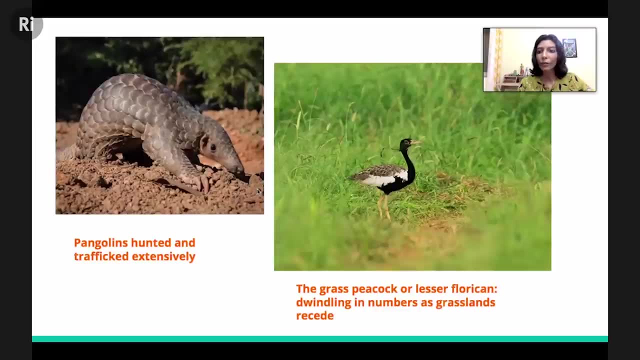 the swamps. in the Western Ghats, in the southern parts of India, we've got lush wetlands that are that host migratory birds that come from afar, And in these landscapes we've got some of the most endangered species of wildlife- pangolins- that are being hunted and trafficked extensively. 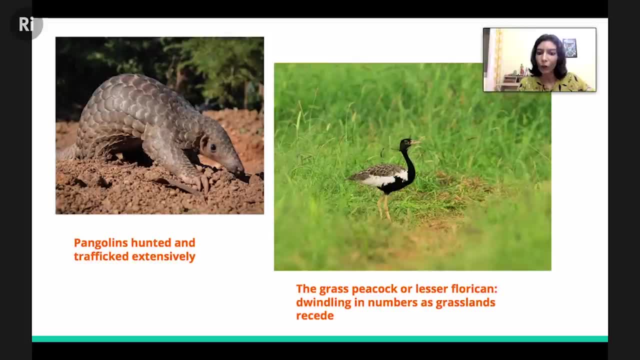 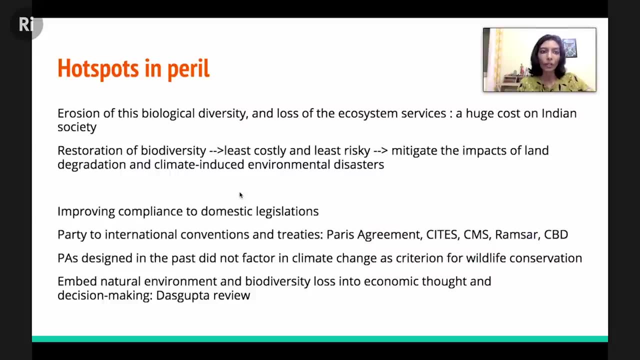 we've got these beautiful birds, like the lesser florican, which are dwindling in numbers as grasslands are receding, And so we know that our, that our hotspots are in peril. And and why is this important? Because erosion of this biological diversity, this ecosystem services. 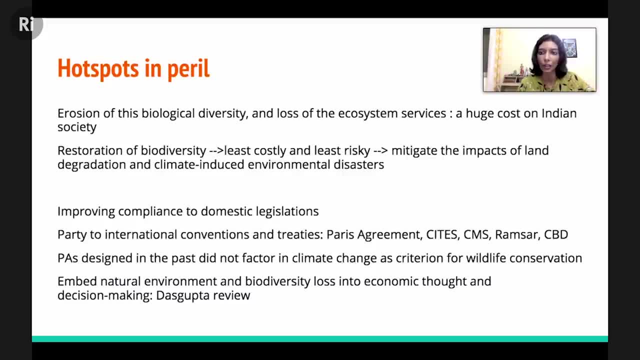 which is so intricately connected to communities in India. it's a huge cost to our society, And so, of course, restoration of biodiversity is perhaps one of the most least costly and least risky way to mitigate the impacts of climate change. But, at the same time, India has to contend with a lot of 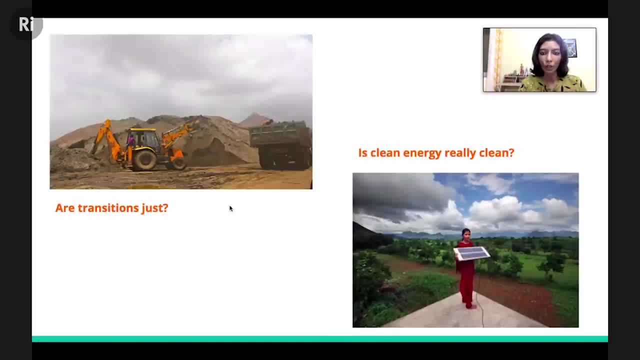 factors. you know we are party to a lot of international treaties, including the Paris Agreement, including the CMS, CBD, all these important global agreements cards. We've got to comply with domestic legislations within our country And, at the same time, we are gearing up to be a global superpower And there's a lot of transitions. 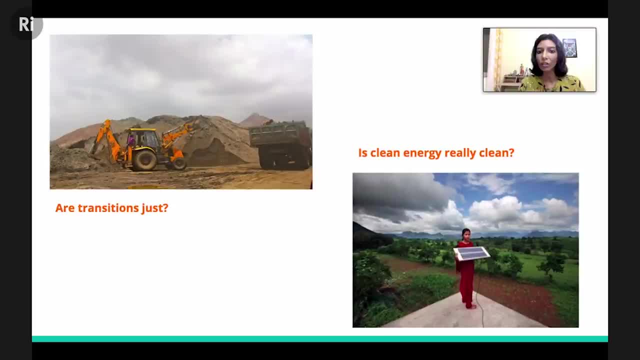 that are happening. There's a lot of mining, there's a lot of energy transitions And we are wondering: are these transitions just? At the same time, there's a buzz on clean energy, So we are also wondering: is clean energy really clean And what are the trade-offs in clean energy? 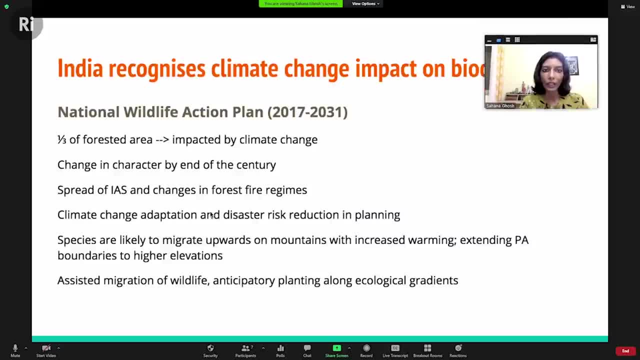 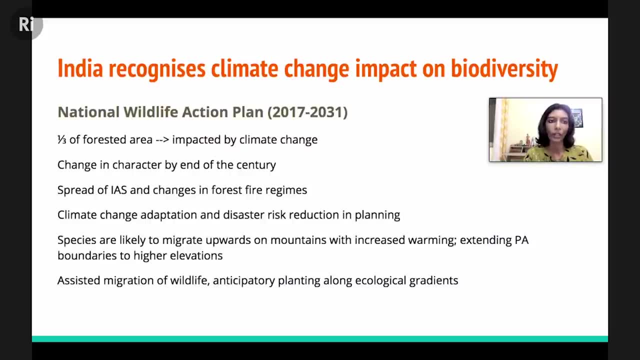 But what we know is that India has recognized climate change as a factor that's contributing to impacts on biodiversity And in our National Wildlife Action Plan. what India says is that it discusses the spread of invasive species. It discusses changes in forest fire regimes due to 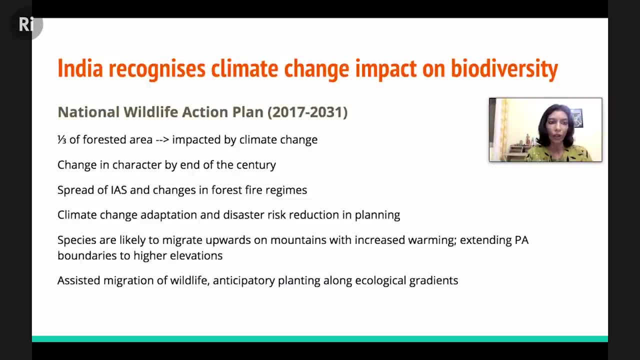 climate change. It discusses the predictions of how much of forested area are going to be impacted by climate change, And also it discusses the impact of climate change on climate change, And also it discusses the impact of climate change on climate change, And also. 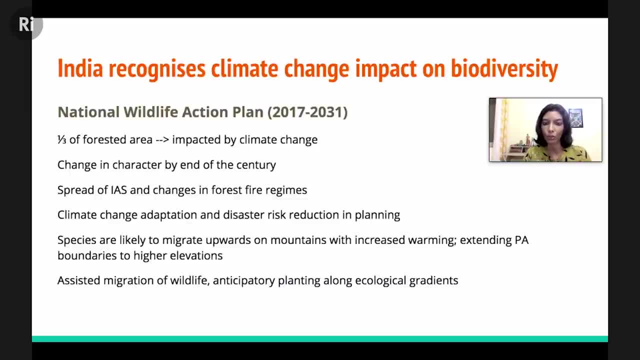 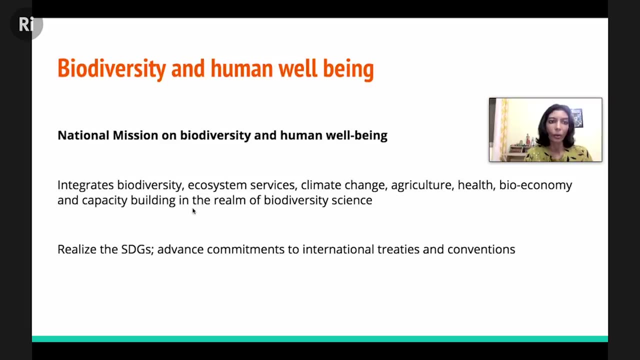 it also talks of species that change their distributions due to increased warming. At the same time, what we are also recognizing that we also probably need to go for assisted migration of wildlife and anticipatory planting along ecological gradients, And there's a very strong recognition that biodiversity and human well-being are closely linked together And with the COVID-19. 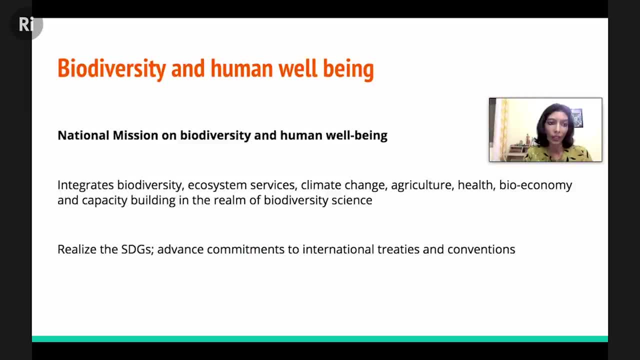 pandemic. this has become more evident than ever. And why are we talking of biodiversity and human well-being? Well, because India also has a national mission on biodiversity and human well-being And this will sort of help us realize the SDGs, sort of help us. 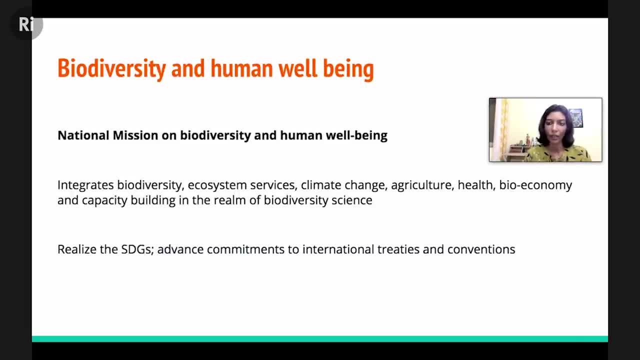 advance commitments to international treaties and conventions And SDGs, as Zituni and Tilly mentioned, that these are important goals that we really need to recognize And we need to recognize the intersectionalities of all these factors together. It's biodiversities, ecosystem services. 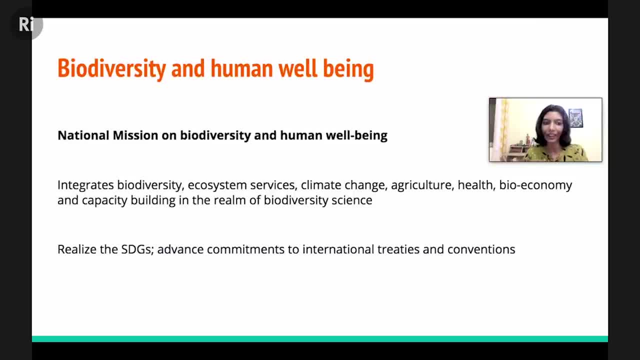 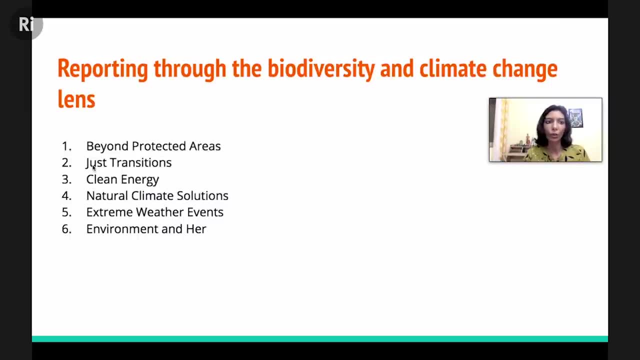 climate change, agriculture, food security, health, And so this mission is sort of integrating all of these together. Now, as journalists, you know what is our role here. As journalists, you know we have to recognize the facts, We have to sort of ensure that the scientific facts go out to. 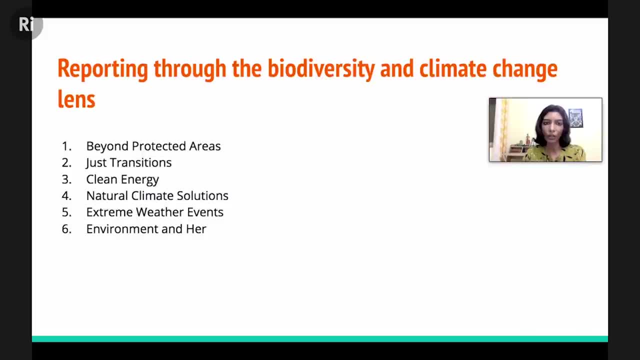 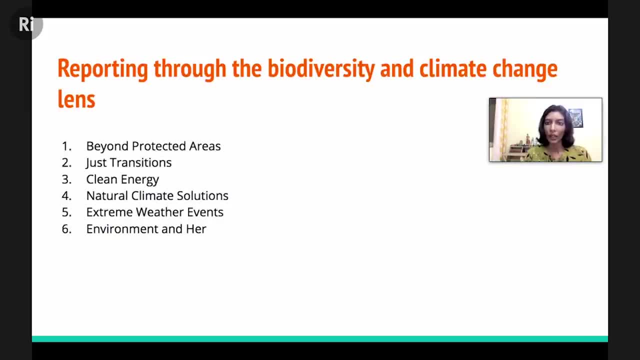 broad areas to cover biodiversity crisis and the climate emergency. So we are looking at wildlife and human interactions beyond protected areas. We are looking at these interactions in shared landscapes, in urban landscapes, in human-dominated landscapes. We are looking at just transitions. We are looking at mining, you know, and what is being done and how can these? 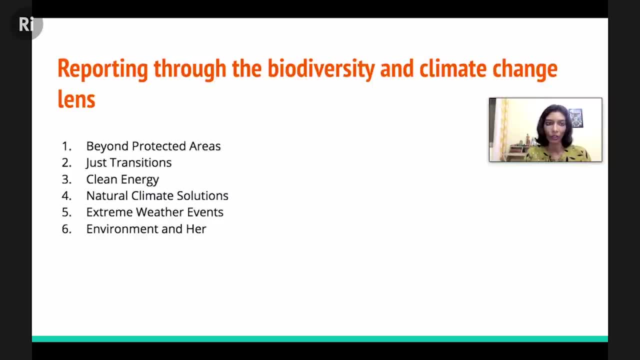 transitions be just to the communities that are involved in these transitions. We are looking at clean energy solutions, We are looking at nature-based climate solutions, which is the buzzword these days, And we are trying to sort of investigate: do these climate solutions actually work? And if they do work, 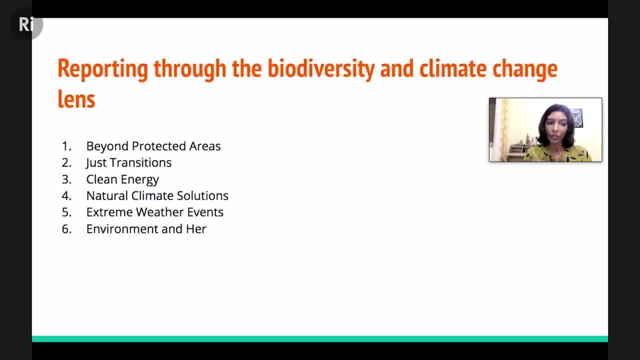 can they be replicated elsewhere? We are looking at extreme weather events, As you are all aware, you know that India is founded by cyclones and intensity, which has gone up in recent decades, And we are also looking at these events that are impacting our biodiversity as well. And last but, 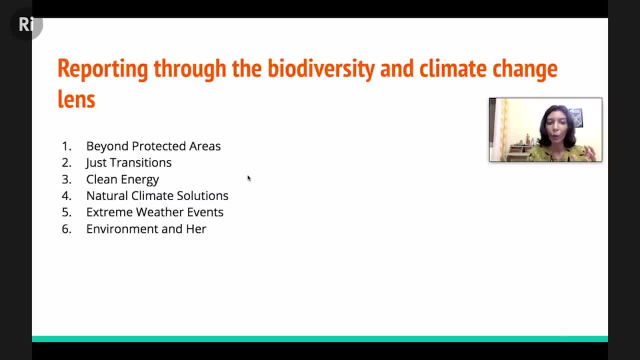 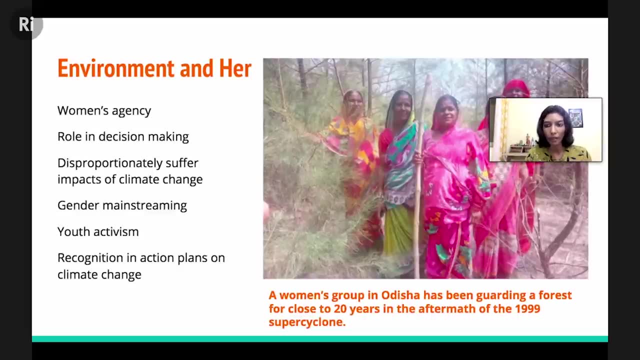 not the least, we are looking at climate solutions. We are looking at climate solutions, We are looking at gender, We are looking at women and their role in the environment. So we've got a series that sort of looks at women's agency in the environment, looks at their role in decision-making and how. 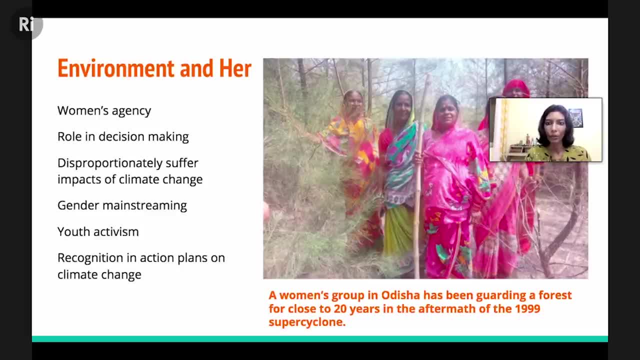 they are sort of tackling the challenges of climate change, Because what we know is that they are disproportionately impacted by climate change, And we are also trying to examine if gender is being mainstreamed by our national climate change. And we are also trying to examine if gender is. 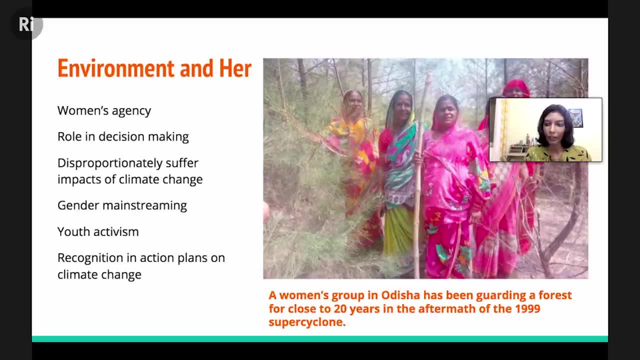 being mainstreamed by our national climate change, And we are also trying to examine if gender is being mainstreamed by our national climate change And, of course, youth activism, which has come up in recent years, you know. so we are also looking at all these factors together. So this is basically. 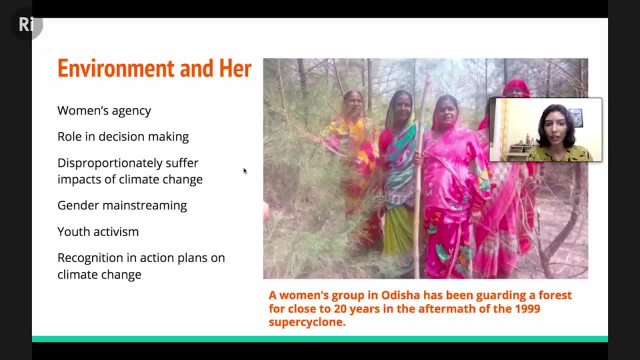 you know, we have to look at the intersectionalities of these areas. as journalists, It's a huge responsibility that we have And this is where experts like Tilly Zatini and others you know, who come in and sort of help us to inform the public, to inform policymakers. that you know. 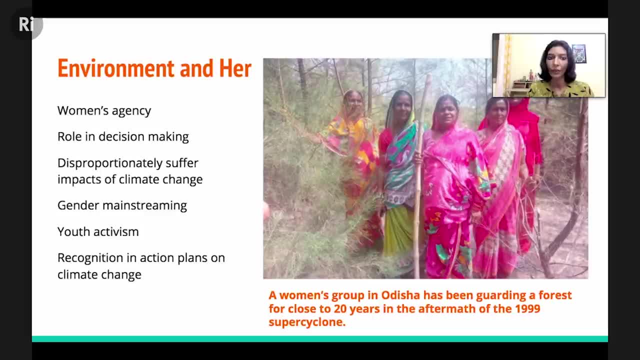 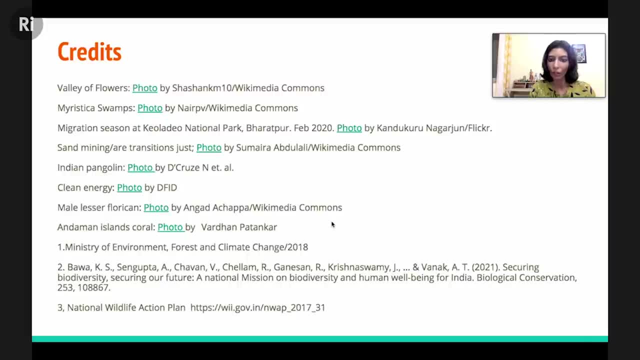 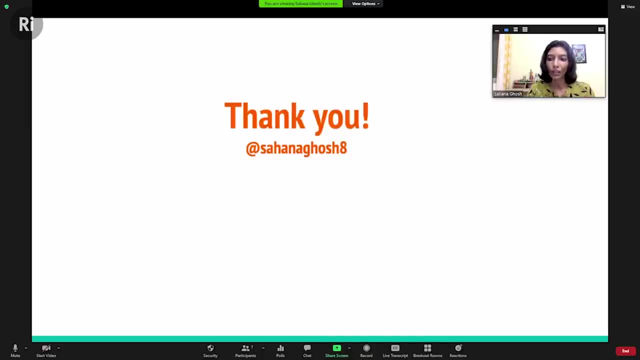 this is what is happening And these are the actions that we could take. So- and you know, I've taken a whole lot of photographs and these are the credits, these are the documents that, if you want to go back to, you can sort of look at the data from there. Thank you all for having 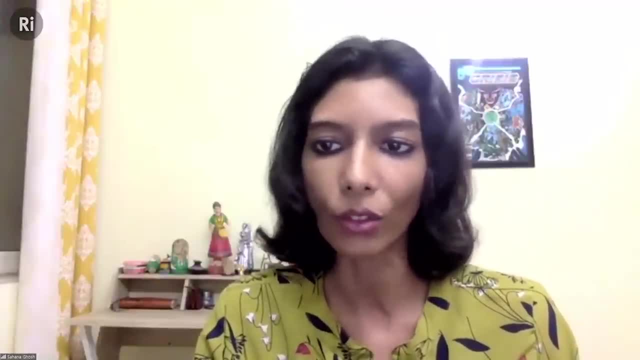 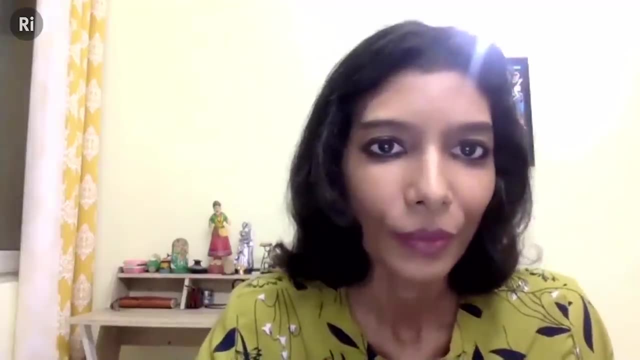 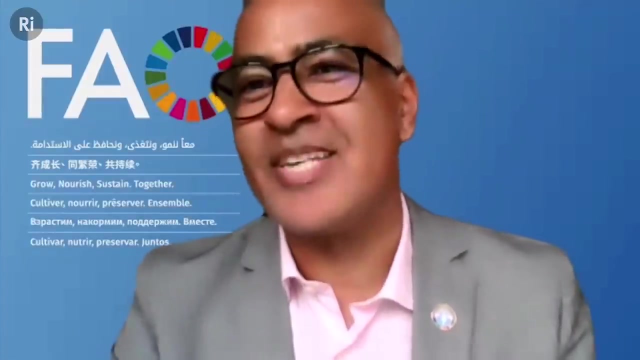 me here And I'm welcome to feedback and questions. And you know I welcome you to India if you ever come here. Thank you so much. Thank you very much, Sahana. That's really very helpful. I'll pick up again just a couple of things that you mentioned, particularly the 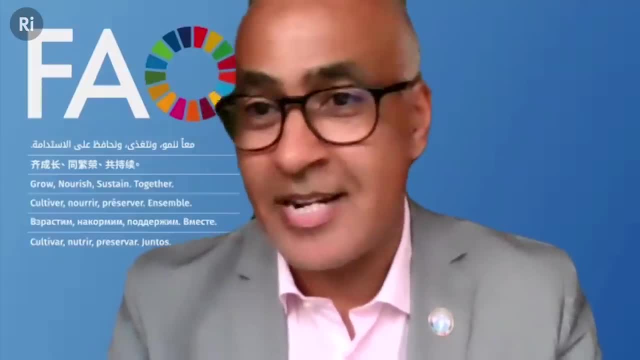 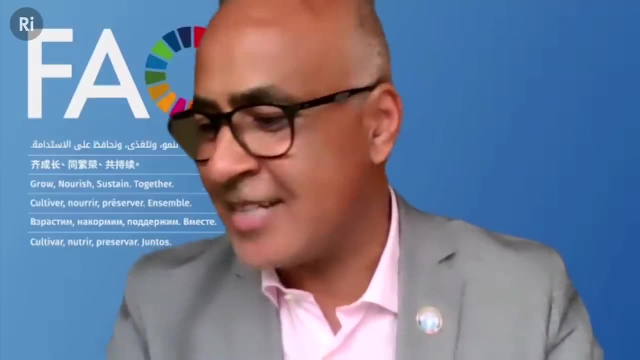 integration aspects And I think, as a journalist, that's really extremely important because it reflects the world we live in. we can't treat things in isolation. you know everything is interconnected And, as you said, you have to look at biodiversity, climate change, ecosystem services. 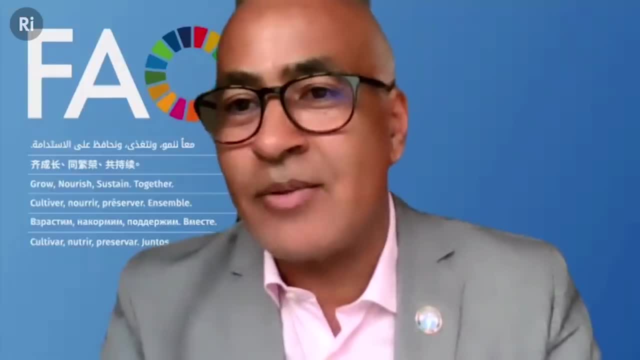 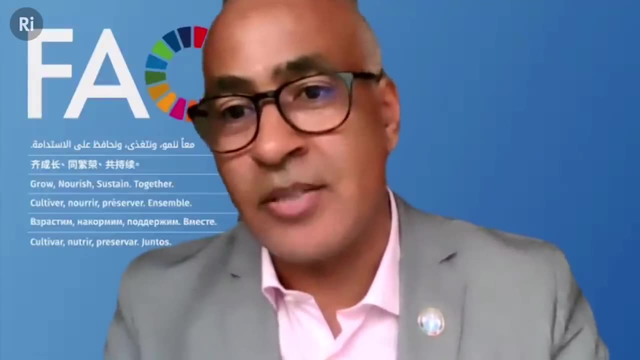 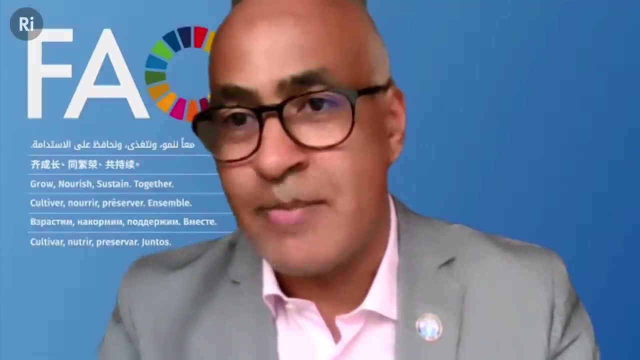 and others in an integrated way, really, because- and that also highlights the importance of looking at synergies between these and also the trade-offs, So it's really critical. And the second point I wanted to highlight, and thank you for mentioning that- is the role of women and youth in the 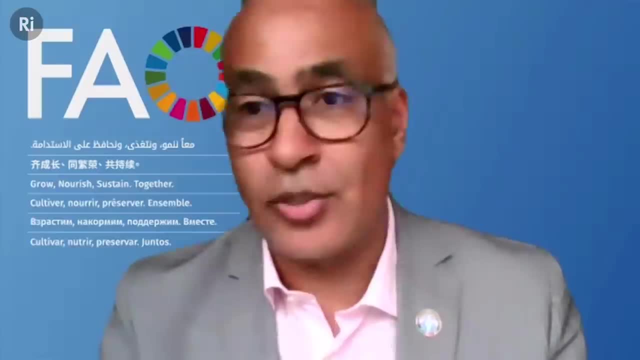 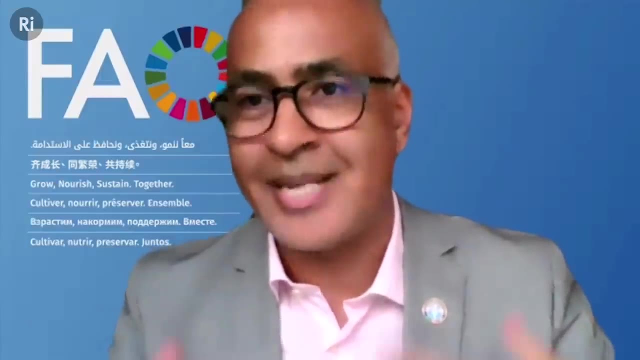 environment in decision-making. That's something that we're not doing enough of really, particularly the involvement of decision-making. I think when we talk about gender, it's not just a talk about gender, but actually to involve marginalised women and communities in projects. 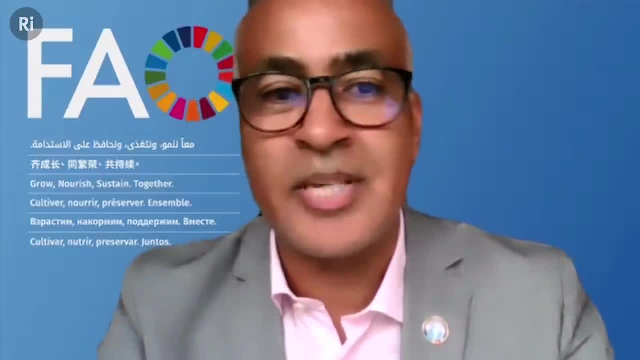 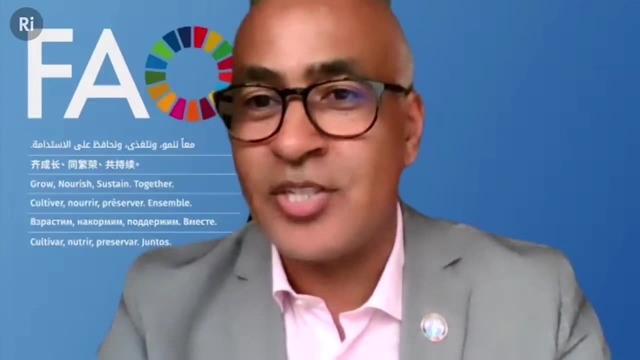 in decision-making so that we can make the change we want. So thank you very much for that. Let me now move to another area, particularly areas to do with communication and communication with kids. So it's not very easy really to explain these things, particularly to. 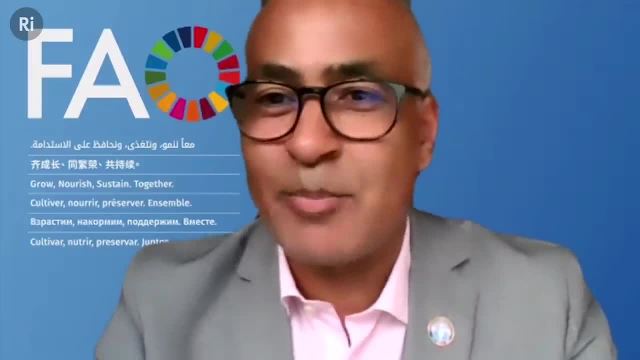 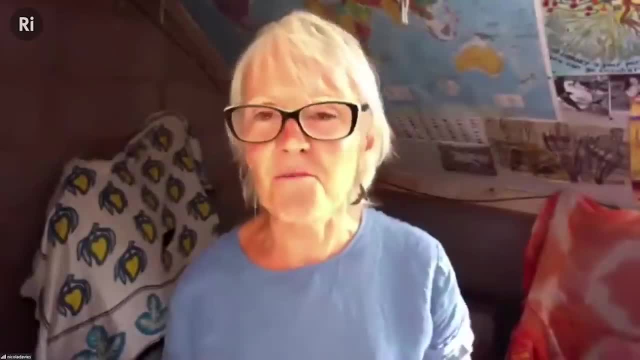 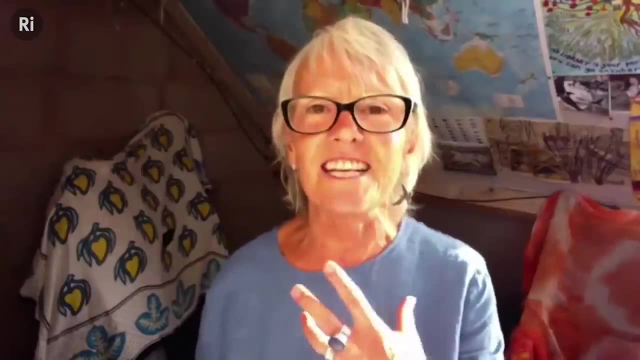 who will tell us all about it? Nicola, over to you. Thank you so much. I'm absolutely delighted to be part of this panel this evening. Lovely to hear Tilly talking about planting, the importance of planting connecting with the natural world. 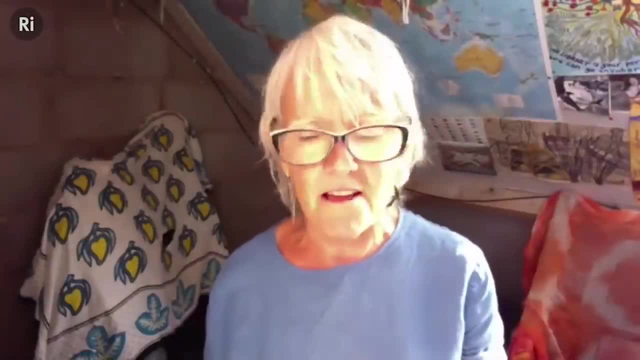 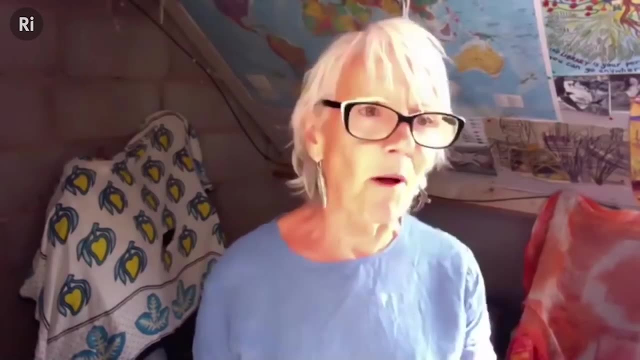 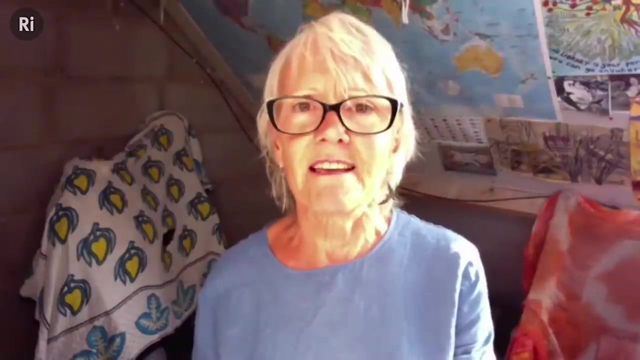 and to hear Sahana talking about conflicts with wildlife, wildlife corridors. These are all things that I've written about, sometimes for the very youngest children. I've written about microbiology, I've written about DNA and I've written about biodiversity. Now, why write about those things? 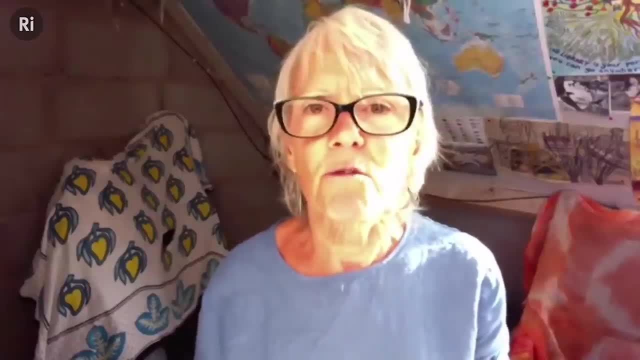 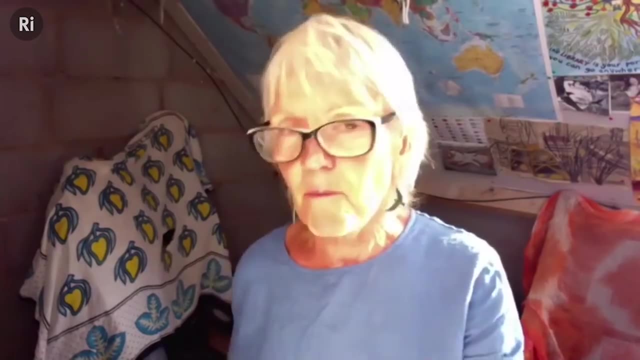 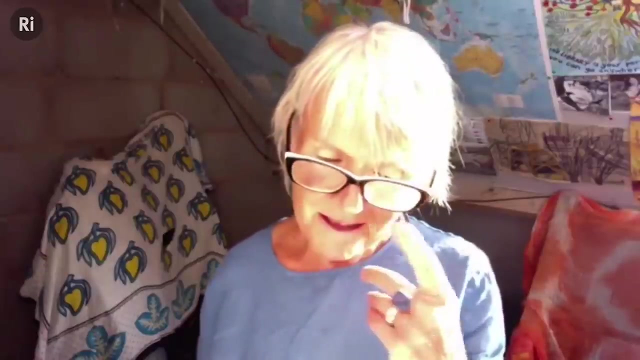 Well, the first thing is: if we're going to change, change has to come at all levels. Everybody has to understand it. And the second thing is: well, there are two more things actually. One is that kids have pester power, enormous pester power. 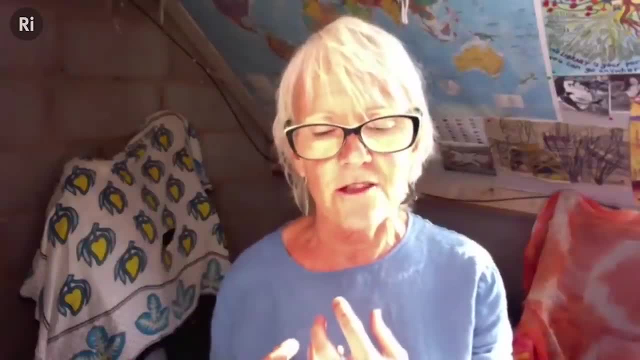 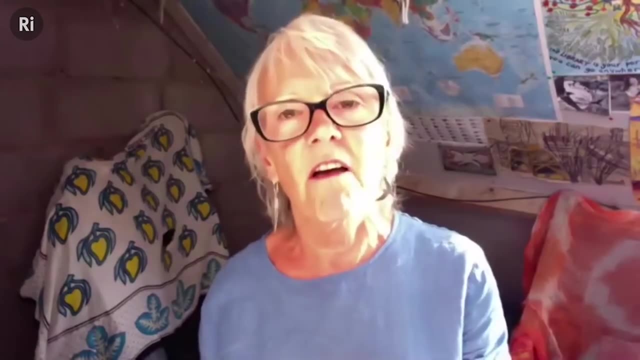 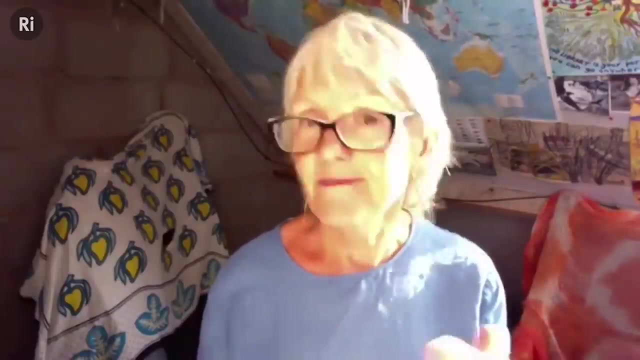 If children understand something, they can push the adults to change, And the other thing is many adults really, really don't get the basics of the science that they need to understand to grasp climate change and biodiversity, For instance. many adults- Donald Trump, I would call as an example- 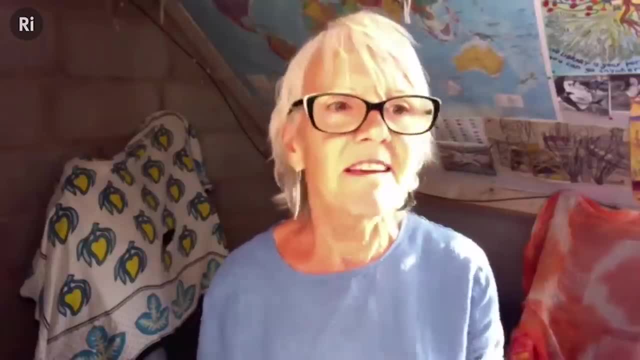 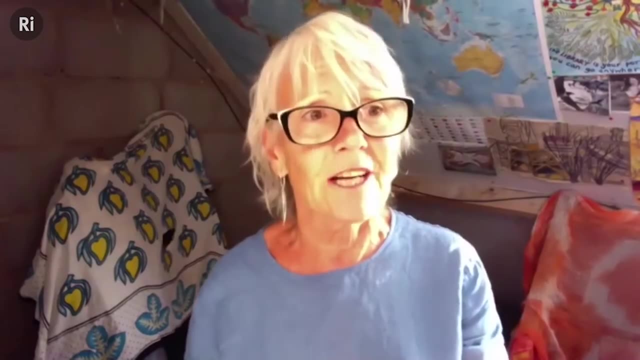 don't understand the difference between climate and weather because they don't understand what averages are. They don't understand statistics. So if you explain these things in a way that the very smallest children can understand, then the adults reading those books to the children. 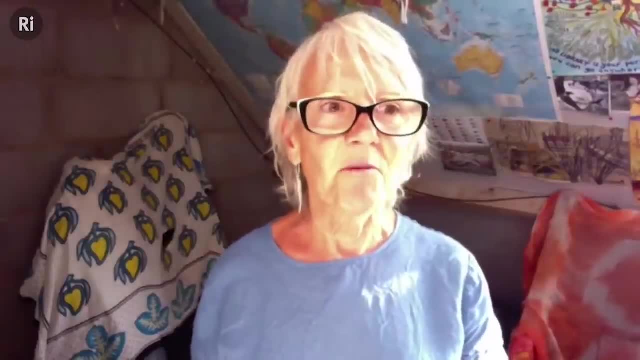 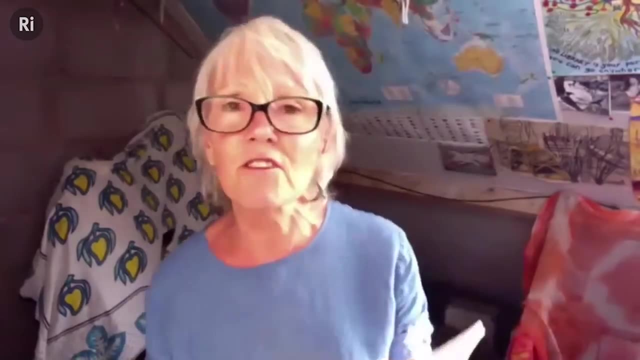 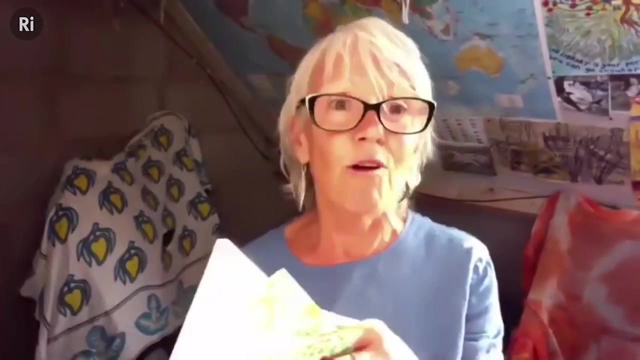 can also quietly say to themselves: oh okay, well, I really get that now. So rather than talk about how this is done in theory, I'm just going to read you a picture book. Now you probably all think you're way past picture books. Let me tell you you're absolutely not. 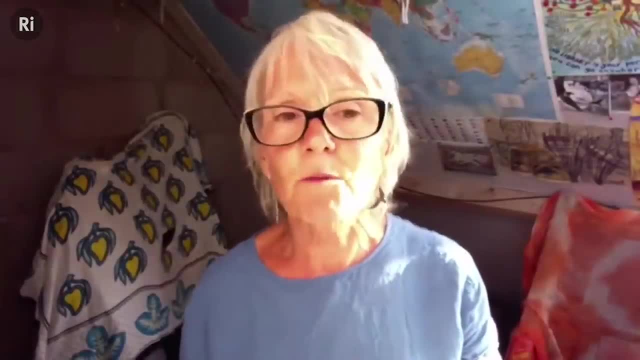 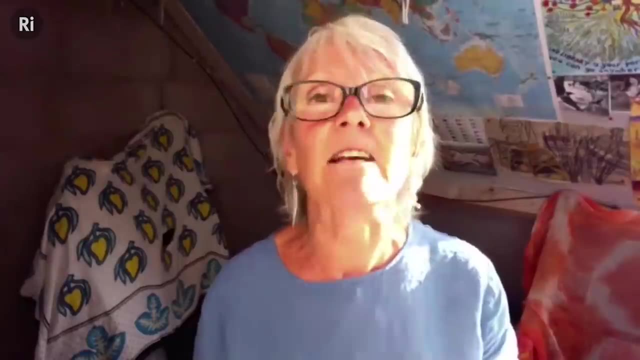 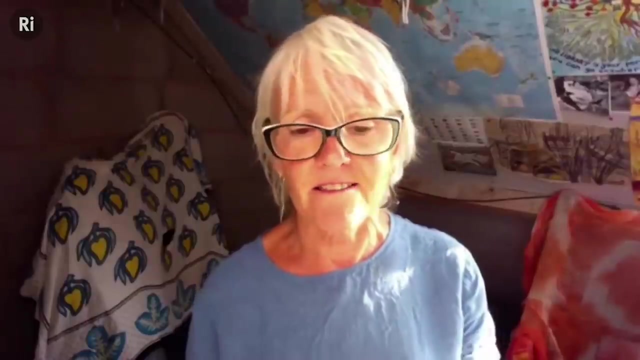 The picture books that I write. I like to impart information. I want my audience to read something, But, most importantly, I want them to feel something, because they are not going to take any action at all unless they feel something about the facts that I've imparted. 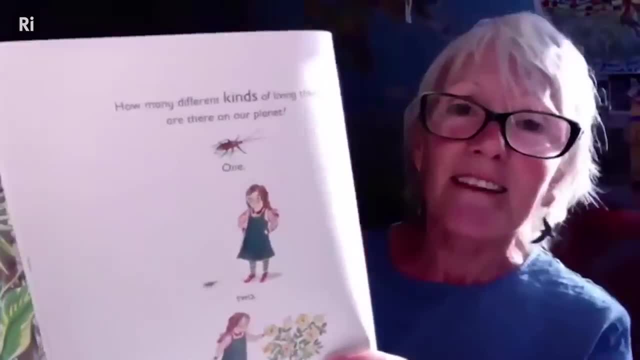 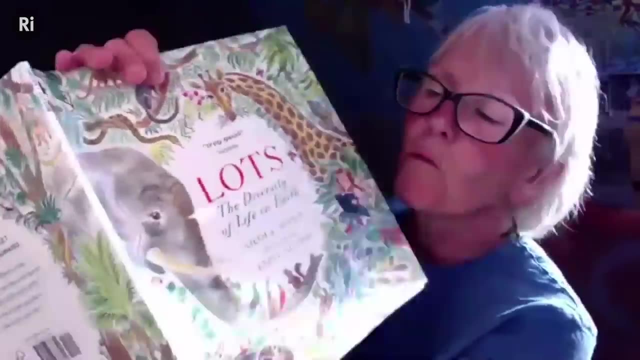 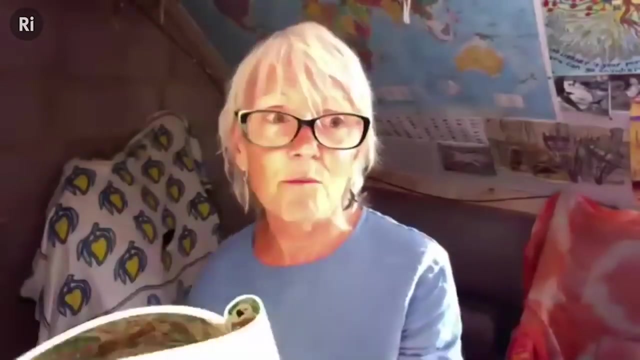 So I'm just going to hold the pages up and read this book to you. So it begins. it's called Lots. by the way, I'll show you the cover. I can't claim the illustrations. Wonderful illustrator Emily Sutton. There's a lot to be said about the role of illustration and visual imagery in communicating about science. 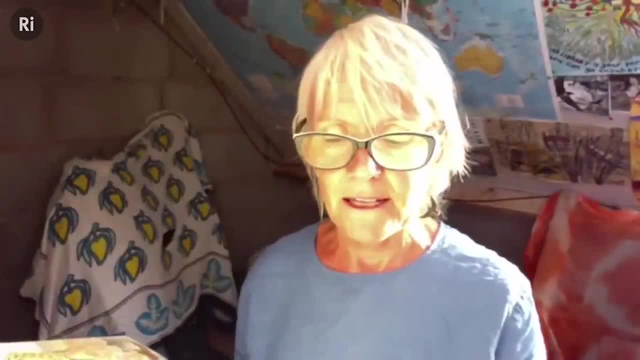 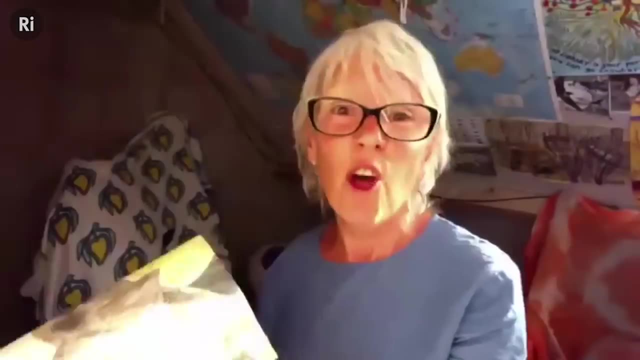 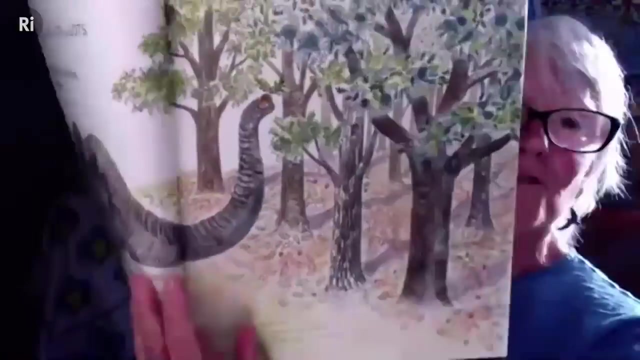 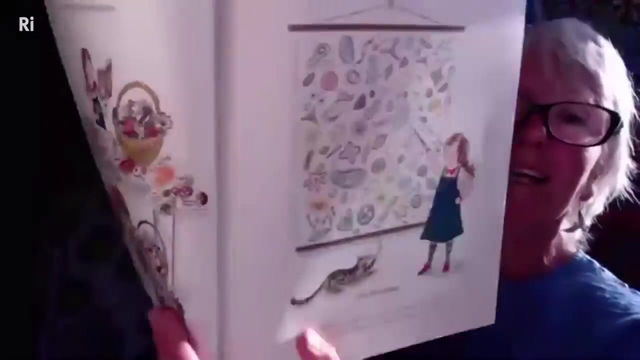 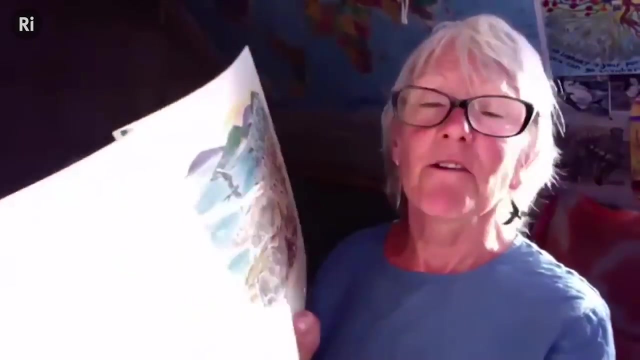 How many different kinds of living things are there on our planet? One, Two, Three, Lots. There are lots and lots and lots, from big things like elephants and oak trees to little things like mushrooms and microbes. Everywhere you look, there are living things In deserts. 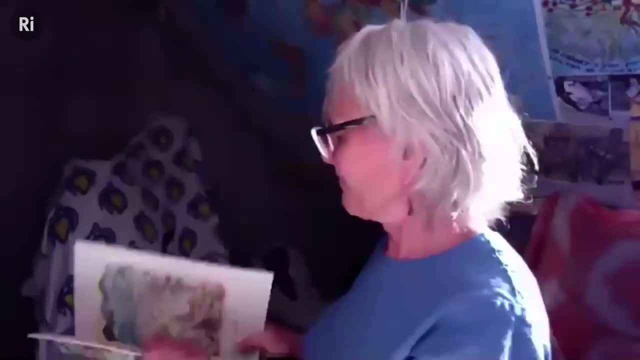 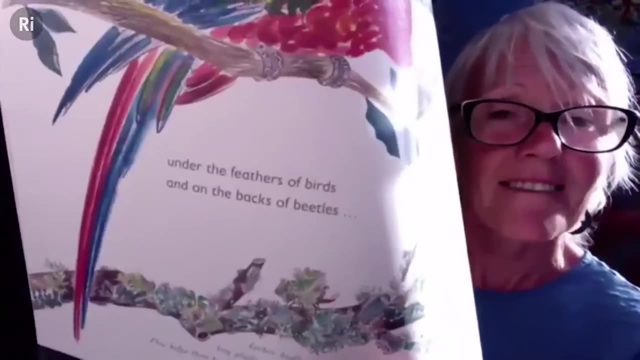 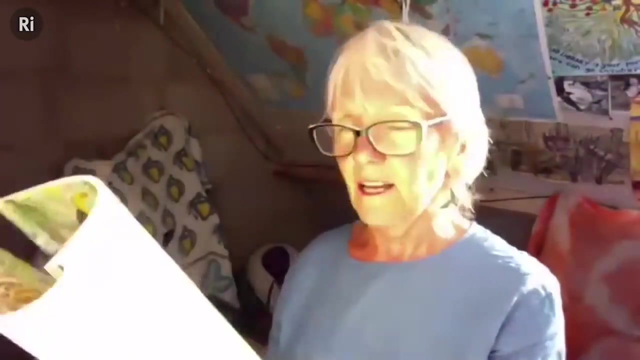 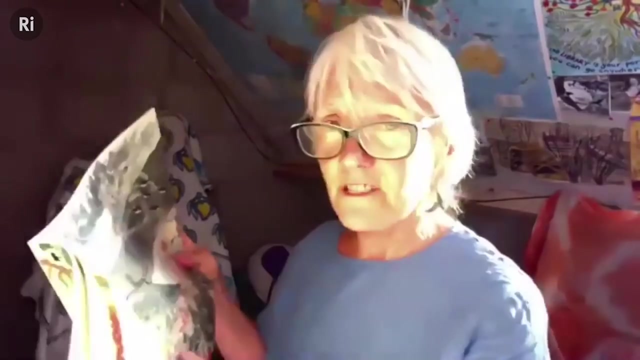 On islands Far out to sea, Under the feathers of birds and on the backs of beetles, Even in places where you would think nothing could live at all, like boiling volcanic pools. Counting how many kinds there are can be difficult, because some places are very hard. 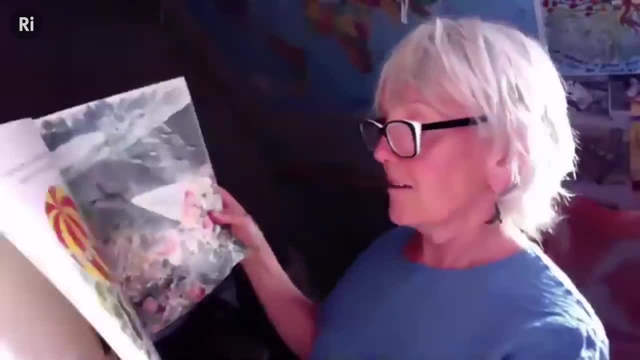 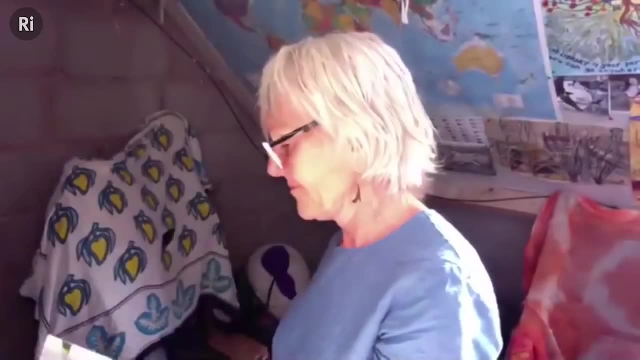 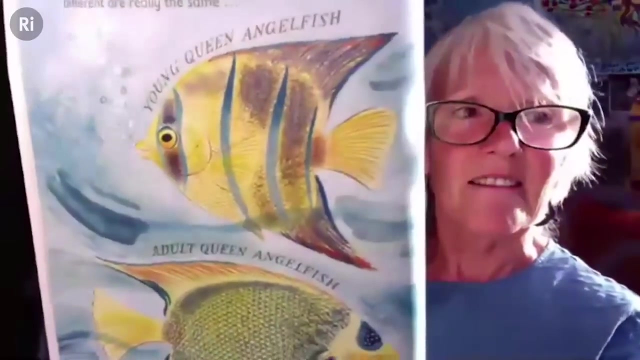 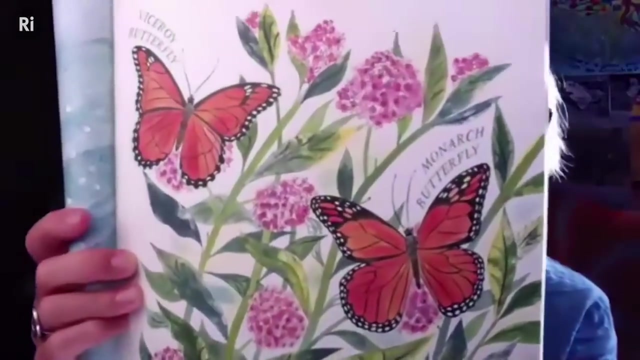 Like the tops of trees in the jungle Or the very bottom of the coldest seas. It can also be difficult because sometimes things that look different are really the same And sometimes things that are different look the same. But mainly it's difficult because there are just as many things that are different. 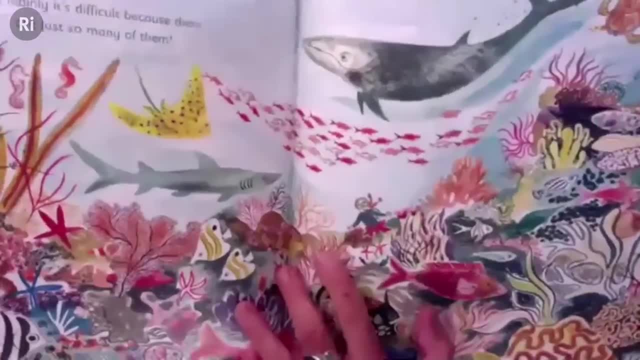 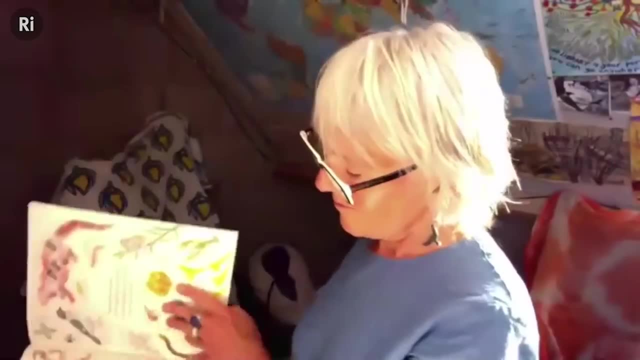 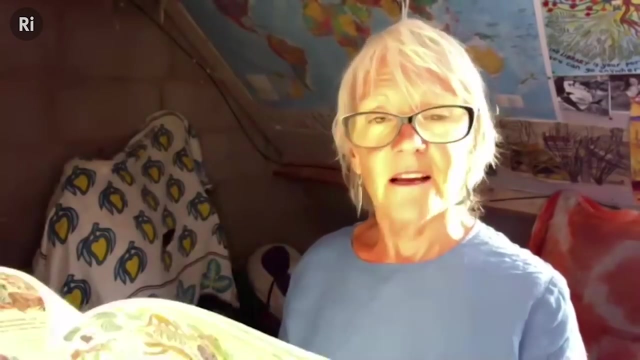 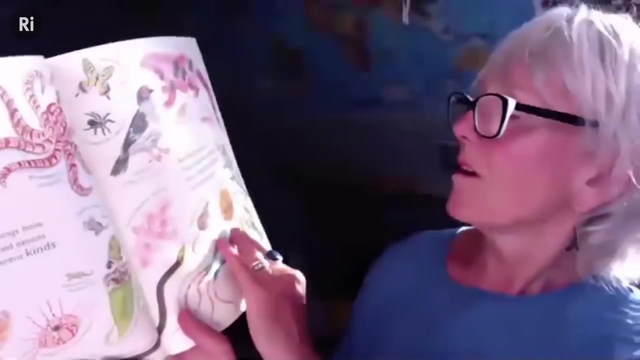 And a lot of them are very difficult because there are just so very many of them. So far, human beings have found and counted almost 2 million kinds of living things, but that's only the start. There could be many millions more. 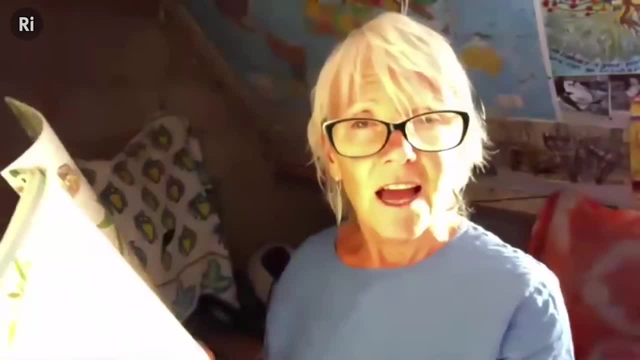 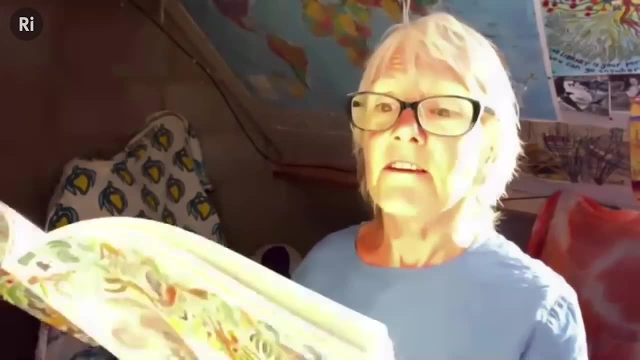 Thousands of new kinds are found every year, And the more we find, the more we learn about how living things depend on each other for food, for places to live and ways to grow. I won't go through all those examples really, but there's lots of little examples there. 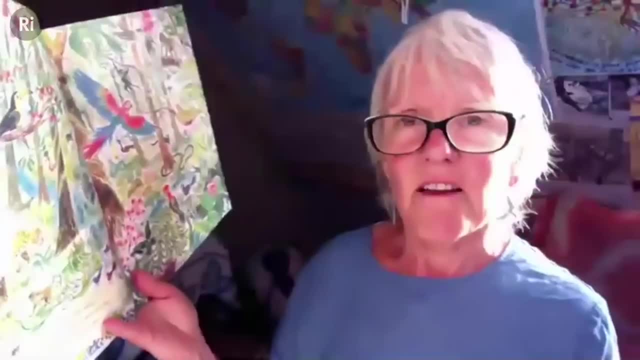 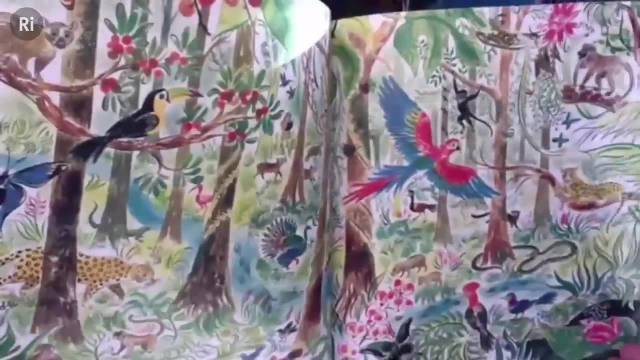 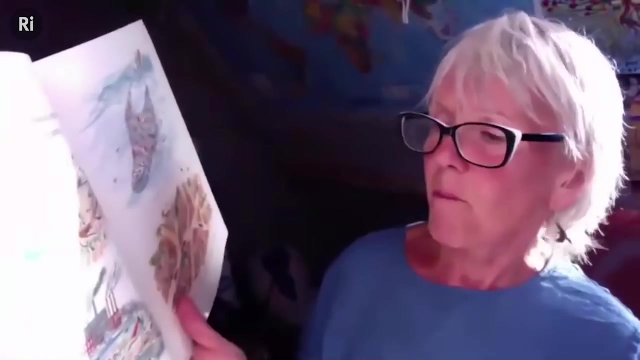 of how that works. We have learned that every kind of living thing is part of a big, beautiful, complicated pattern. The trouble is: all over the world. human beings are destroying bits of the pattern, poisoning the air, rivers and oceans. 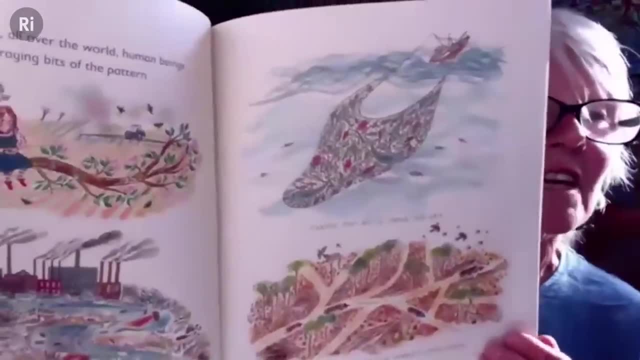 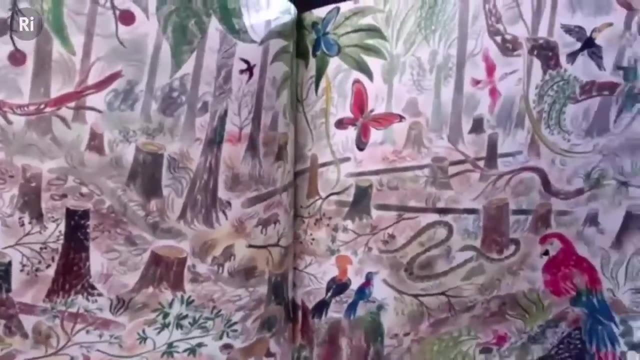 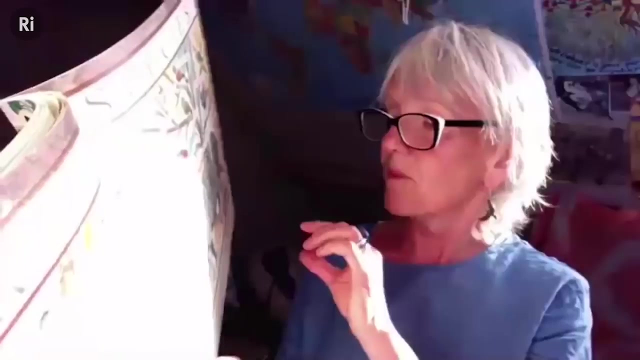 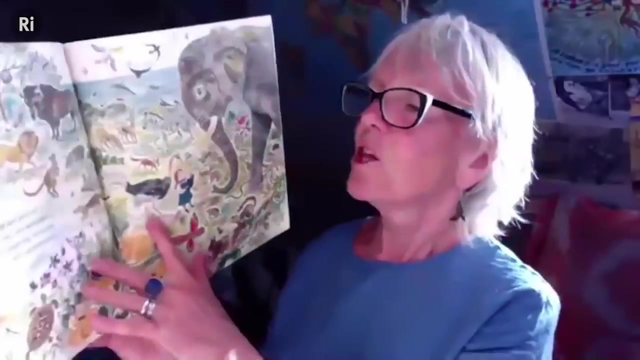 taking too much from the sea, building roads that cut forests to pieces so that animals and plants disappear. Many kinds of living things have already been lost. Perhaps some have disappeared before we even found them. Human beings are part of the pattern too. 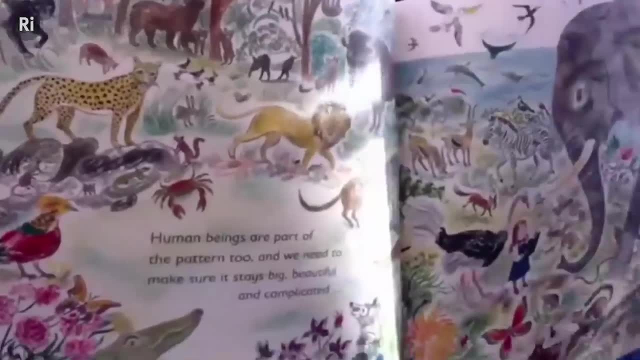 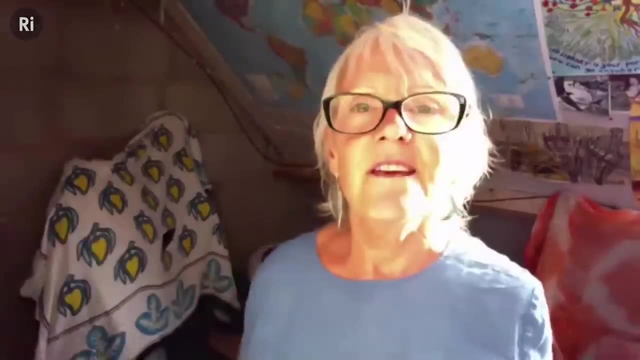 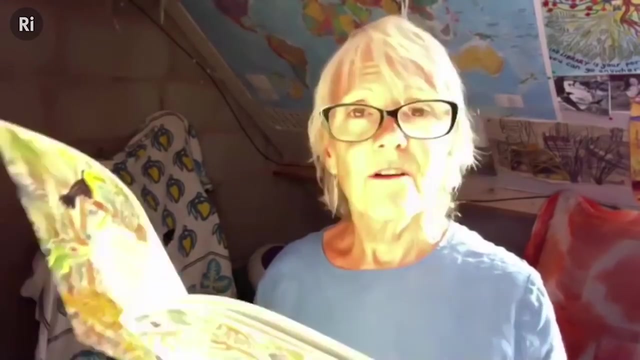 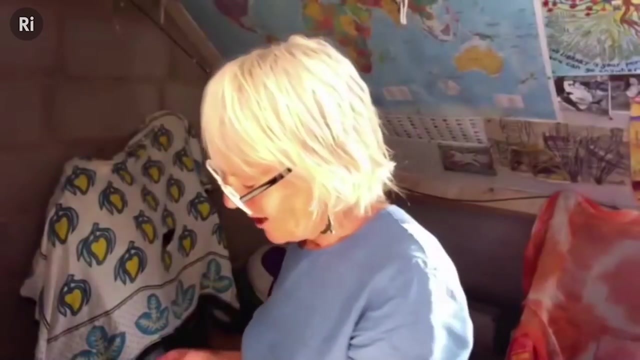 And we need to make sure it stays big, beautiful and complicated, because we could not live on an earth where we had counted down instead of up from lots to one. So we need to stop that Now. the one thing I would say about this book: 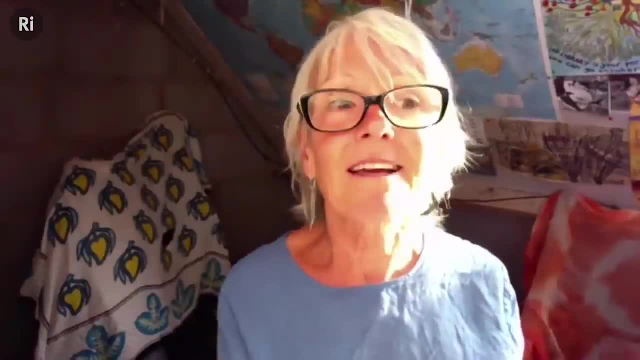 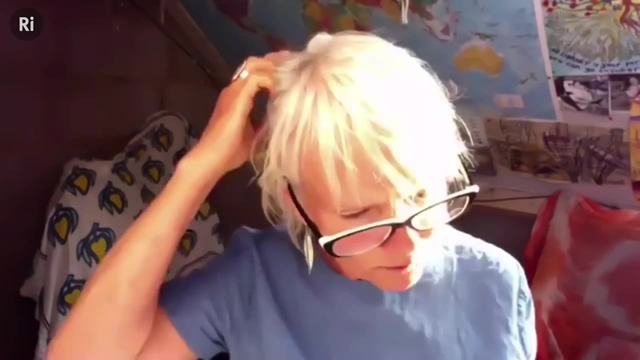 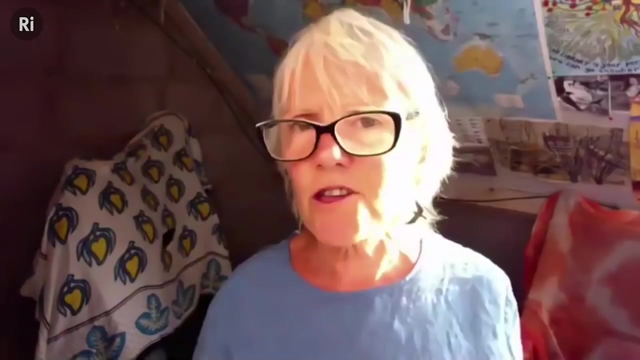 is that those of you who are biologists out there, you will recognize the biological information that's gone into that book, And all of the statements in there are, of course, backed up by a lot of complicated factual information and good science, and all the illustrations are too. 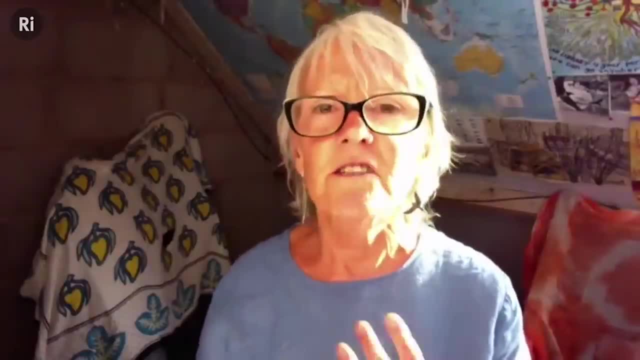 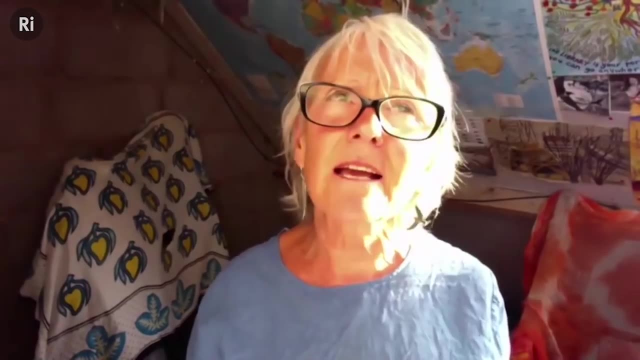 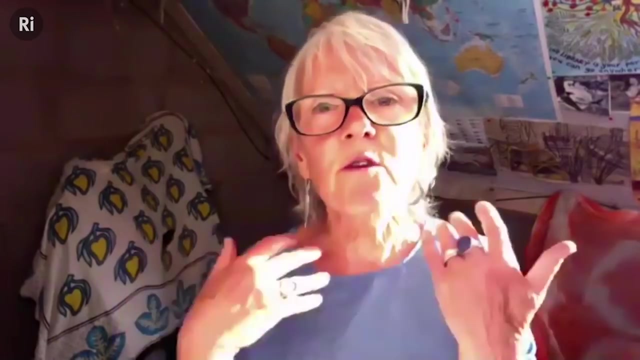 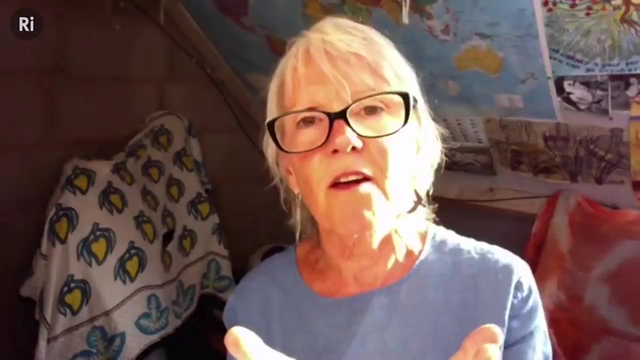 but they're distilled down into simple statements that are intelligible to a woman wide audience. and the other thing to say about picture books is: unlike a film or an animation or a theatre performance or a television program, picture books are read multiple times and they are read at the speed dictated by the reader. is the person who completes the circuit of the. 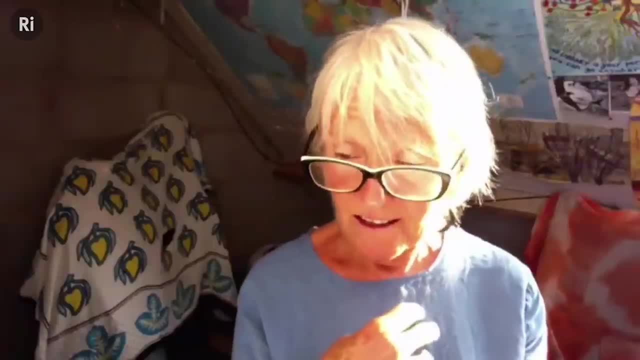 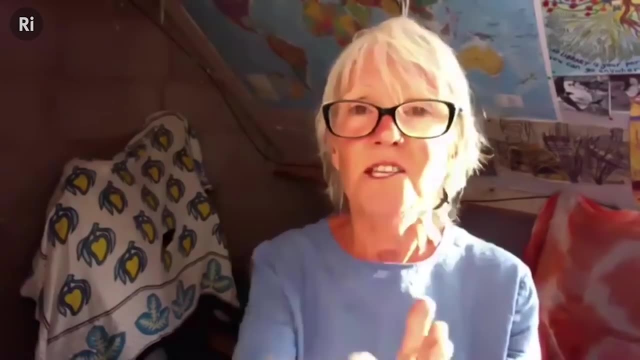 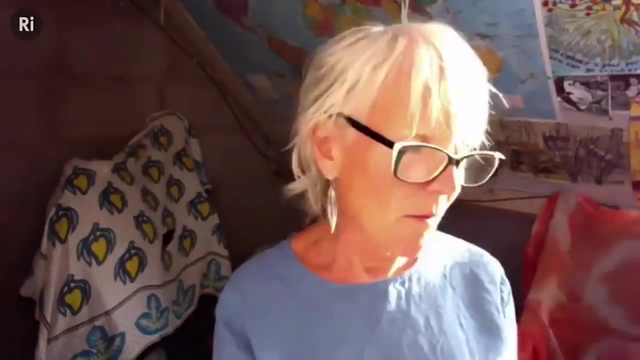 illustration, the words and that circuit is is as individual and unique as that reader. so the message is delivered in a way that is individual and unique and can sink in over a long time and therefore have a big emotional punch, and this book has been translated into multiple languages. 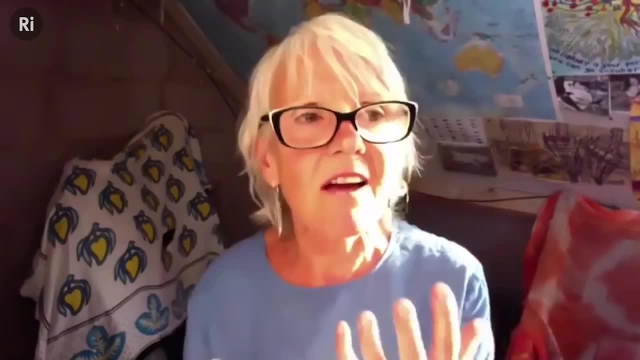 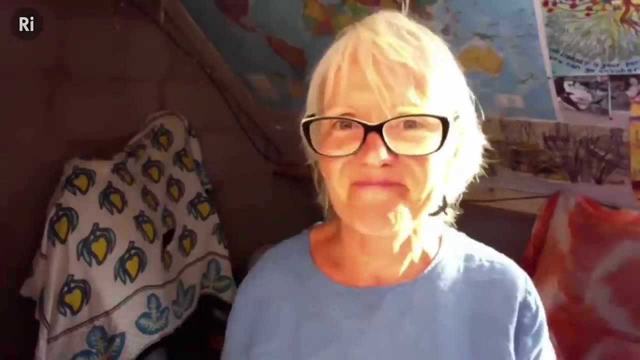 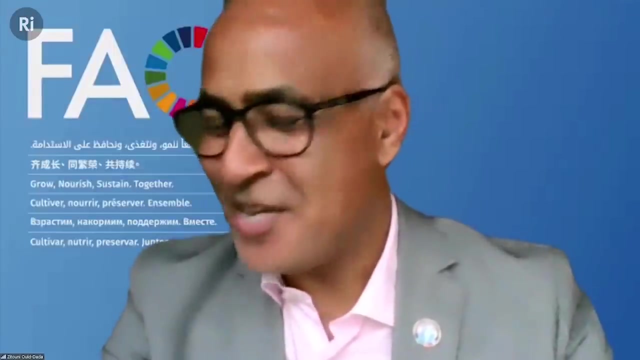 around the world, so I hope that its message of what diversity is and how everything is connected um is going to spread. thank you very much, Nicola, um the way you told that story, um you know, I found it so captive and interesting that I forgot to time you. 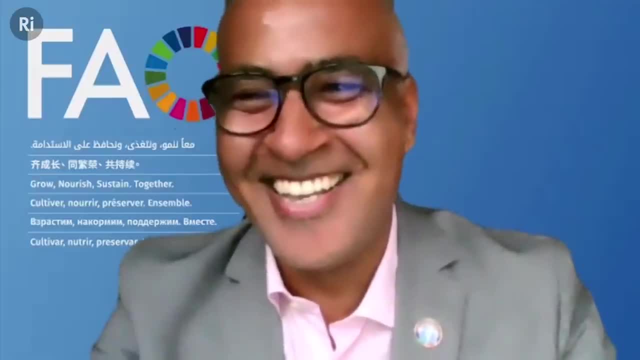 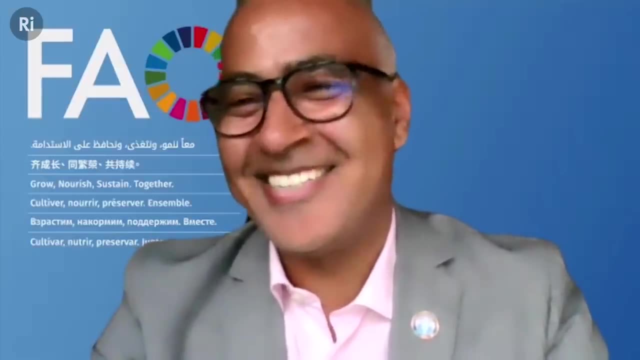 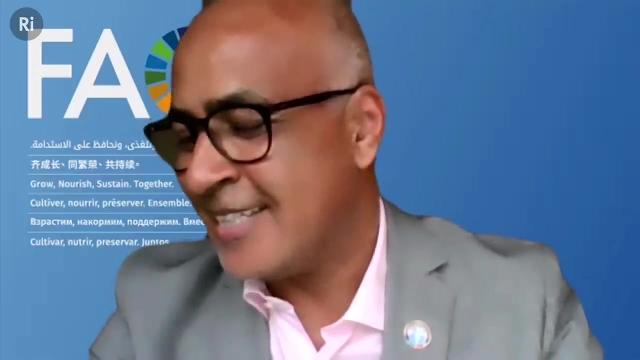 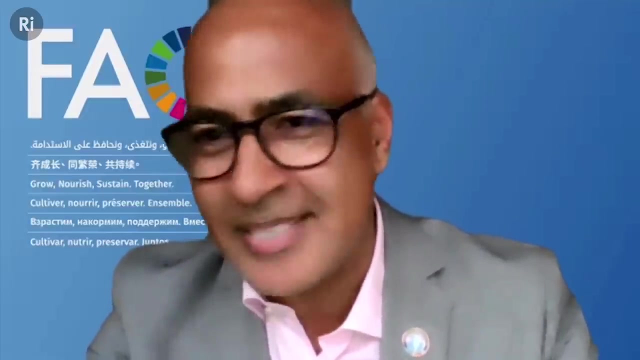 I came in under. I timed it earlier because I knew you know I I knew I could definitely say done quickly now. you definitely stayed below the 10 minutes, but thank you very much. that's really very powerful and I like your um point about the simple statements, and that's exactly what we need: something simple that everyone can understand. 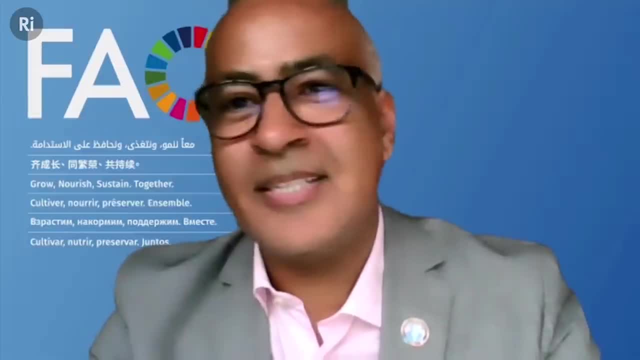 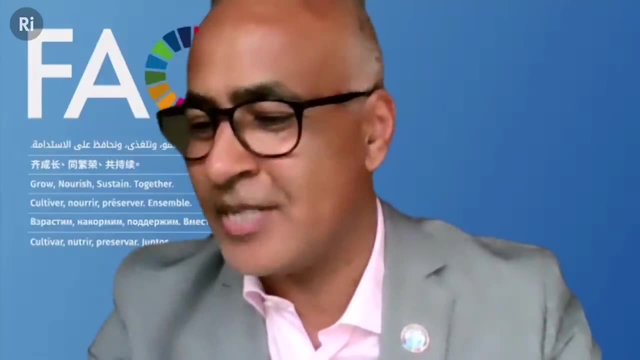 it's emotional silver bullets. that's what you need. you need something that goes not here. it goes here. yes, and that's what I wanted to pick up on on the point you mentioned earlier. it's so powerful. you said you know reading picture books. you want the kids to feel like they're in a place where they're. 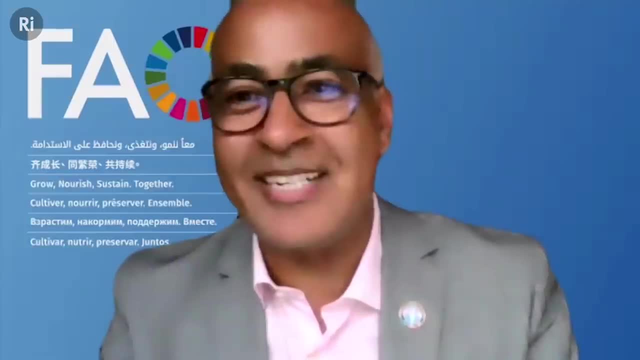 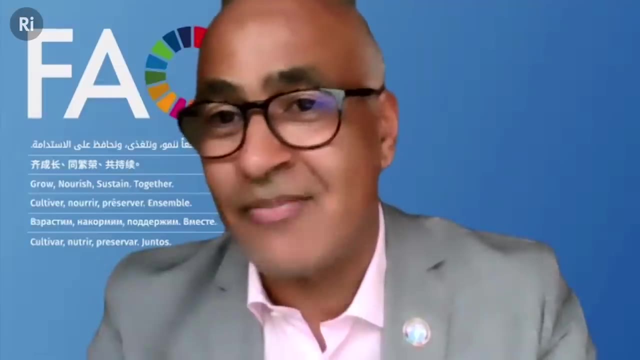 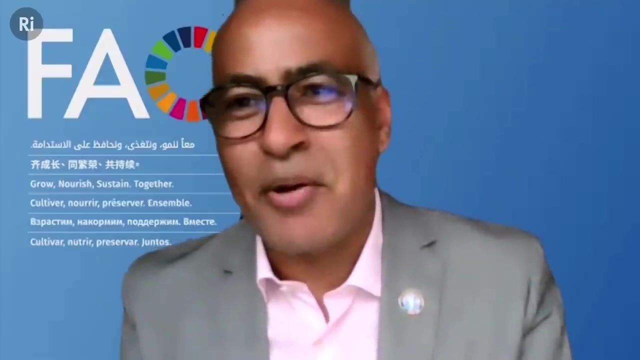 able to feel something so they can act, and I think that's really the key. and if you look today at what we're facing with regard to climate change and biodiversity loss and environmental degradation in in, in general, people actually don't seem to feel the the problem and what and and how much. 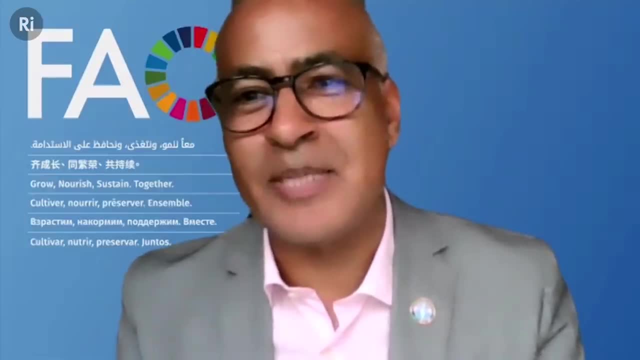 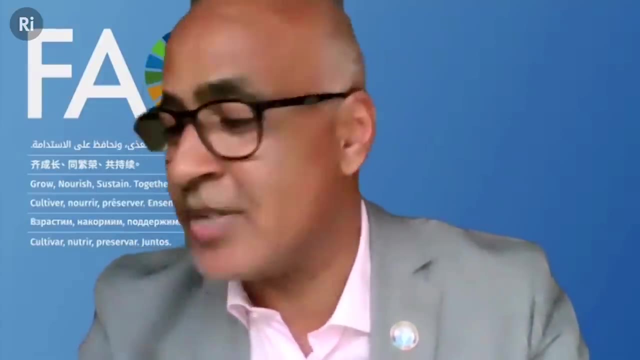 we're hurting the planet and how much we hurt in the environment. so unless you feel that and you feel concerned, of course you you're not going to act. so thank you for that. I mean, the feeling is is really powerful, um one. and I liked also what you said about you. know all these little. 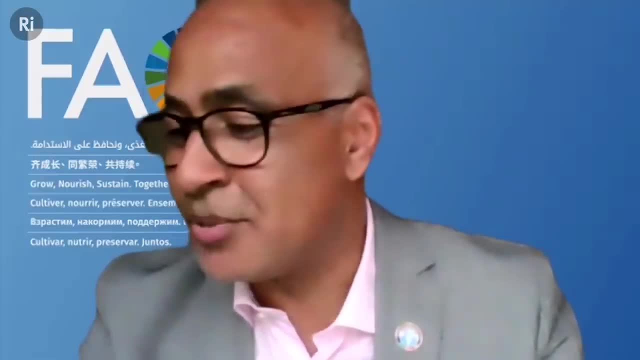 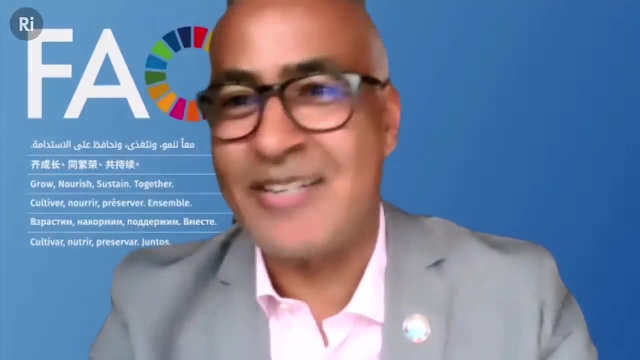 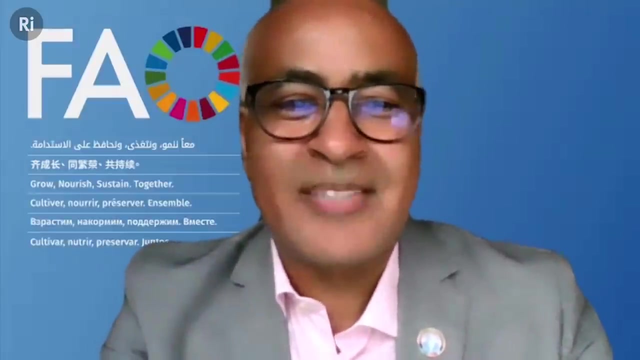 things are part of a big, beautiful and complicated uh pattern. I think that summarizes really very nicely. so thank you very much for that. I mean you highlighted so many key points, but just picked up a couple there. um so let me now move on to our fourth speaker, who's also a children's book writer. 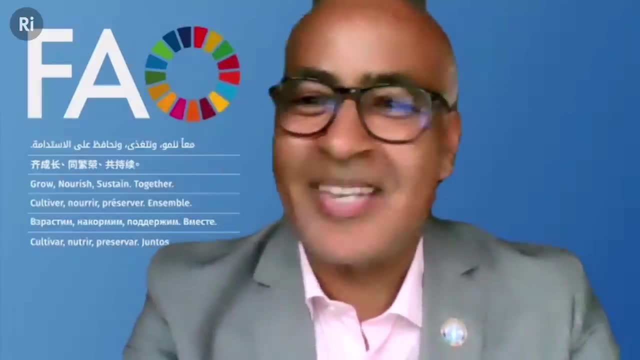 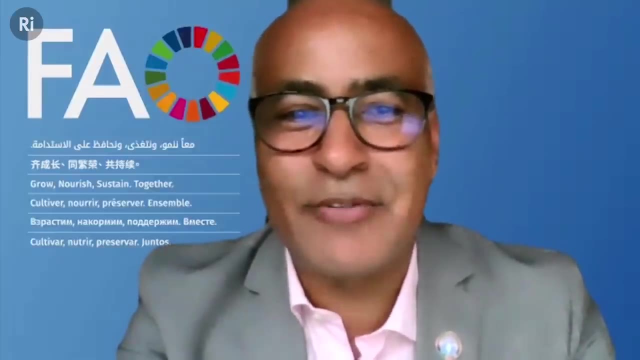 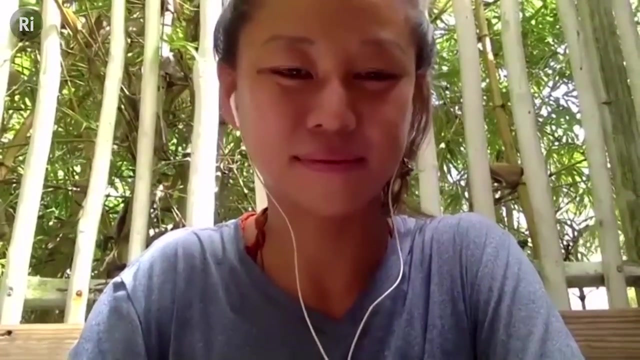 from another part of the world, and I think that's really powerful. and I think that's really powerful. um, and, and see, you know her experience as well. um, so, Angeline, over to you. we lost her. where is she, Angeline, can you hear me? yes, I'm here, can you hear me? 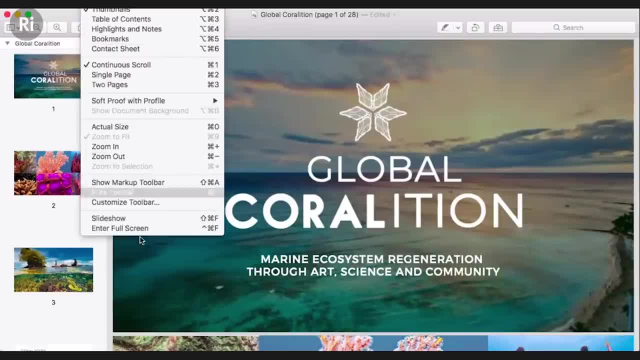 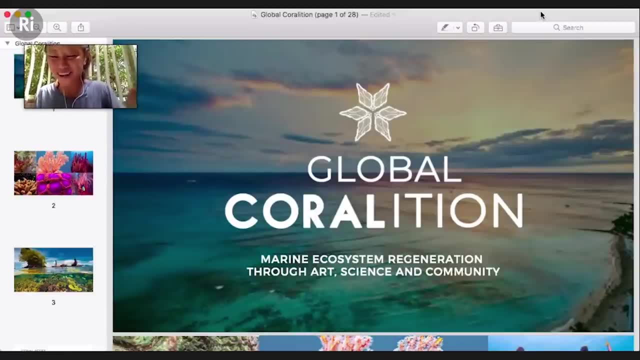 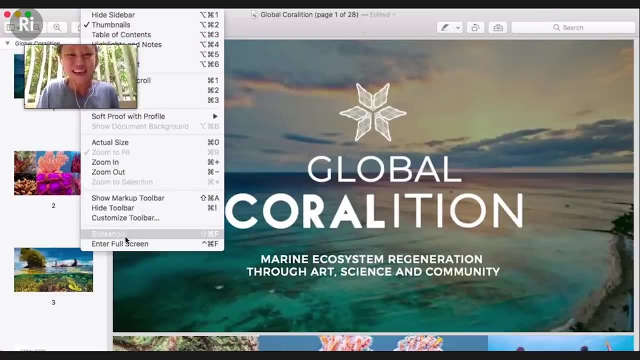 yes, we can. yes, awesome. thank you so much for having me. I am in between a bamboo forest and a busy street in the Dominican Republic, so I apologize for the noise, but I hope you can hear me, and thank you so much for for having me. um, so I am, yes, a co-founder of an organization. 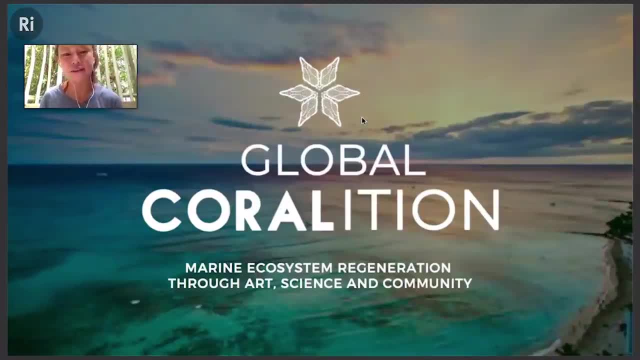 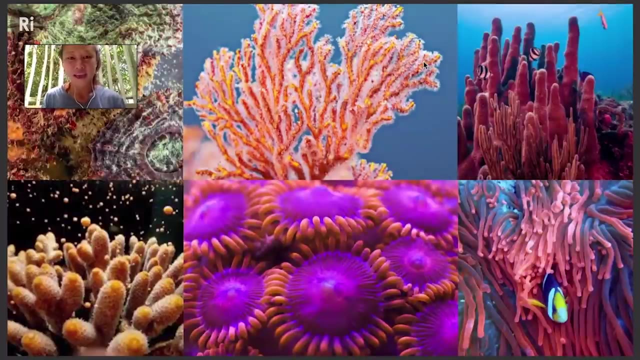 and a non-profit called Global Correlation. we're dedicated to marine ecosystem regeneration using a combination of art, science and community. I'm just going to dive right in. corals are these incredible, beautiful animals made up of tiny polyps, and there's over 6 000 different species of coral. 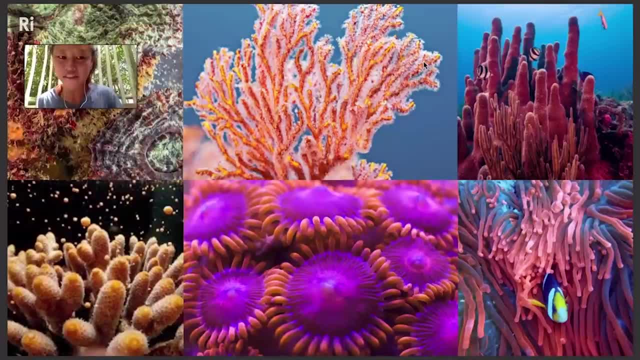 some are soft, some are hard. the picture on the bottom left are corals spawning. they release millions of eggs and sperm all at the same time once a year in, and it's their way of trying to promote further biodiversity and keep their species alive and reproduce together and it 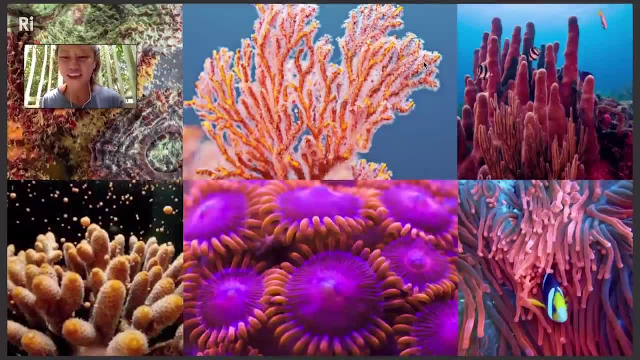 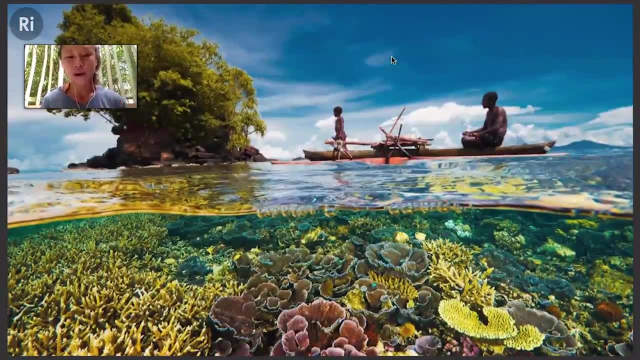 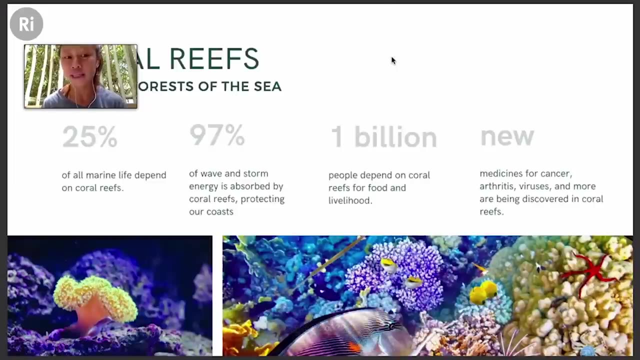 only happens once a year under the full moon. it's a really magical cosmic event and all together, corals- many different species in one area- create a coral reef ecosystem and that becomes home for over 25 percent of all marine life, live and eat within the coral reef. 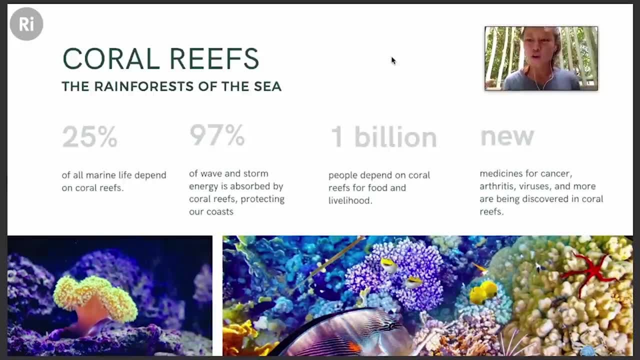 they call them the rainforest of the sea, the, the coral reefs absorb 97 percent of wave and storm energy, which protects their coastlines. they provide food and livelihood to over 1 billion people around the world and because corals can take over the world, they can take over the world. 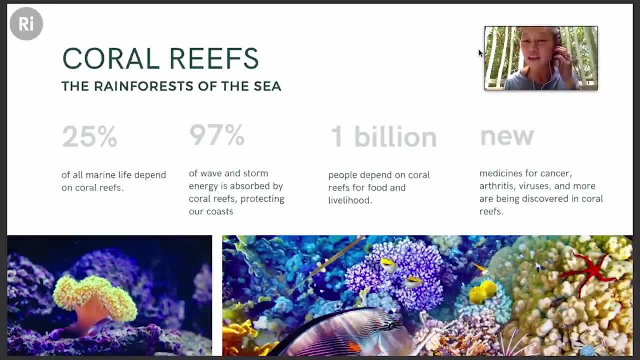 and because corals can take over the world, they can take over the world. and because corals can take over the world, they can take over the world. and because corals can take over the world and bioactive compounds, they've been discovered to be potential new medicine for cancer arthritis. 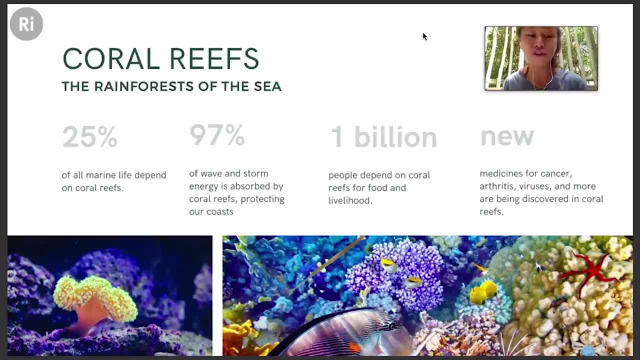 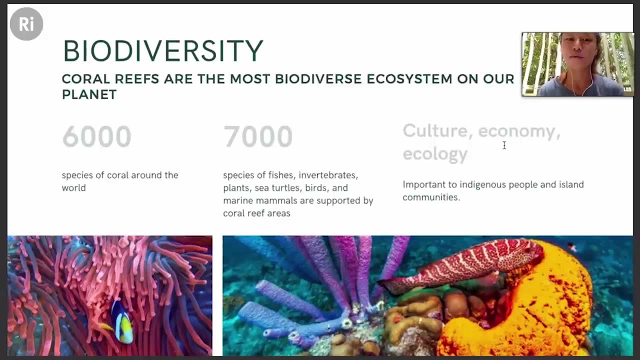 viruses and more. they say we're 300 to 400 times more likely to fight due medicine in the ocean than we are on land. and in terms of biodiversity, they say coral reefs are the most biodiverse ecosystem on our planet, with over 6 000 different species of coral supporting 7 000 different. 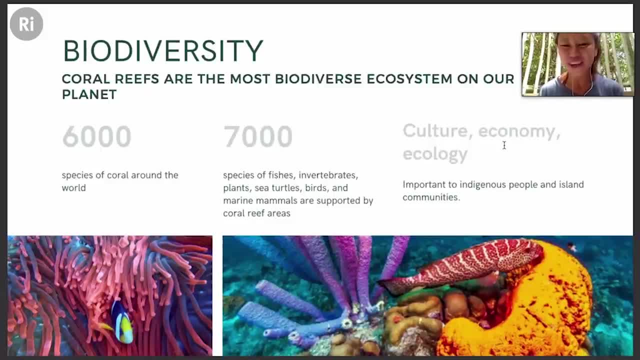 species of fish, invertebrates, plants, sea turtles, birds and our planet and so on and so forth. so you can Epitome to the seaf. VI: marine water misinforms, leaving breathless animals and marine mammals um. they are important culturally, economically, anowo ecologically. 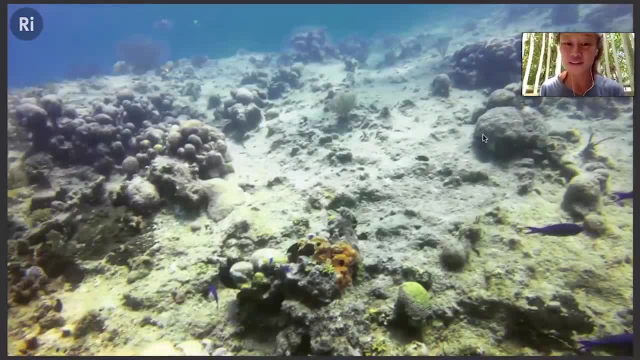 to Indigenous people and island communities all around the world, and so it's so heartbreaking nowadays to see what the reef looks like now. this is the reef here in the Dominican Republic, where we have less than 10 percent of our reef left. most of it is covered in algae. all the fish have been. 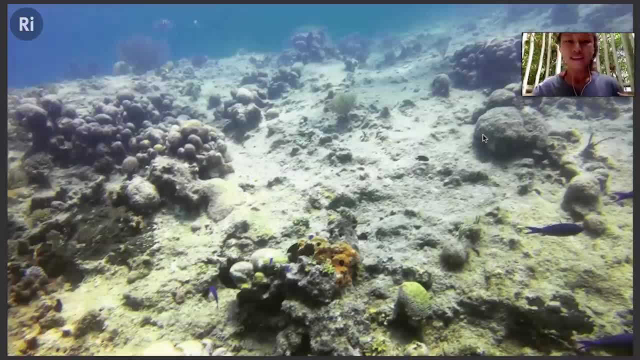 this loss of biodiversity? it's because, as the as the as global warming causes sea temperatures to rise, it causes the little algaes that live in the corals to leave, which caused the corals to bleach and they eventually die as the temperatures keep rising and rising also as co2 gets emitted into the atmosphere. 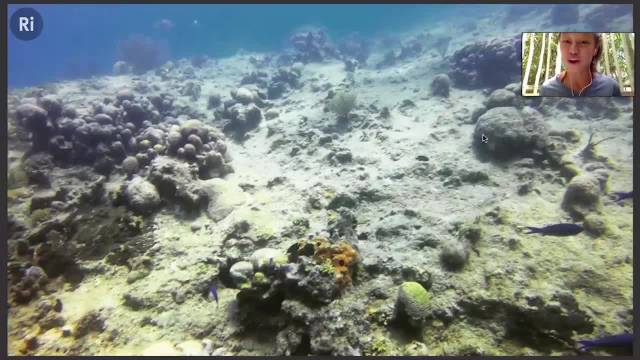 that co2, over half of it, gets absorbed into our oceans and that changes the pH chemistry of the ocean, which has reduced calcium carbonate in the water which the corals used to build their skeletons, so that, combined with local pollution and overfishing, they say the fish eat the algae, so the herbivores are. 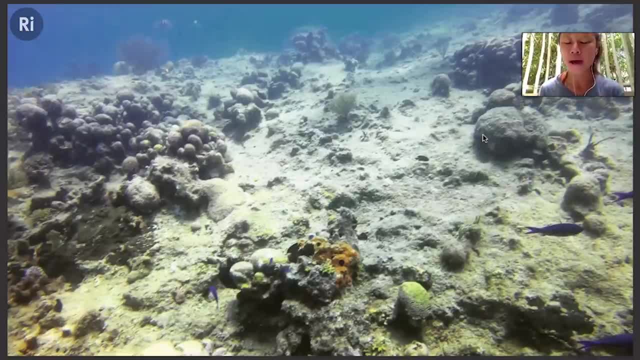 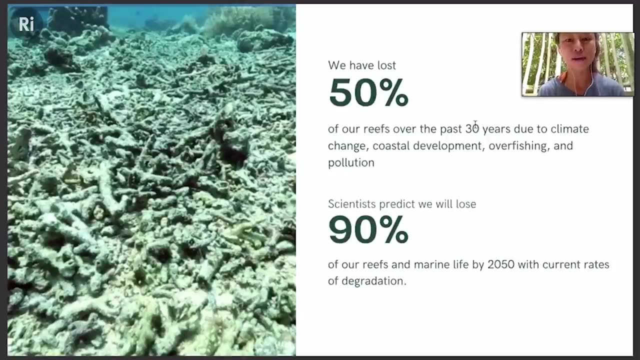 really important in the ecosystem and they keep the algae in balance and when you take them out of the the reef, you get 80% to 100% coral coverage of algae which suffocate the corals. so it's a crazy situation we're in because we've lost half of our coral. 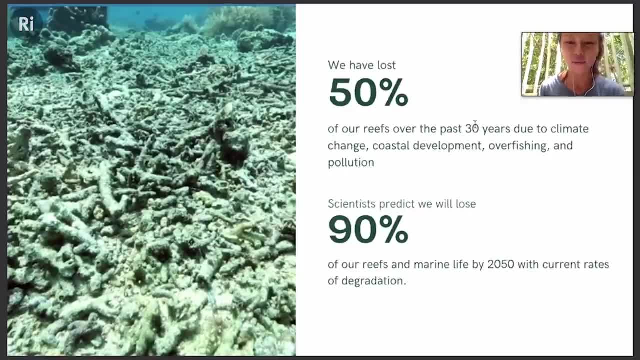 reefs in the last 30 years and scientists predict we will lose 90% of our reefs and marine life by 2050 at the current rates. a recent exciting article came out where scientists studied the recovery rates of marine ecosystems and they actually believe we can rebuild our marine life by 2050 because they recover. 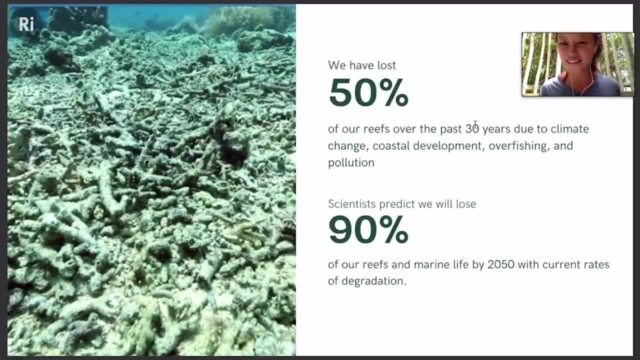 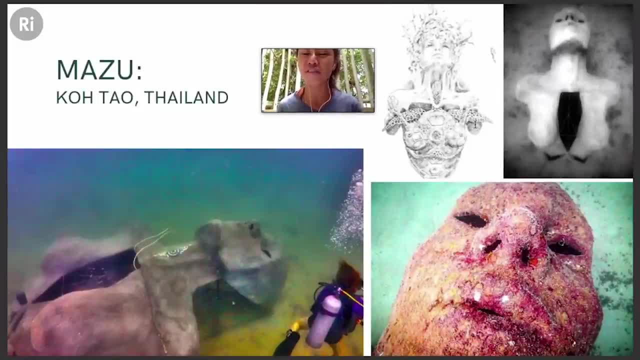 very quickly if the right interventions are taking place. and so me. I'm an artist, my partner- we're artists- and we actually fell in love with the reef in Thailand and we were watching it dying before our eyes and we just thought: what can we do about this? and we built our first sculpture, her. 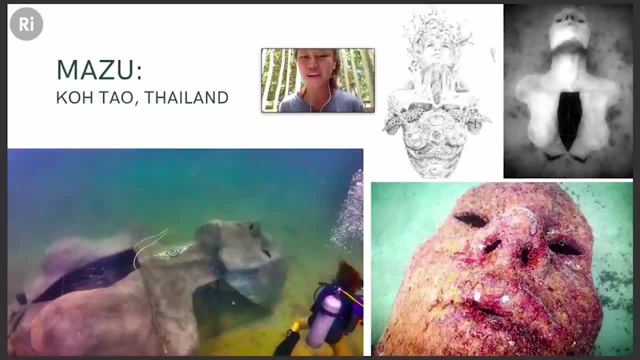 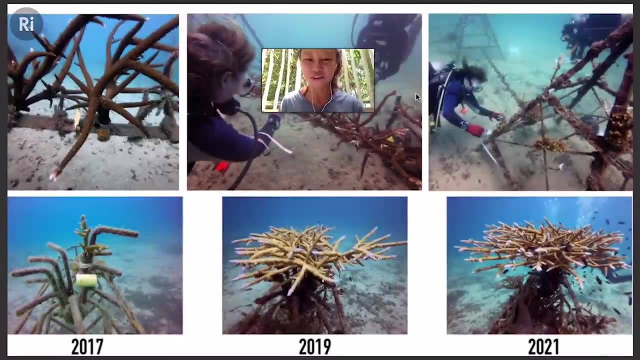 name is mazu. it was inspired from a drawing and we deployed it in the ocean and she be within four months. she was covered in Crestus coralene algae and we gifted it to a local dive community in Thailand and they built 30, six pyramids around the sculpture and started granted coral all over it. it's 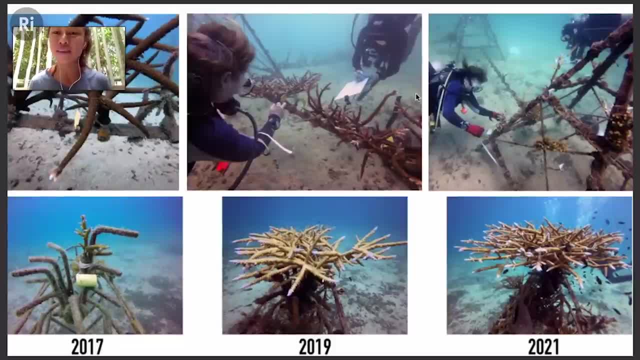 part of a bomber or artificial maybe site that people their and learn from and they learn how to directly with them, and they created their own kind of restoration dive project and business and in Thailand- and if it's really beautiful to say that is at this point we began learning everything that we. 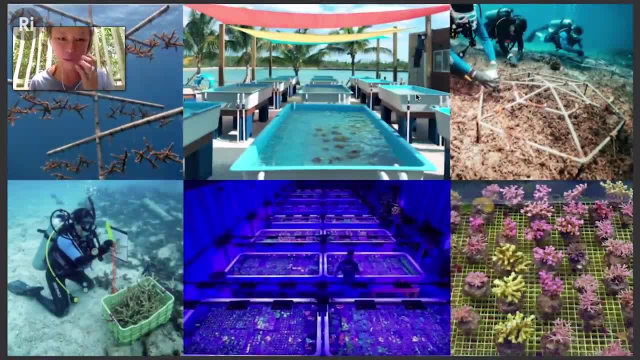 care about rocky on coral and all the different techniques in ways that people- People are doing it around the world. You can grow them on land. You can grow them in the water. People have discovered you can grow much faster on land using techniques of cutting coral called microfragmentation. 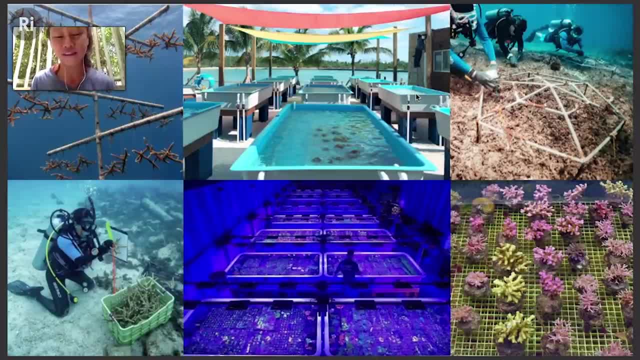 When you slice it into tiny pieces, they grow 25 to 50 times faster. You grow them in tanks, on land. You can feed them, You make the water cleaner, You can talk to them, clean them, sing to them And they eventually grow over this ceramic plug. 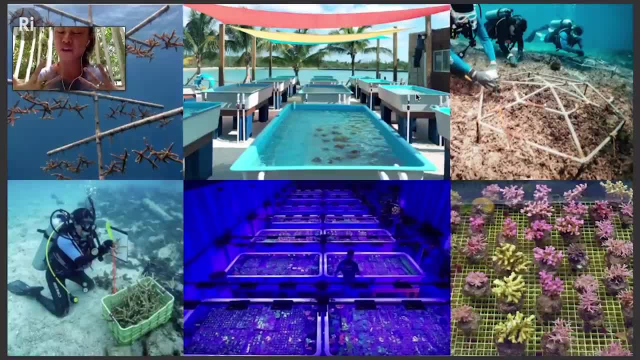 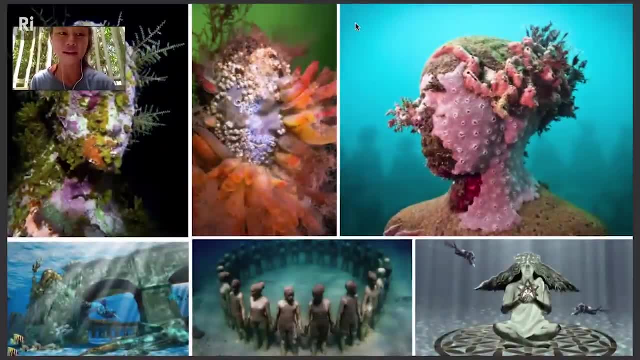 and you bring them into the water, in the ocean, and they actually will, over time, fuse together to create huge colonies. So the scientific advancements are incredible And as artists we were amazed and mind-blown by the other people around the world building sculptures. 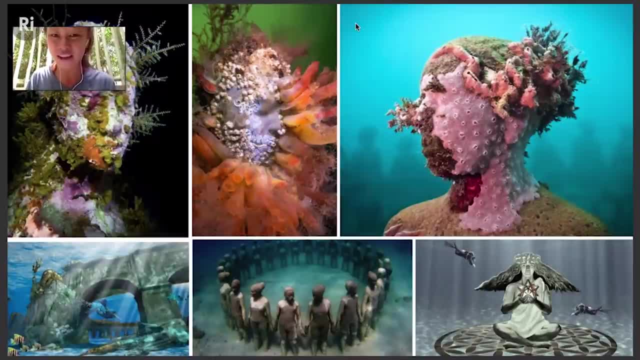 deployed into the ocean. A lot of this work is Jason DeCairos-Taylor and other designs that have been made of how can we build structures underwater that can be inspiring. bring people to the sea, grow coral on them, become new habitats. 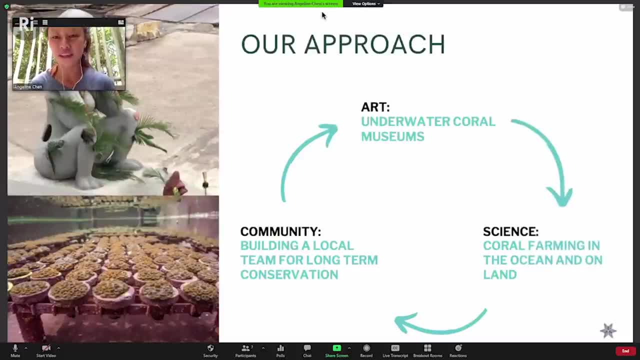 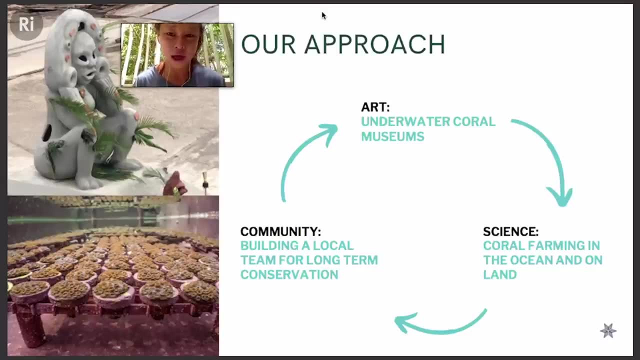 And so we designed Global Coral-Lition, using this approach of building underwater coral museums in local communities, with local people on islands where reefs are at risk, And we pair them with restoration projects, with coral farming on land and in the sea, And then we work closely with the local community to learn these techniques. 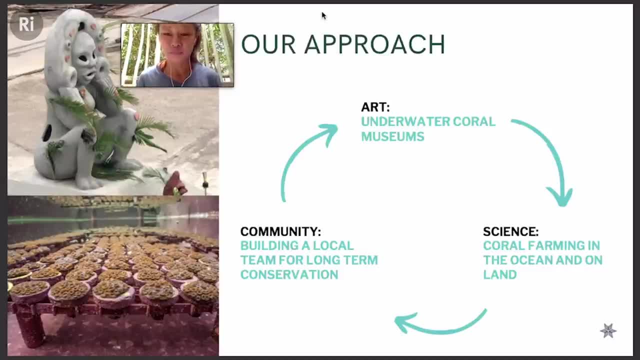 and then we work closely with the local community to learn these techniques. and then we work closely with the local community to learn these techniques and build their own project and economy around coral restoration in their area. and build their own project and economy around coral restoration in their area. 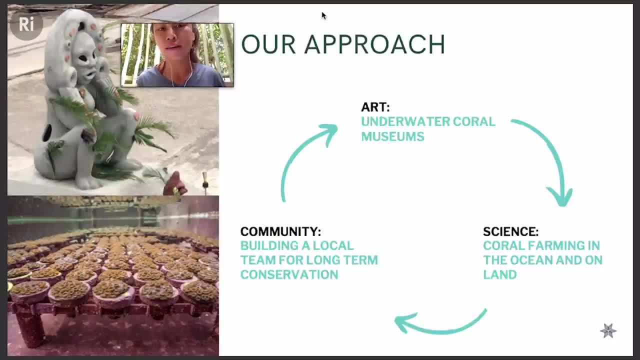 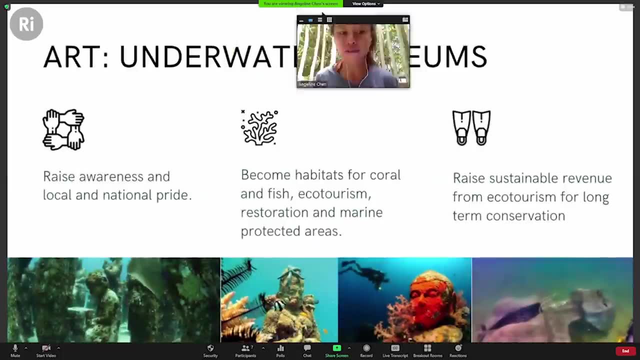 One of the other big keys is: how do you reduce the main causes of degradation in the region? One of the other big keys is how do you reduce the main causes of degradation in the region. So the art has been really beautiful because it raises awareness, local pride. 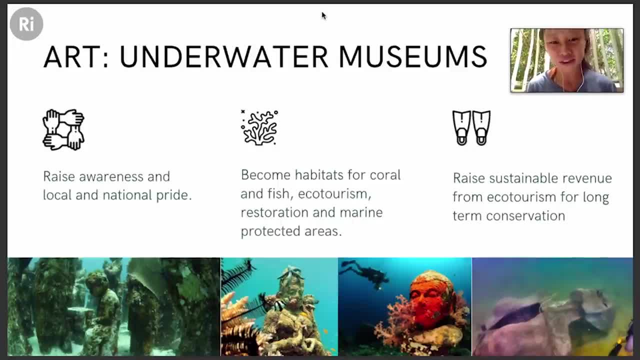 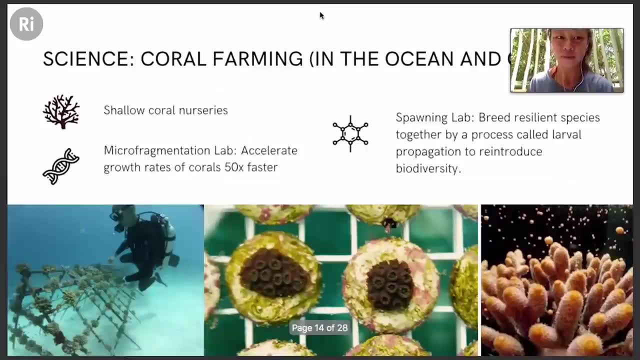 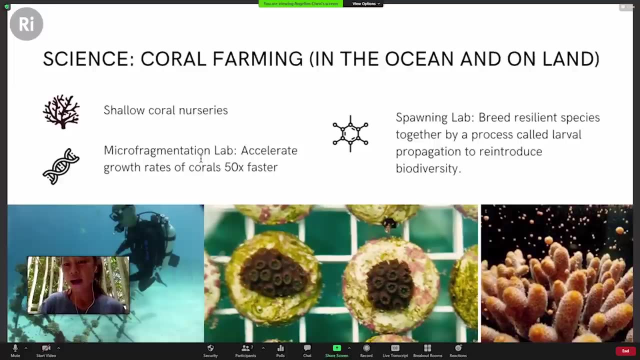 becomes both a marine protected area, eco-tourism site and a restoration site and can be sustainable revenue for the future. With the science, I was sharing a bit about micro-fermentation, which is a really exciting method. With the spawning of corals, scientists were actually bringing these larvae together. 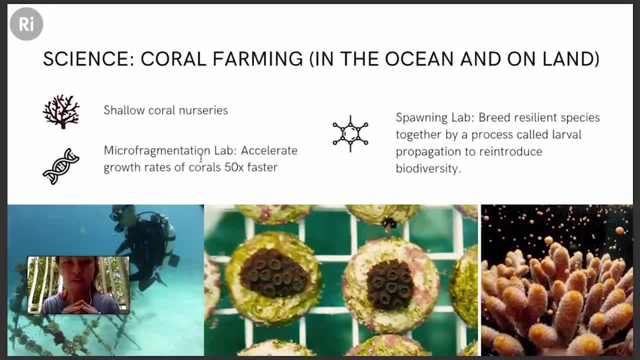 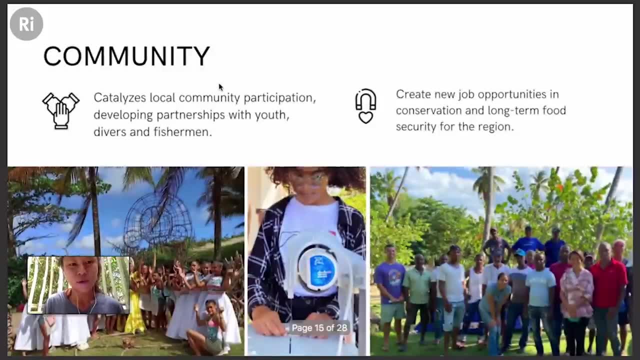 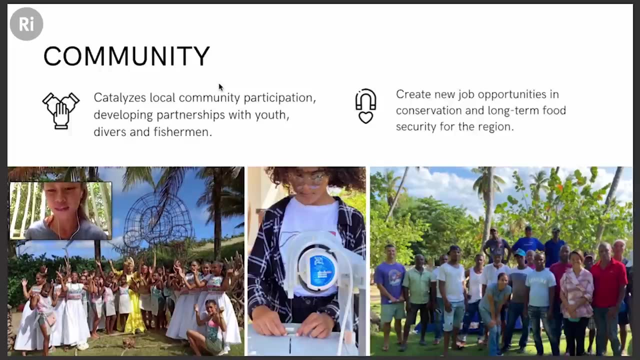 and breeding them together on land and getting over 90% success rate of reproduction. So that's also really exciting. And with community, it's all about bringing people, engaging them, making them connect with these animals, connect with the project and to fall in love with it as well, because you do protect what you love. 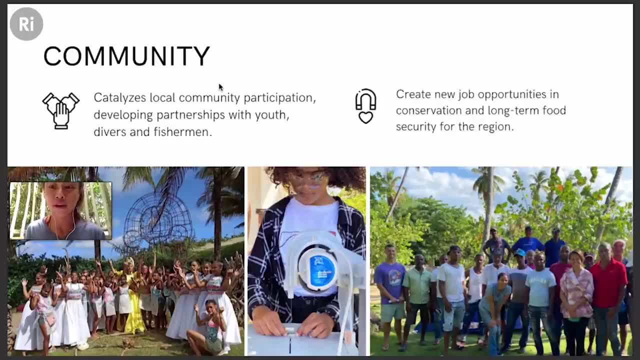 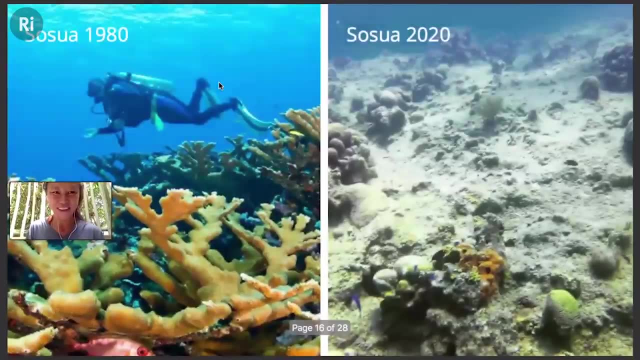 And when we can design projects in a way that creates new opportunities, new jobs, long-term food security for the region. it's good for everyone And just being able to help people see how we can organize in these ways is really exciting. So here's the SUA where we are right now. just how much it's changed. 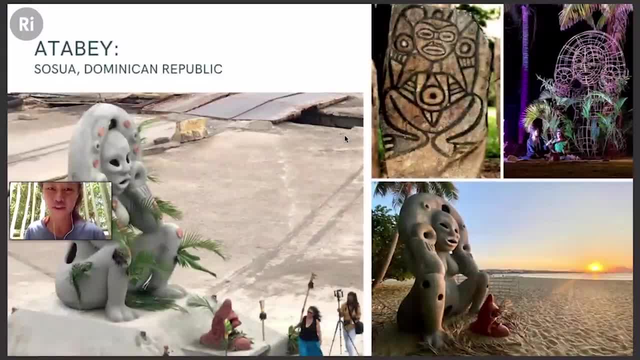 And we've launched our first project here. We work a lot with indigenous wisdom. This is Atebe, the mother earth spirit of the Arawak Taino people, the indigenous people of the Caribbean, And we built this sculpture to deploy and launch a restoration project here. 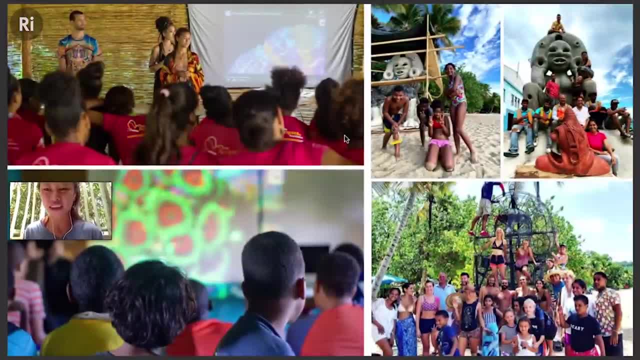 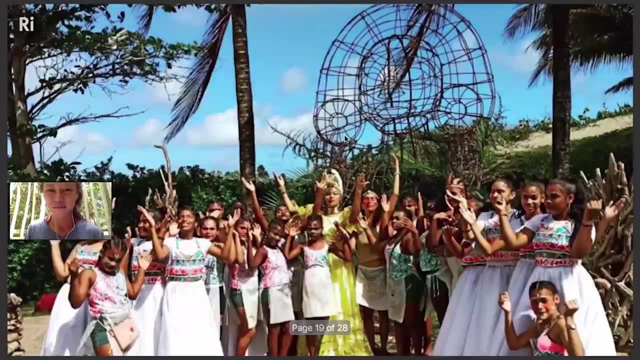 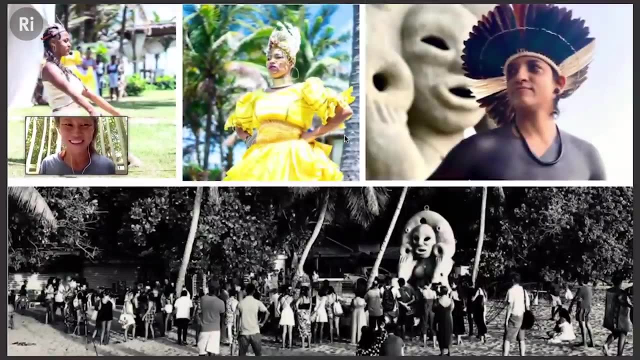 Just engaging all the kids, sharing the project We build in a public place so everyone can see it and feel it and connect with it. I think I'm going over time so I'm just going to rush through these photos. Working with you know, everyone has a part to play. 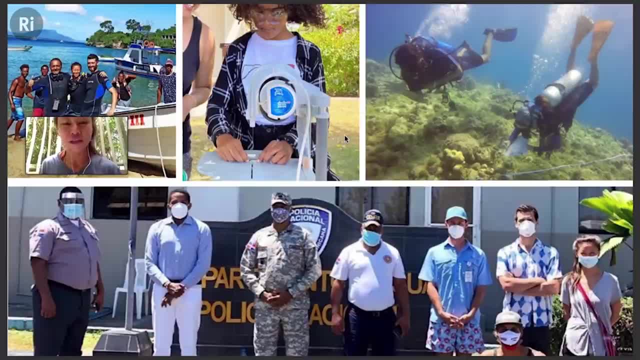 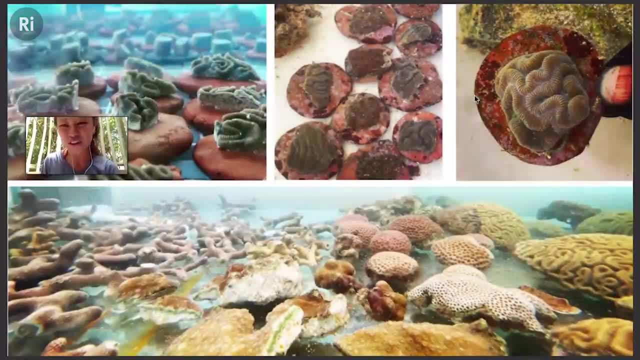 As you guys said, the officials, the dive community, the youth, the fishermen. We did a small micro-fragmenting project and found huge success with corals growing, And now we're on our second sculpture here, inspired by Ana Kaona. 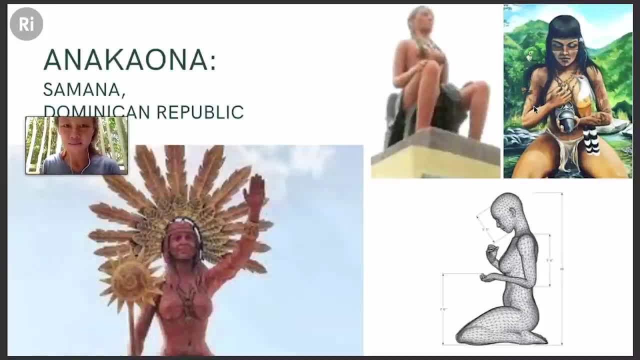 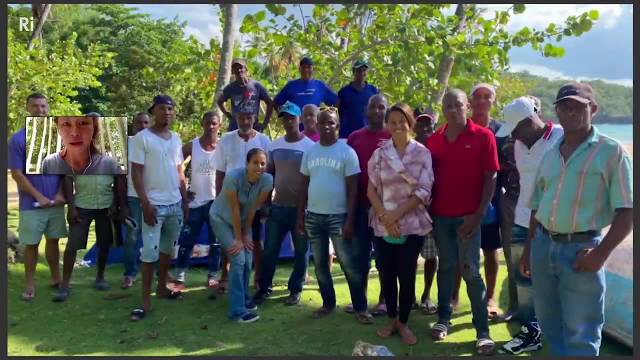 who was an indigenous chief on the island when the Spanish arrived, And this is launching our second project here in the DR. It'll be mainly working with the fishermen of this small town who their livelihood has been really threatened by the collapse of the ecosystem here. 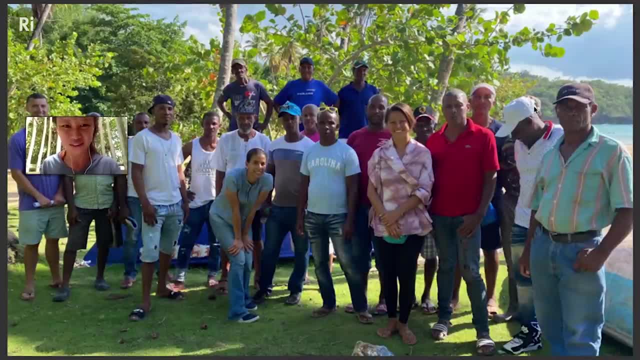 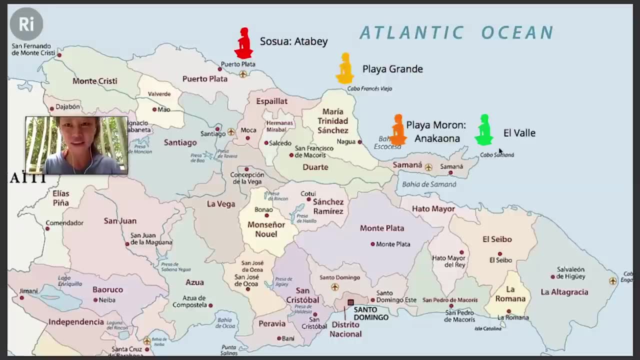 And so we're helping them transition into coral farmers, which is really super exciting, And our hope now is to reach four different areas on the North Coast here And we hope, you know, one day to target the most endangered coral reef ecosystems. 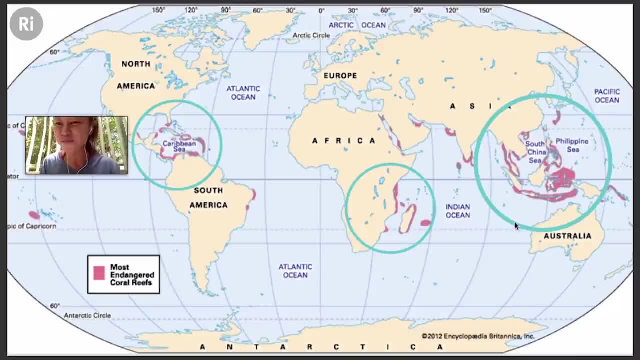 collaborate with other restoration groups- hopefully meet you in India one day, And you know it is so important to collaborate, to take a holistic approach, to work with kids, to help people be more educated about what's happening and to feel connected to it and realize that everyone can make a difference. 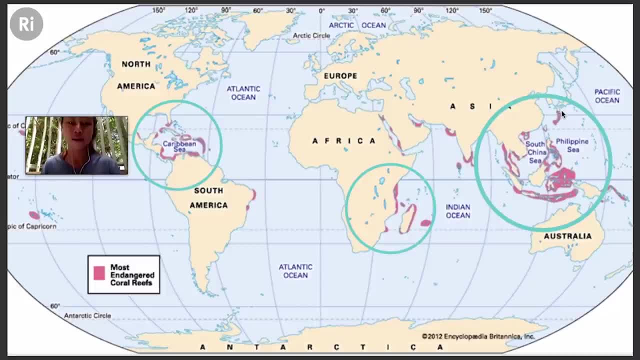 and has a part to play, no matter what your background is. I learned all of this. I learned all of this in the last three years just because the reefs and realized this was happening. And I have no scientific background personally, but I'm so grateful when I do meet scientists. 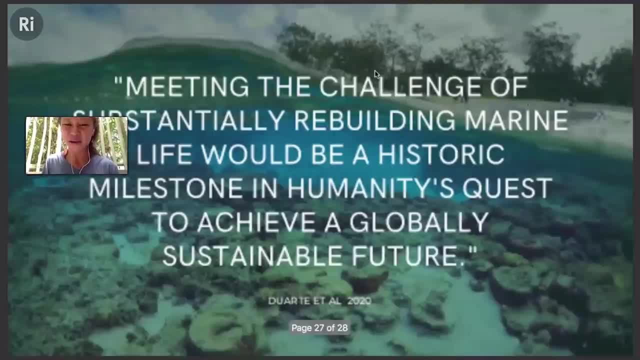 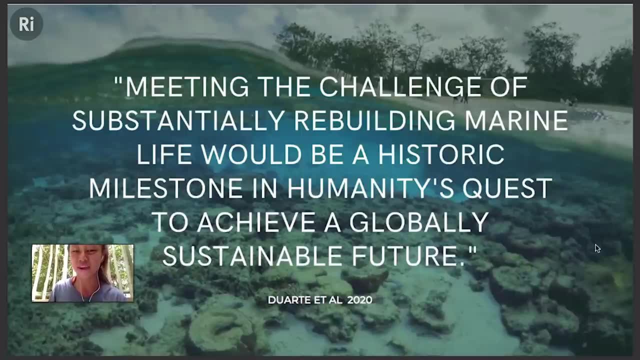 and we get to collaborate and learn from each other- And this is just a quote I really love, which is: meeting the challenge of substantially rebuilding marine life would be a historic milestone in humanity's quest to achieve a globally sustainable future. Thank you so much. 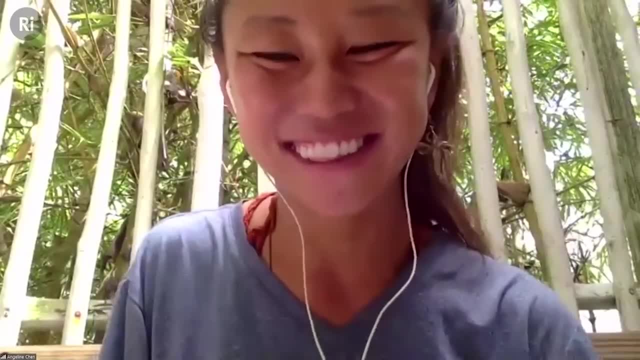 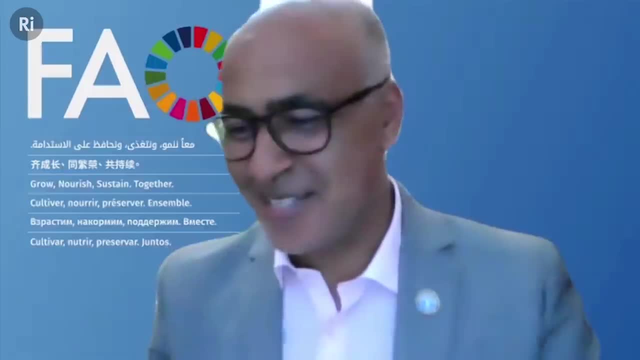 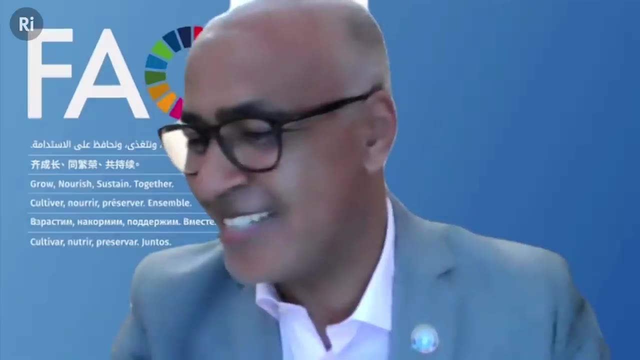 Thank you. Thank you very much, Angeline. It's very nice to hear the perspective of an artist And I liked your connection between the art community and science, So thank you very much for illustrating that really nicely. Again, you know the key points I picked up. 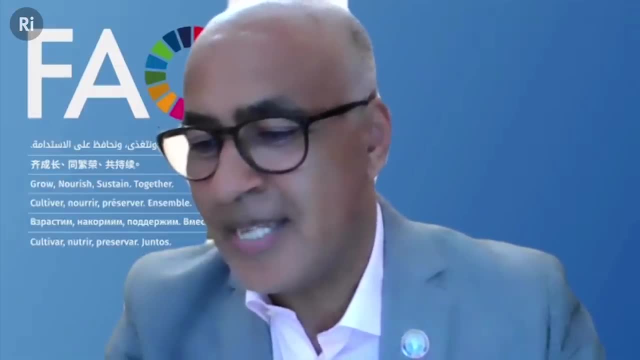 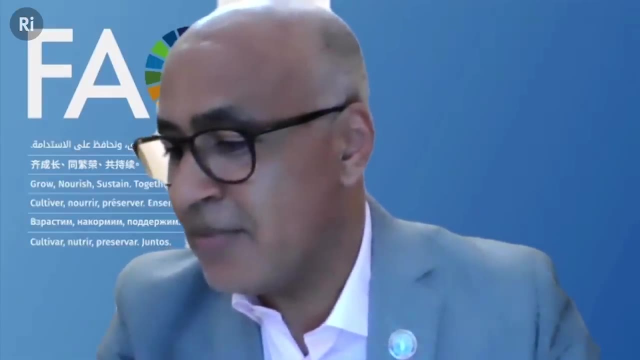 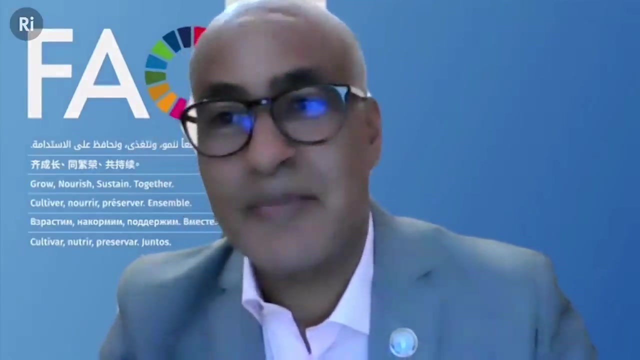 you know how the coral reef is economically, ecologically and socially important And it's shocking that we lost 50% of our coral reef in the last 30 years And we're going to lose about 90% by 2050. 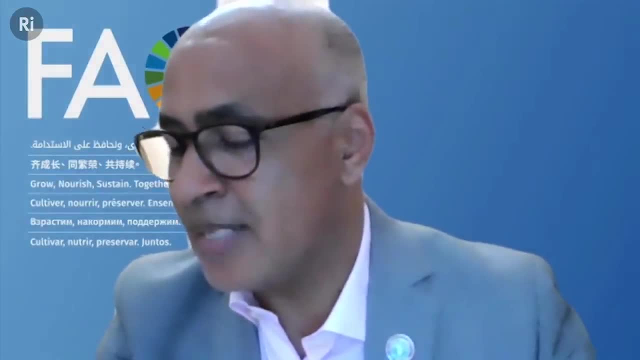 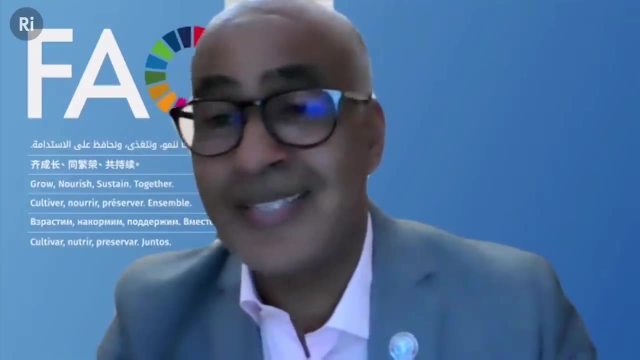 if we continue at this rate. And also you highlighted the fact that 1 billion people depend on coral reef for their food and livelihood. So you can see really the connection and the vulnerability of, you know, people living around the world that depend on nature and natural resources.